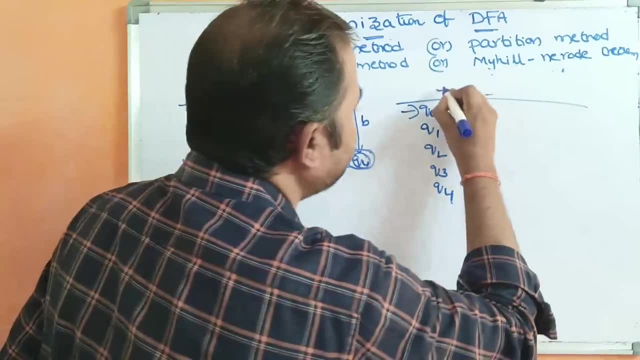 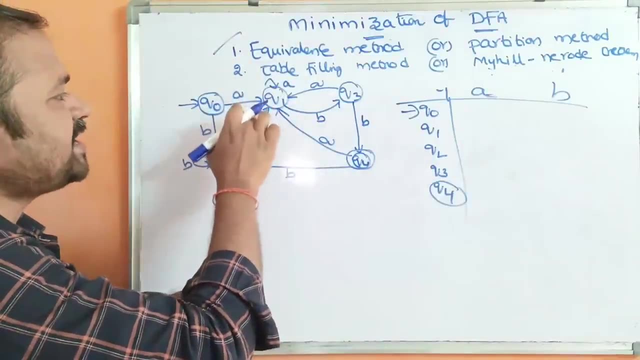 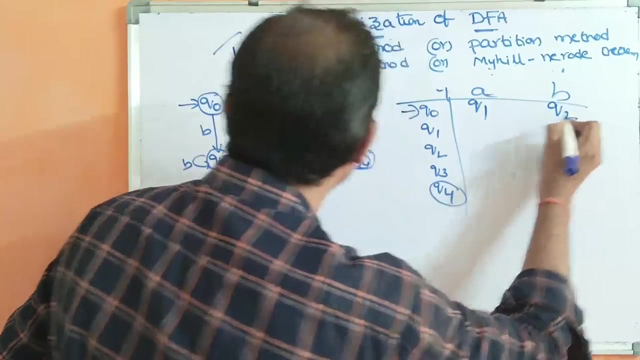 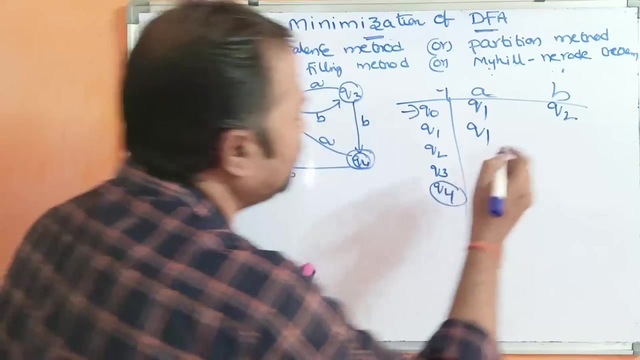 Here we are constructing the transition table. Input symbols are a and b. Here q0 is the initial state, q4 is the final state. q0 on a goes to q1.. q0 on b goes to q2.. Next q2 on a goes to q1.. q2 on b goes to q2 only. Next q3 on a goes to q1.. q3 on b goes to q4. 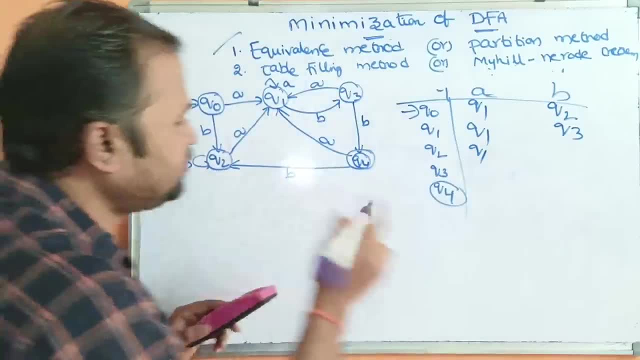 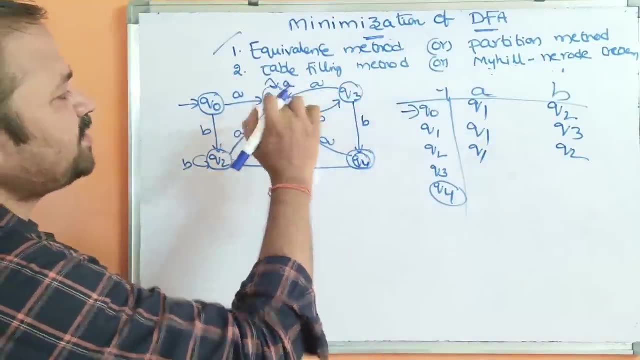 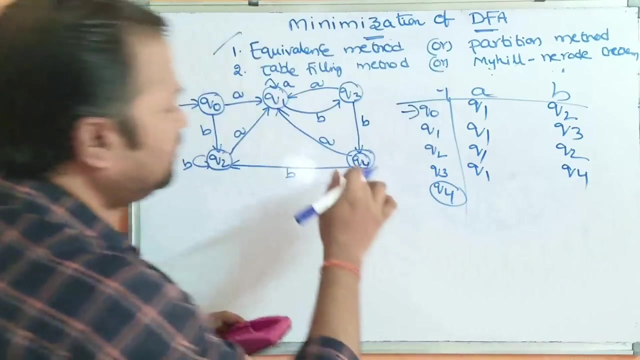 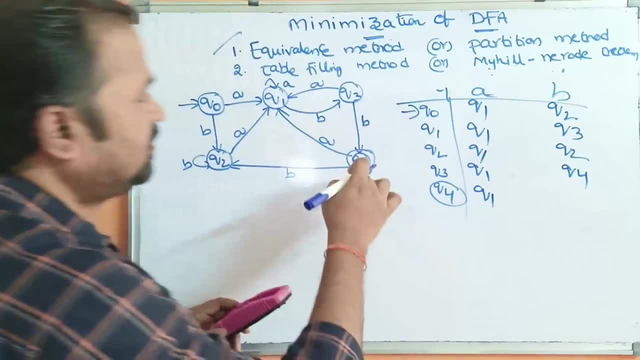 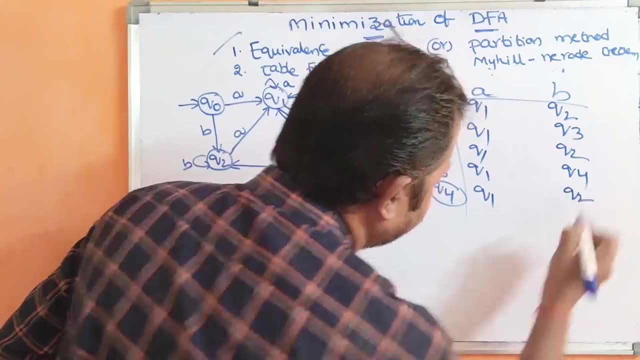 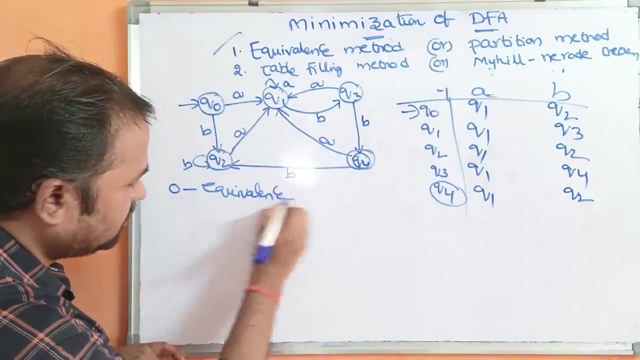 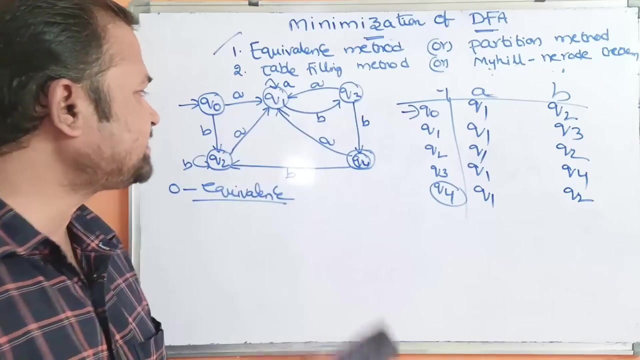 Next q4 on a goes to q1.. Next q4 on b, q4 on b goes to q2.. So first here we have to calculate zero equivalence. So in this diagram the final state is q4, whereas the non-final states are q0, q1, q2, q3.. 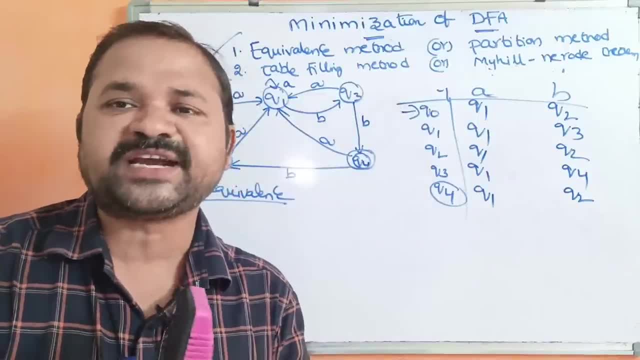 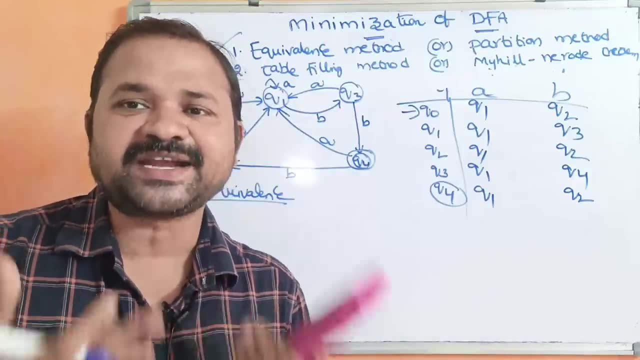 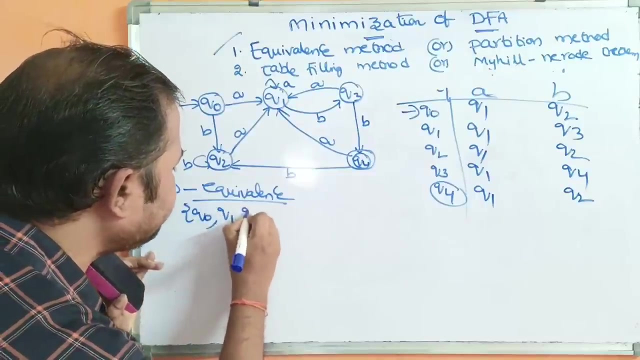 So zero equivalence mainly contains two set of states. The first, first set represents set of non-final states. second set represents set of final states, so q0, so what are the non-final states? q0,, q1, q2, q3. 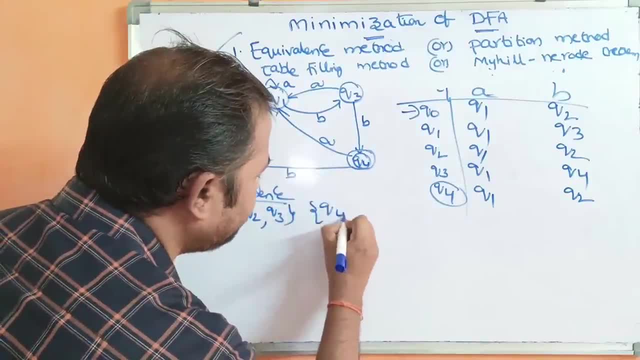 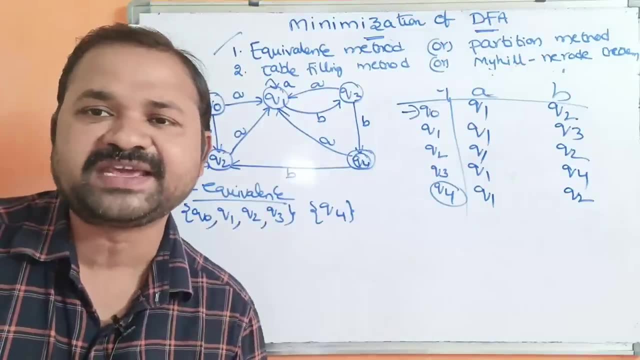 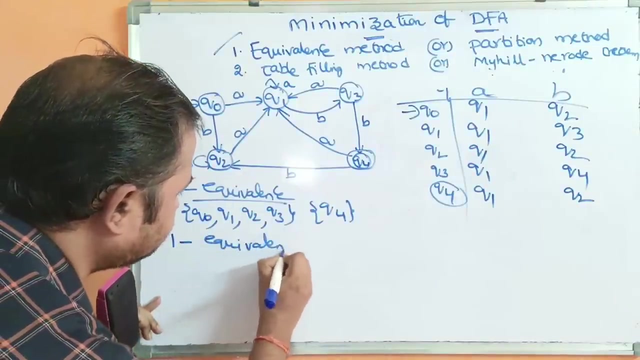 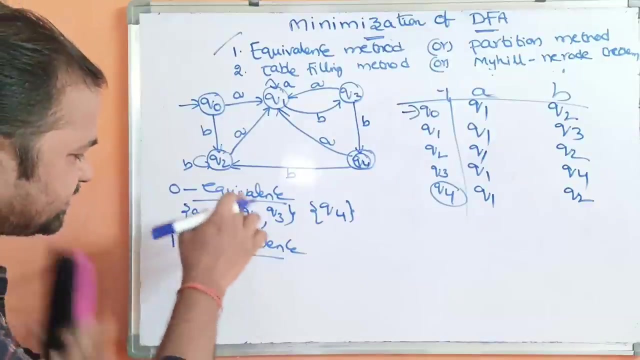 whereas the final state is q4.. In this diagram, we have only one final state, that is, q4. only Now we have to calculate one equivalence based on the zero equivalence. let us calculate one equivalence, one equivalence based on the zero equivalence. so, for that purpose, what we have to do is: here the set contains four states, so we have to check. 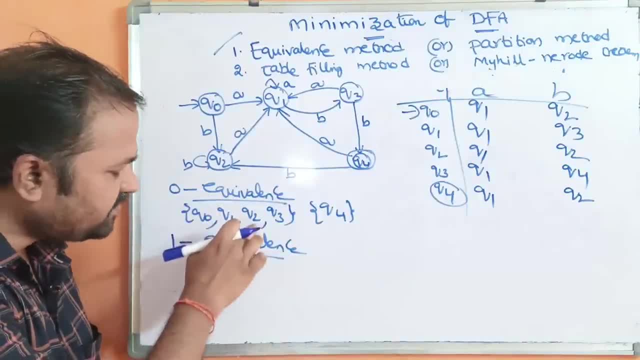 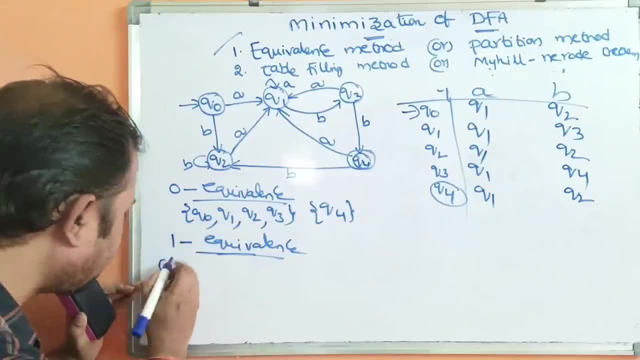 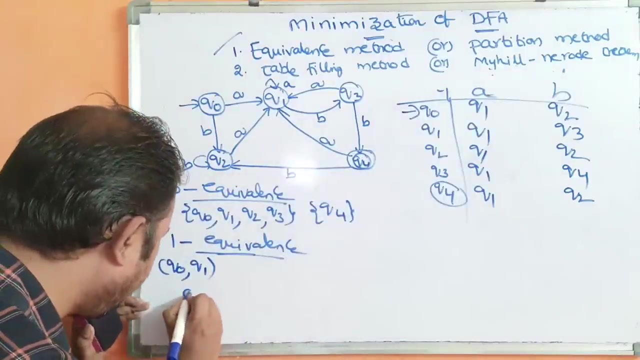 we have to compare q naught with q1, q naught with q2, q naught with q3, whether they are equal or not. okay, let us take the pair q naught and q1 and apply the inputs a and b. okay, so delta of q naught. 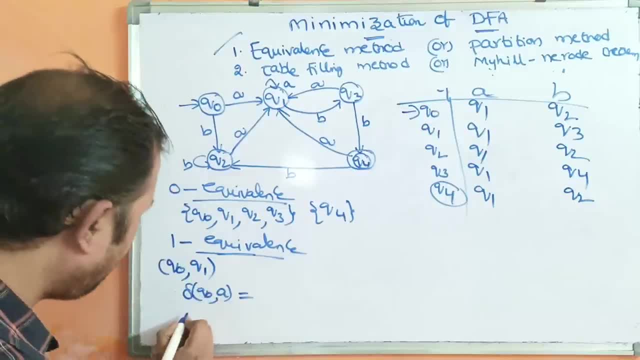 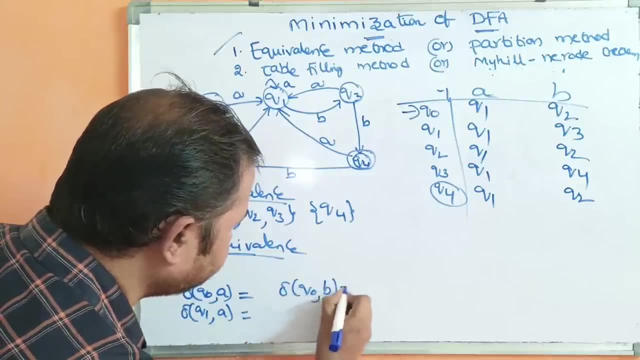 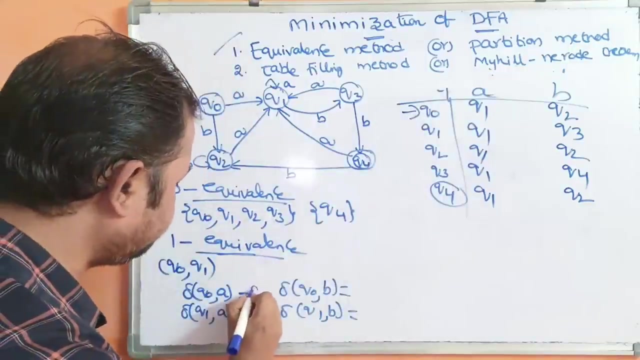 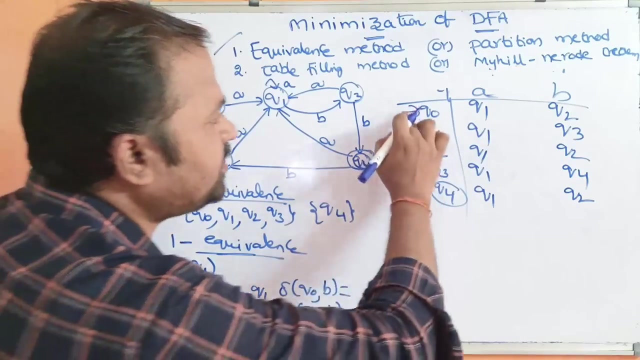 comma a is equal to delta of q naught comma a. that is the first pair next to q1 comma a, next q naught comma b, next to q1 comma b. we have to calculate all these pairs: q naught comma a means q1. next q1 comma a means q1. next to q naught comma b means q2. q1 comma b means q3. 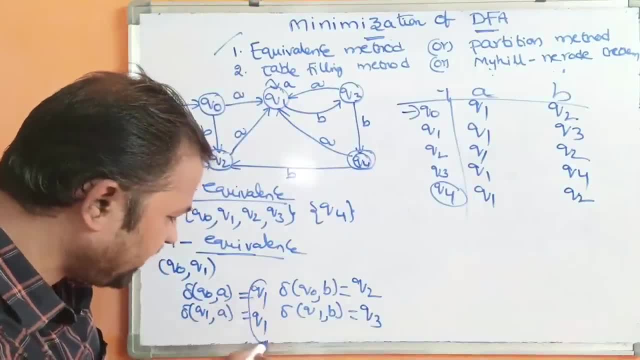 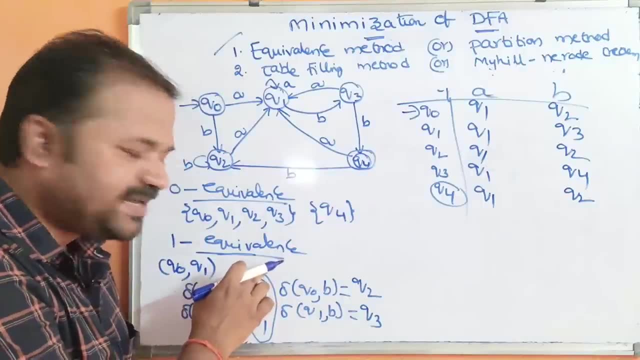 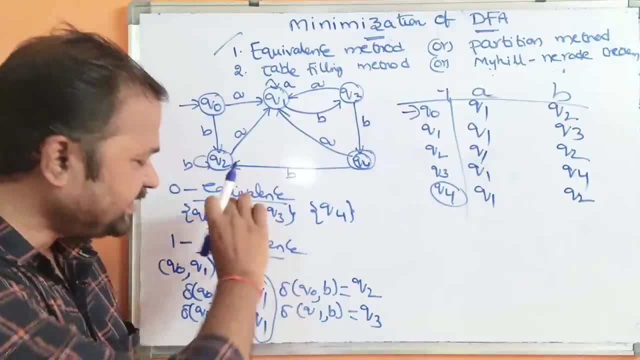 q1, q1. q1 is present in the q1. q1. q1 is present in the same set, so we can say that this is present in same set. so we can say that this is present in same set. so we can say that this is present in the same set. 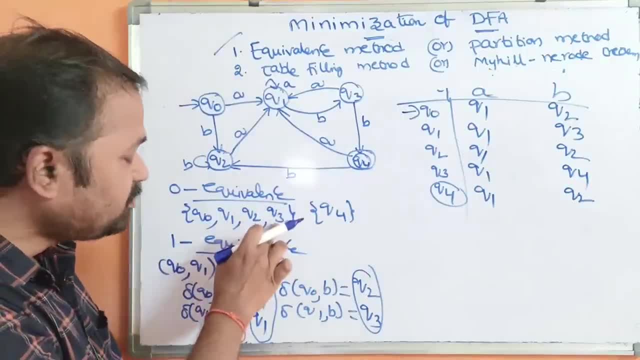 the same set. the same set. next here we got q2, q3. q2 on q3 is present. next here we got q2, q3. q2 on q3 is present. next here we got q2, q3. q2 on q3 is present in the same set. 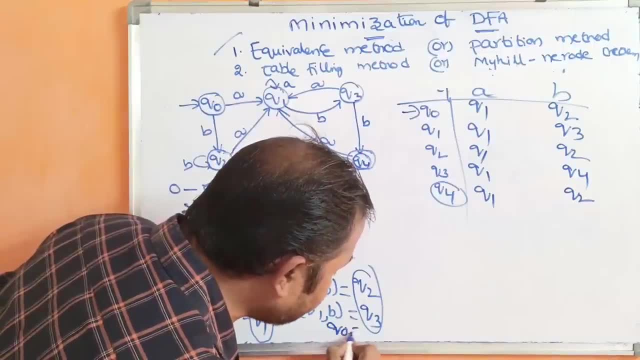 in the same set. in the same set. so we can say that q naught is equals to q1. so we can say that q naught is equals to q1. why? because here these states? why because here these states? why because here these states q1. q1 means only one state, so that is. 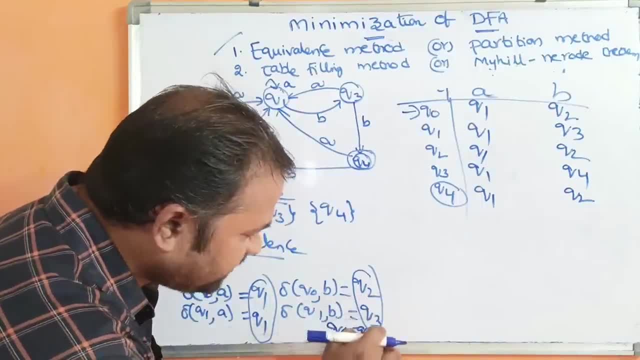 q1. q1 means only one state, so that is q1. q1 means only one state, so that is present in the same set, present in the same set, present in the same set. so likewise here, if we here, we got the. so likewise here, if we here, we got the. 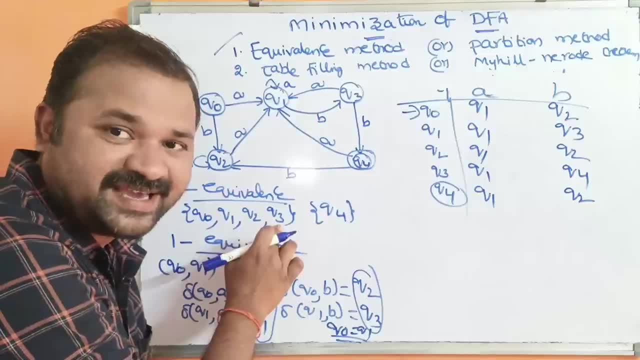 so likewise here. if we here we got the result as q naught q3. q naught q3 is result as q naught q3. q naught q3 is result as q naught q3. q naught q3 is present in the same set. 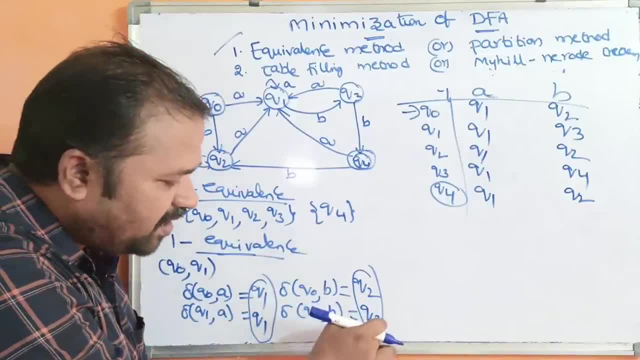 present in the same set. present in the same set. but suppose if we got here q4. but suppose if we got here q4. but suppose if we got here q4, let here we got q4. q2 is present in one. let here we got here q4. q2 is present in one. 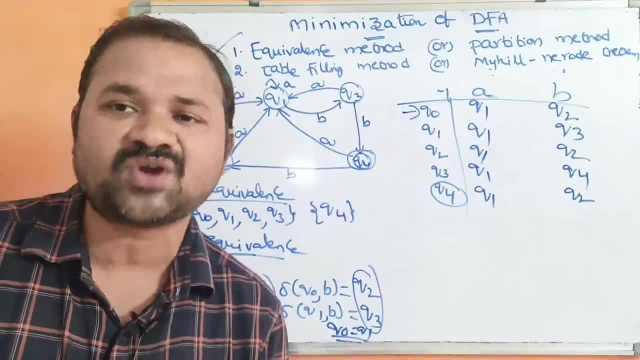 let here we got here q4. q2 is present in one set, q4 is present in another set set. q4 is present in another set set, q4 is present in another set, then we can say that q naught is not. then we can say that q naught is not. 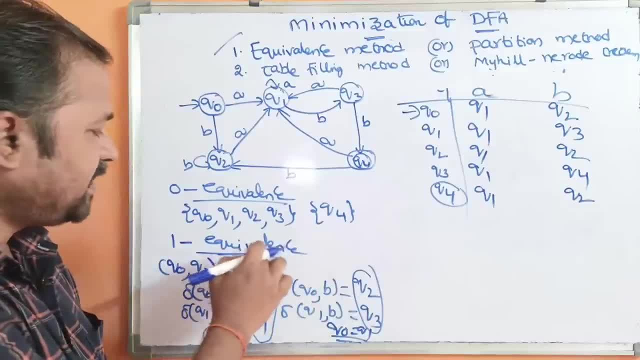 then we can say that q naught is not equal to q1, equal to q1, equal to q1. but here we got q2 and q3 they are. but here we got q2 and q3 they are. but here we got q2 and q3. they are present in the same set. 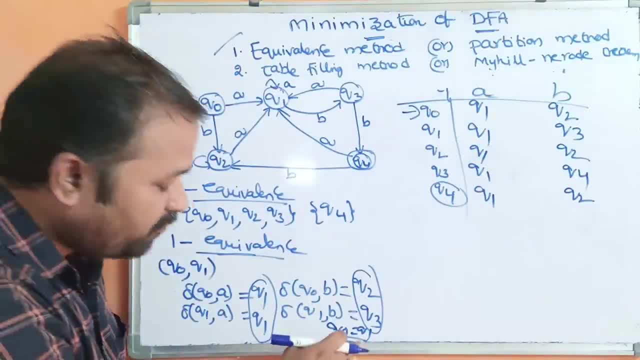 present in the same set. present in the same set. so we can say that q naught is equal to. so we can say that q naught is equal to. so we can say that q naught is equal to the q1, the q1, the q1. now we have to compare q naught with q2. 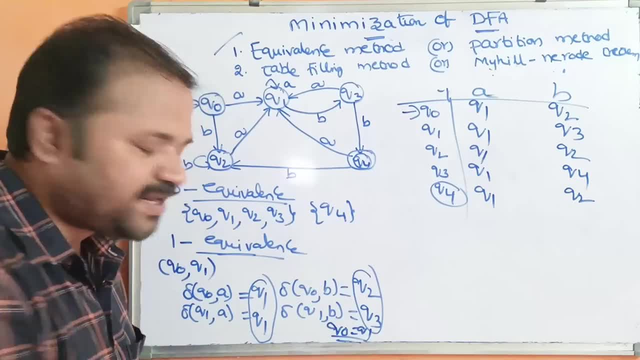 now we have to compare q naught with q2, or we can compare q1 with q2, or we can compare q1 with q2, or we can compare q1 with q2. why? because q naught and q1 are equal. why? because q naught and q1 are equal. 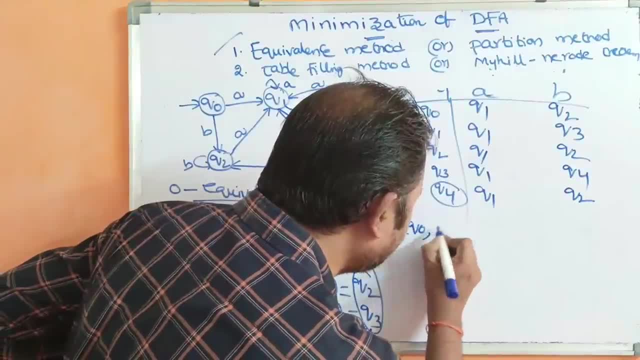 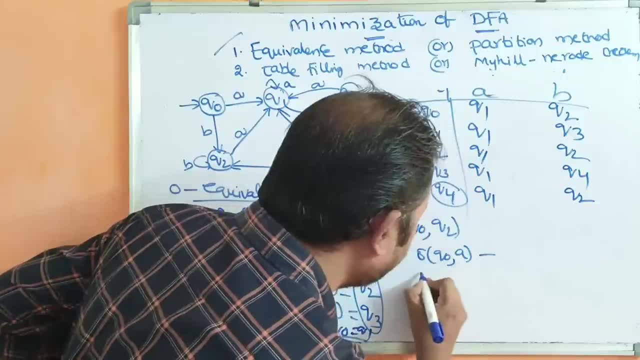 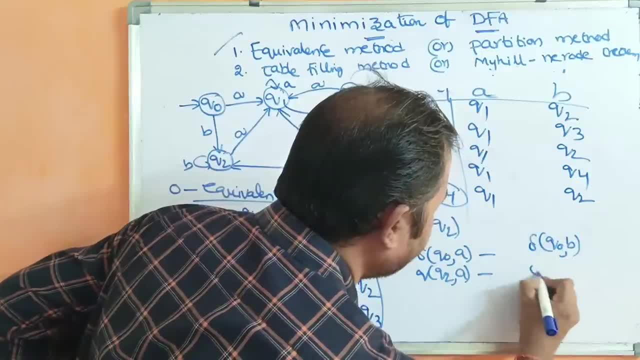 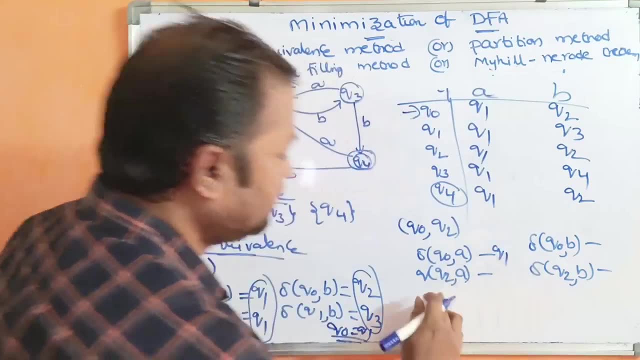 next to delta of q2 comma a. next to delta of. next to delta of q2 comma b. next to delta of q2 comma b. next delta of q2 comma b. So what is q0 comma a: q1.. Next to q2 comma a: q1.. 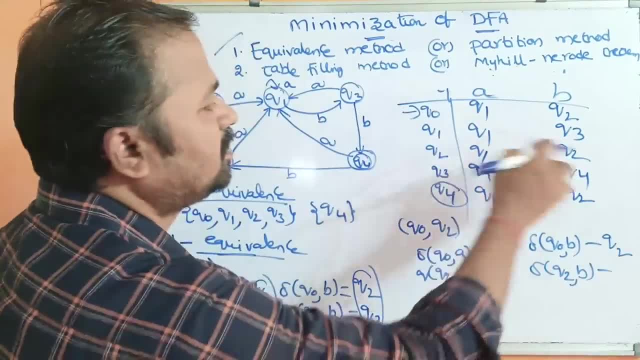 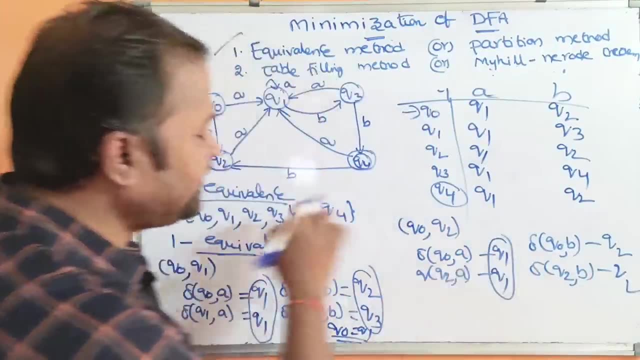 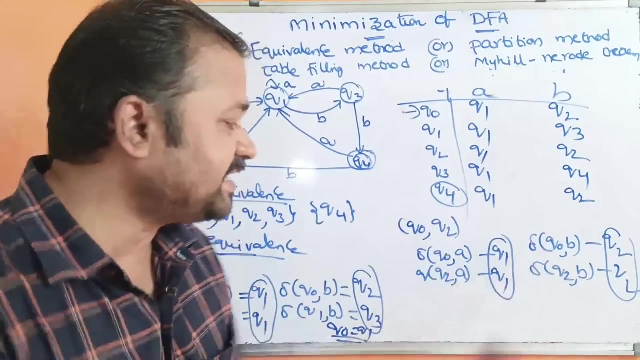 Next to q0, comma b: q2.. q2, comma b: q2.. Here we have q1.. Here we got q1.. q1 is present in one set only. Here also we got q2.. So q2 is present in one set only, So we can say that q0 equals. 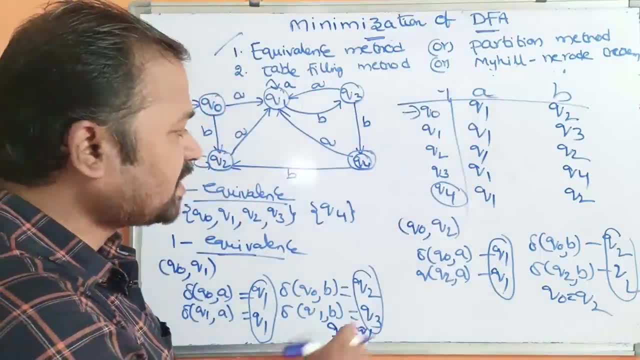 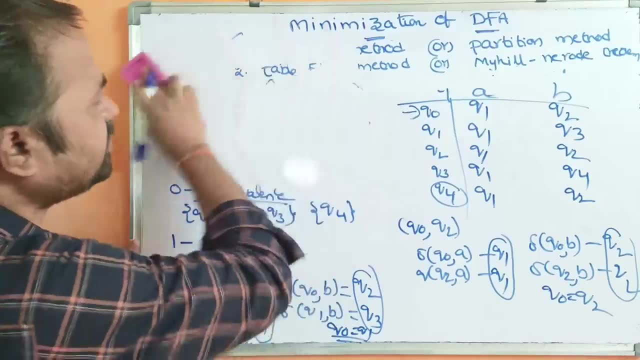 to q2.. So q0 equals to q1, q0 equals to q2.. Now we have to calculate. now we have to compare q0 and q3.. So for space constraints I am erasing this portion. So now let us compare. 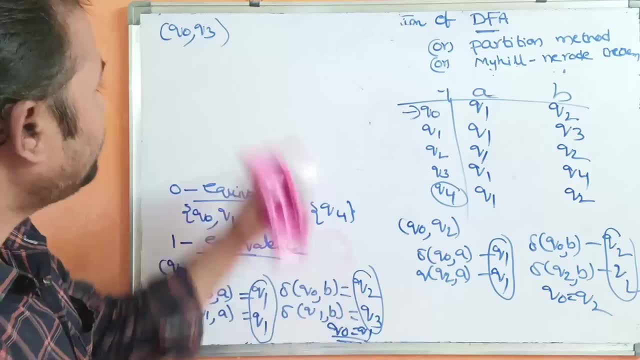 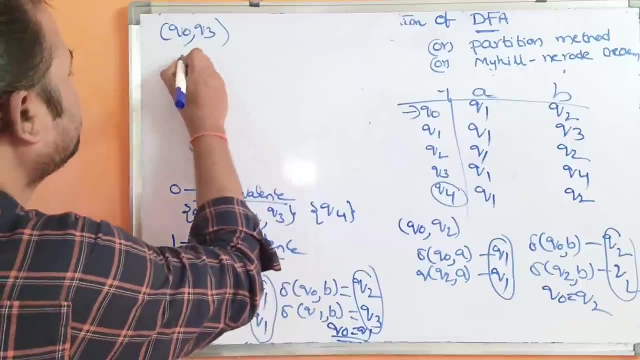 q0 with q3, or we can compare q1 with q3 or q2 with q3.. Why? Because q0, q1 and q2 are equal, only ok. So let us calculate delta of q0 comma a. Next to q1 comma b: q1.. Next to q2 comma b: q2.. Next to q1 comma b: q2.. Next to q1 comma b. 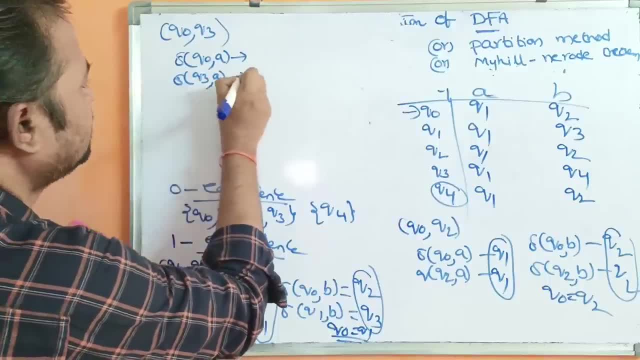 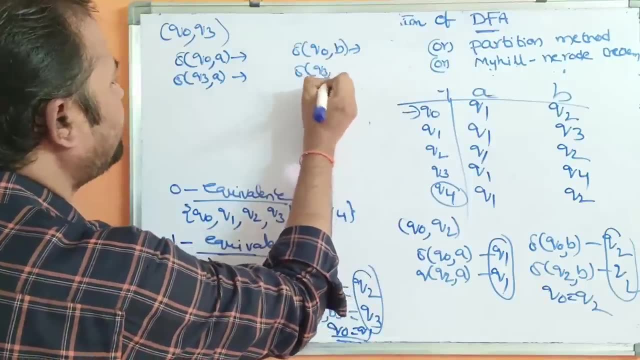 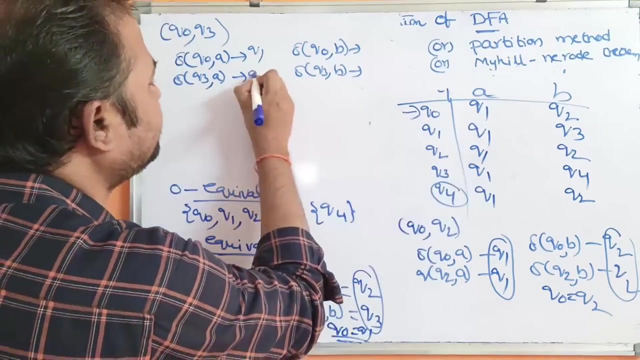 q2.. Next delta of q3 comma a. Next delta of q0 comma b. Next delta of q3 comma b. So what is q0 comma a, q1.. q3 comma a is also q1.. Next to q0 comma b means q2.. Next here. 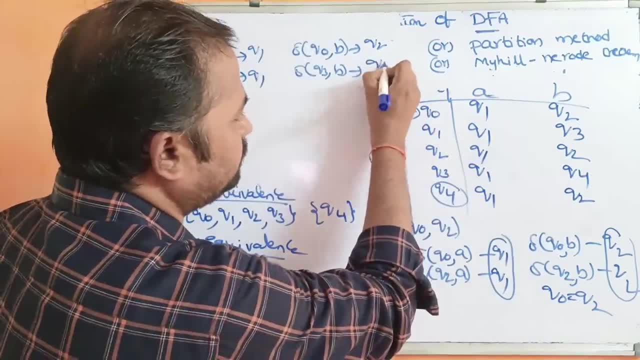 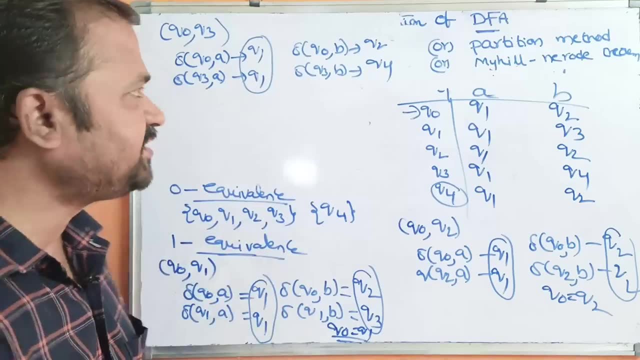 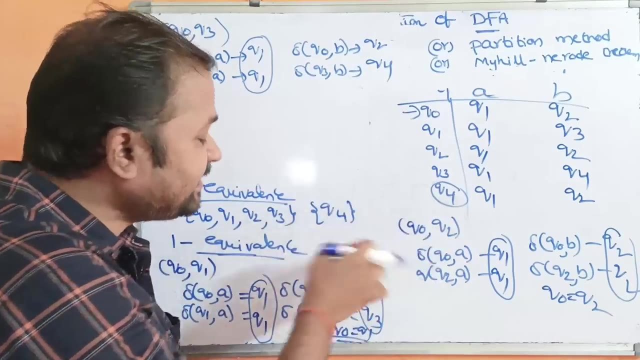 the state is q3. q3, comma b means q4. q4. q1, q1. So there is no problem. So it will be present in only one set only. But if we observe, q2, q4. q2 is present in one set, whereas q4 is present in another set. q2 is present in one. 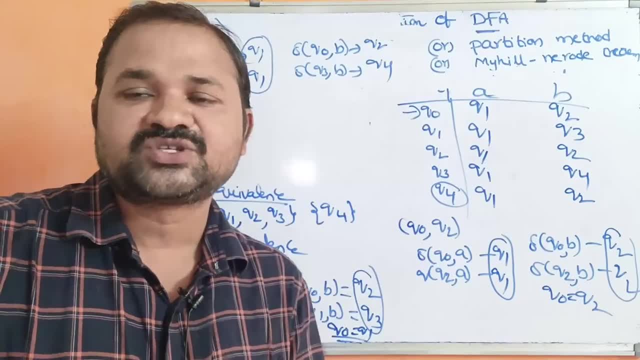 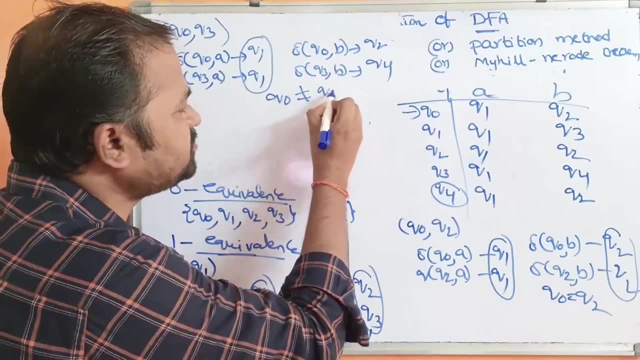 set, whereas q4 is present in another set. So we can say that q0 and q3 are not equal. So we can say that q0 is not equal to q3.. So here q0 equal to q1, q0 is equal to q2.. 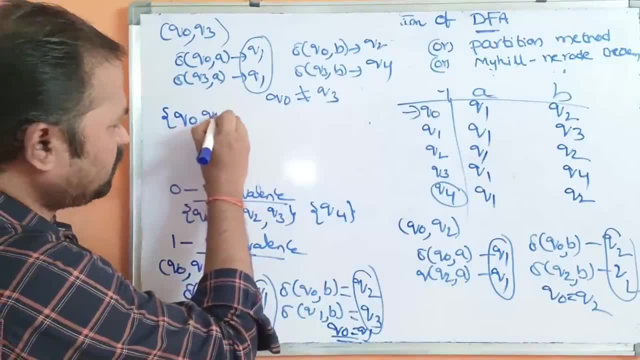 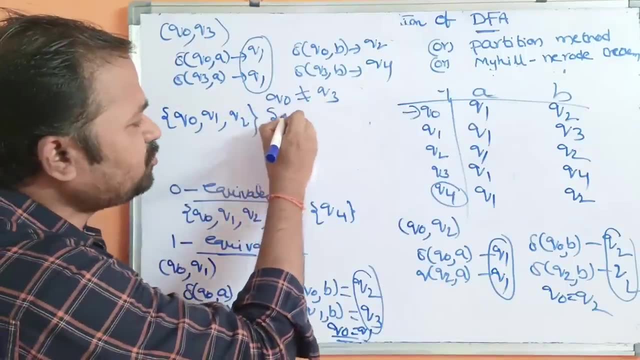 Now one equivalence means q0, q1, q2.. Why? Because these three states are equal, But q0 is not equal to q3. So we have to write q3 in another set. Next, here we have one more. 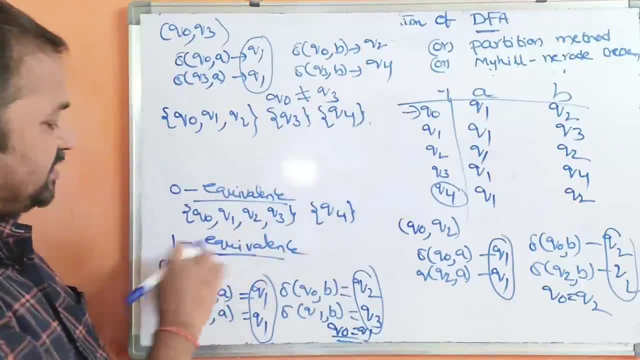 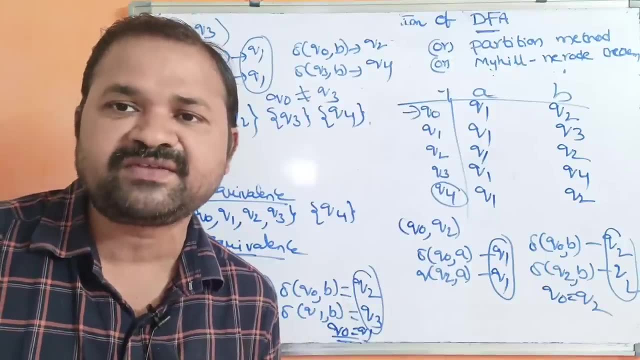 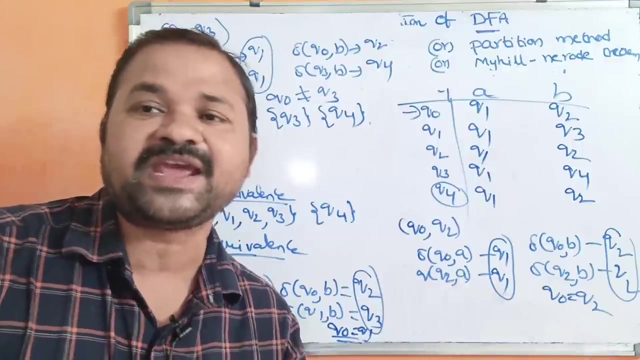 set called q4. So let us write that set here. So this is one equivalence. So zero equivalence is calculated. Next one equivalence is calculated, Next two equivalence, three equivalence. Likewise we have to calculate until The subsequent equivalences are equal. 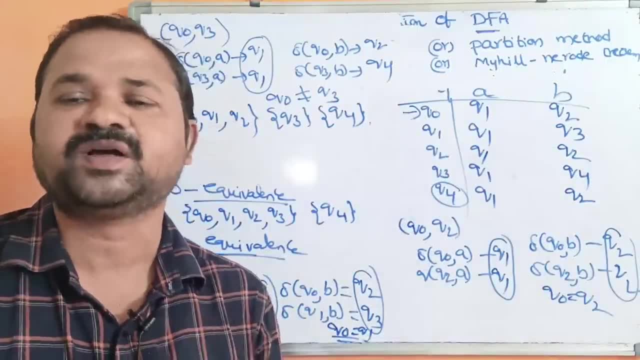 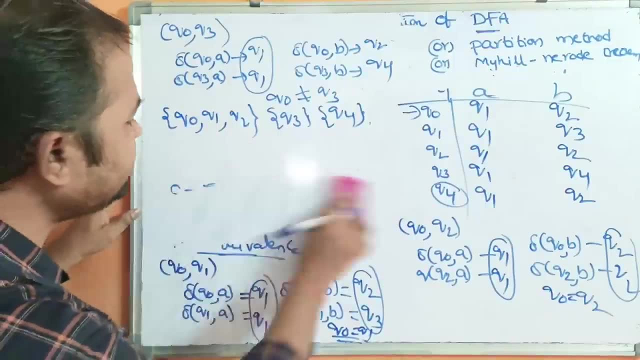 Suppose, if 2 equivalents and 3 equivalents are the same, Then we can quit the process and match the states. So let us see, Let us calculate 2 equivalents. 1 equivalents is over. Now let us calculate 2 equivalents, 2 equivalents. 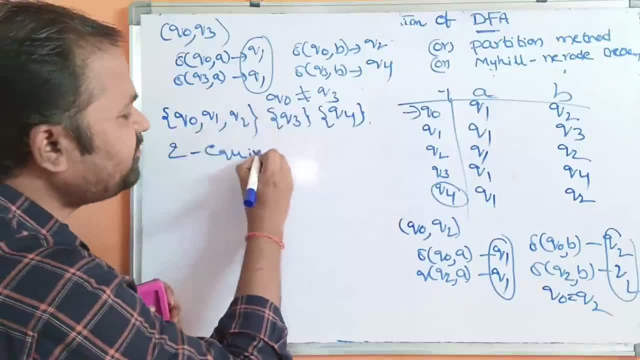 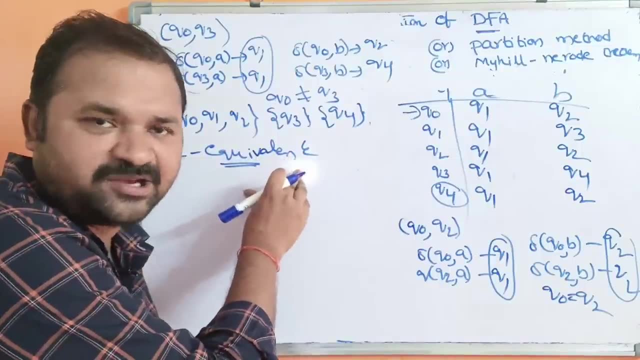 If 2 equivalents, result is also same, Then we can quit the process. Otherwise we have to calculate 3 equivalents. So here 2 equivalents is calculated based upon 1 equivalents. So in 1 equivalents we have q0,, q1, q2.. 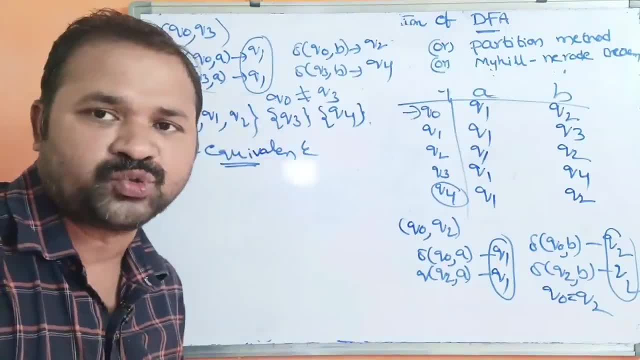 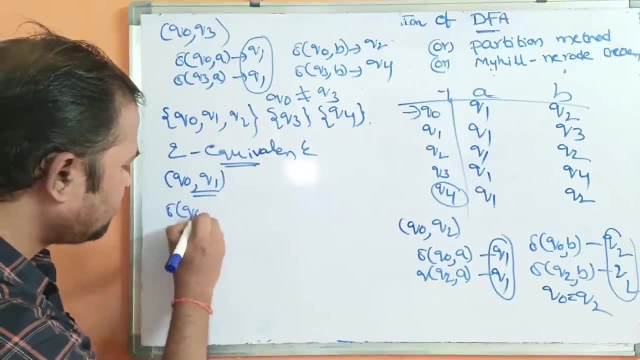 Now we have to compare q0 with q1,, q0 with q2.. Whether they are equal or not. So first to compare q0 with q1.. So delta of q0, a. Next to delta of q1, a. 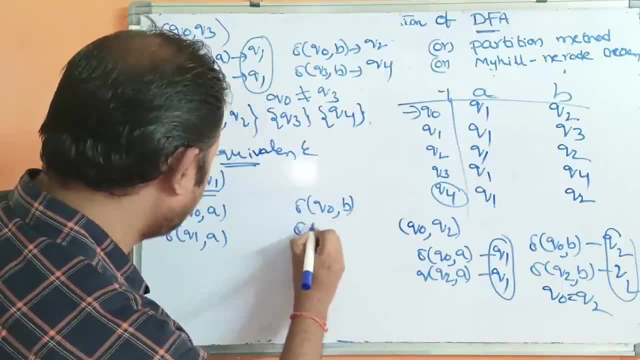 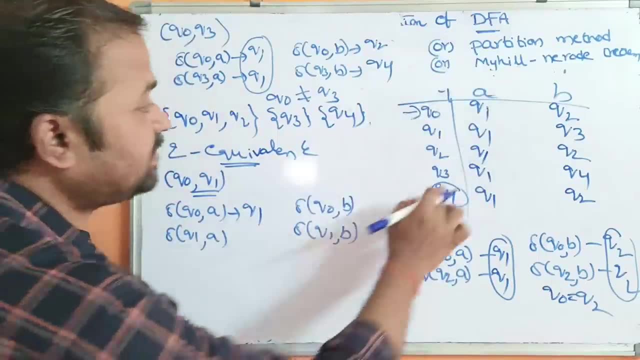 Next to delta of q0, b. Next to delta of q1, a. Next to delta of q1, b. So what is q0 on a? q0 on a means- q1.. q1 on a means- q1.. 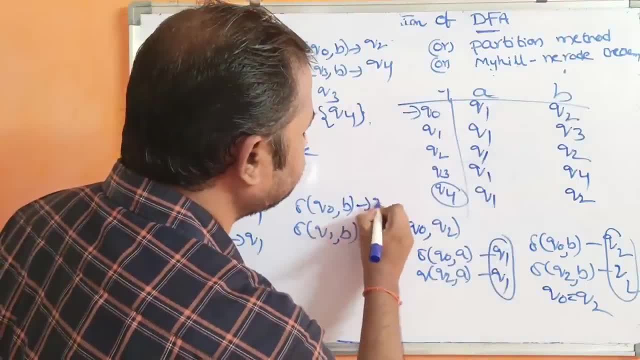 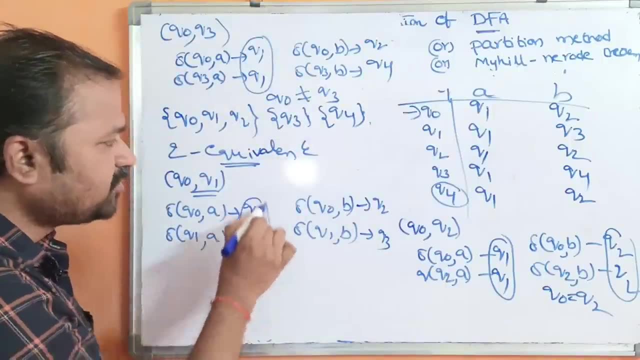 Next to q0 on b means q2.. q1 on b means q3.. Here we have only one state, That is, q1.. q1 is present in only one set, So there is no problem. But if we observe here: 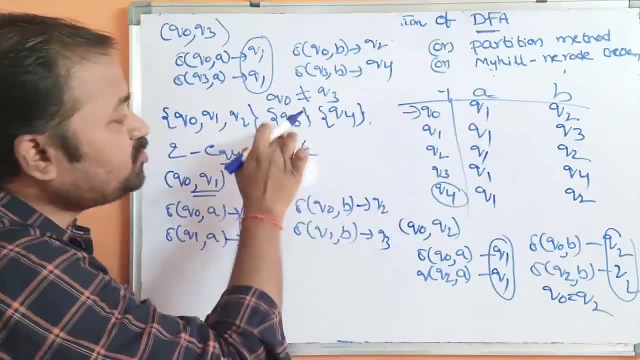 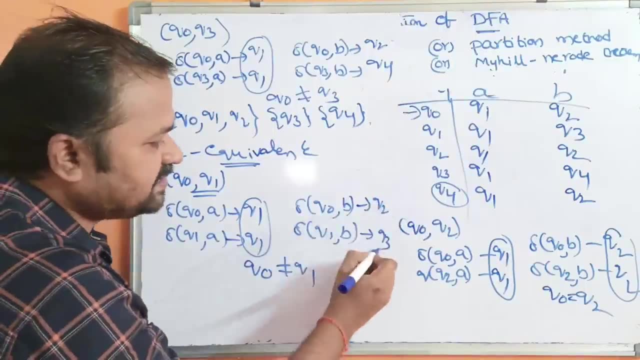 q2 is present in one set, Whereas q3 is present in another set, So we can say that q0 is not equals to q1. Why? Because these two are not equal. q2 is present in one set, Whereas here we got q3. 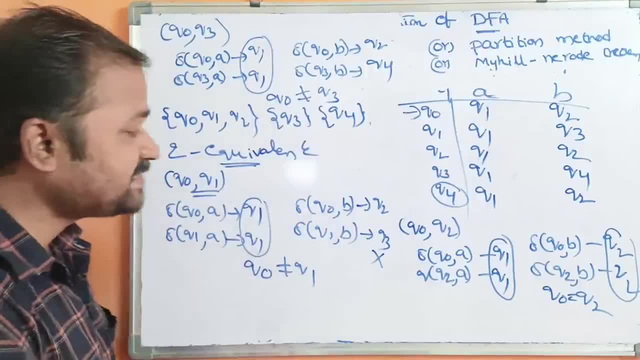 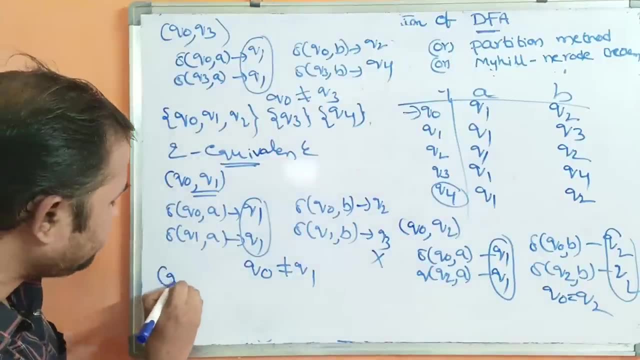 q3 is present in another set, So we can conclude that q0 is not equal to the q1.. Now we have to compare q0 with q2.. Whether q0 and q2 are equal or not, So compare q0 and q2.. 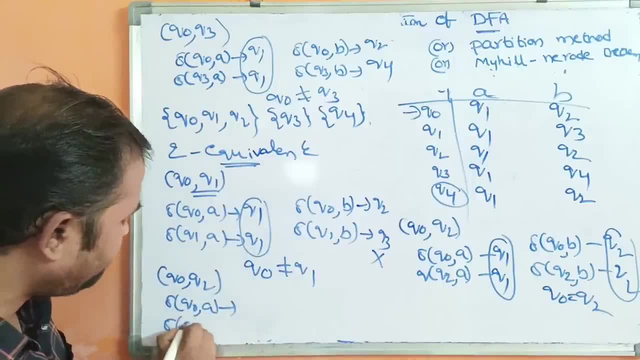 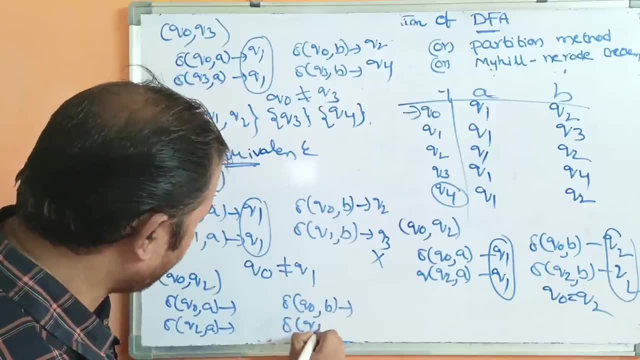 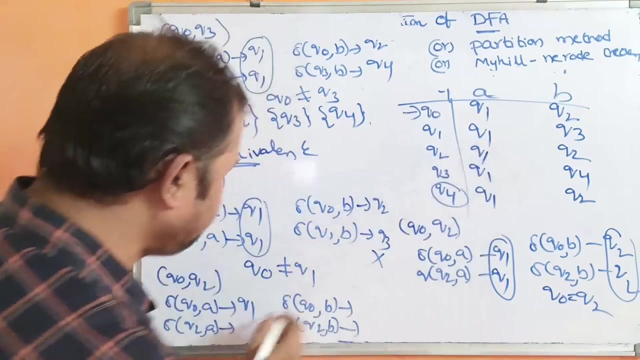 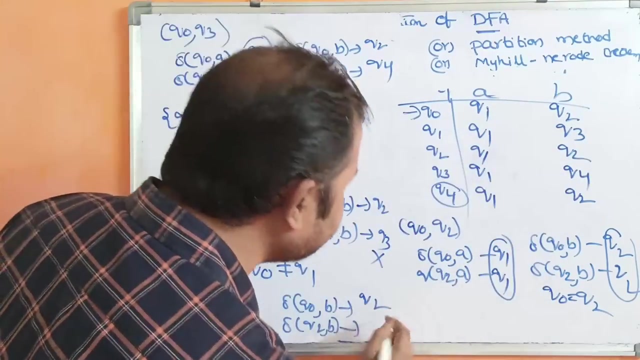 So delta of q0, a Next to delta of q2, b Next to delta of q2, b. q0 on a means q1.. q2 on a means q1.. q0 on b means q2.. q2 on b means q2.. 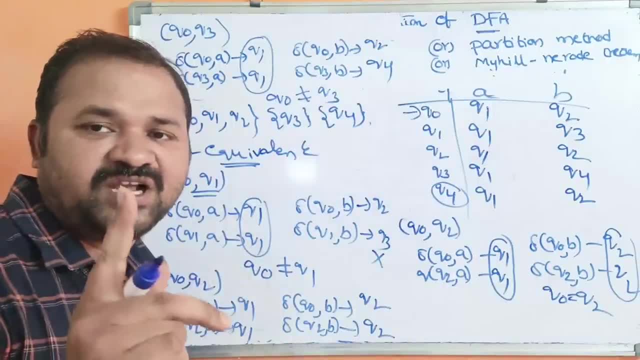 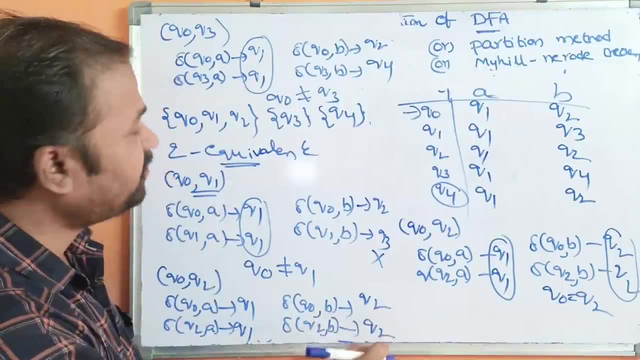 Here we got q1, q1, q1.. So here we got only one state. So that state will be in one set only. So q1 will be in one set only. Here we got q2, q2.. So one state only. 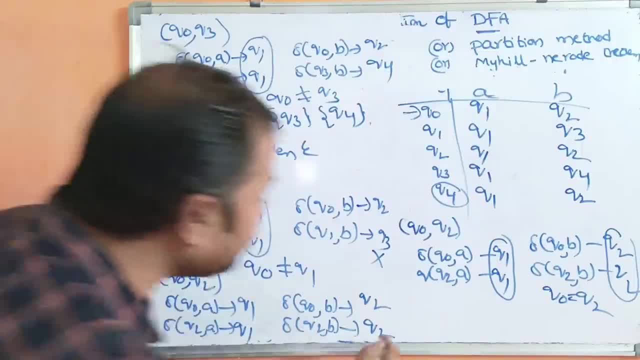 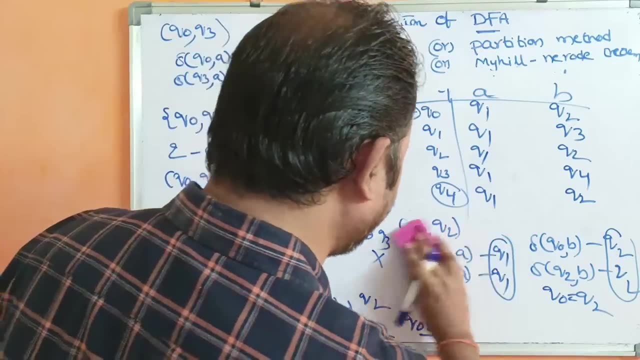 So that will be available in only one set. So we can say that q0 is equals to q2.. q0 is equals to the q2.. q0 is equals to the q2.. So now we can say that two equivalences over. 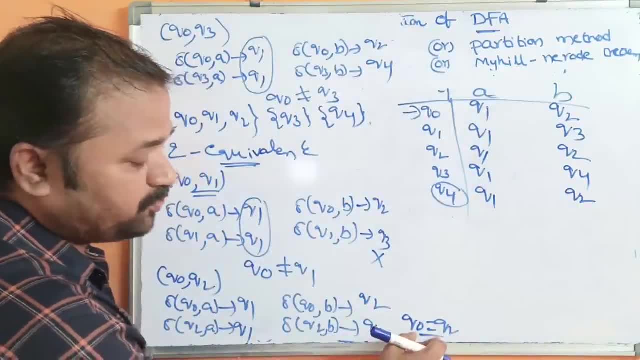 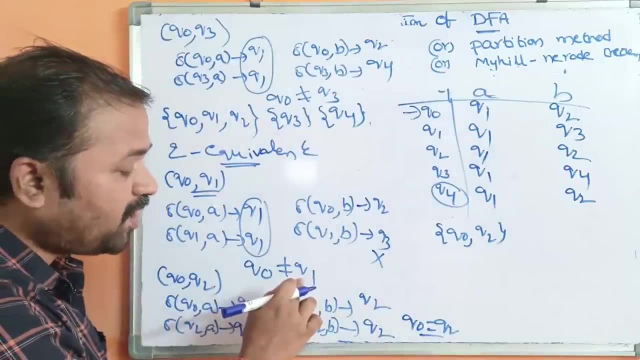 q0 is not equal to q1. But q0 is equals to q2.. q0 and q2 are equal, So q0 and q2 will be in one set. Similarly as q0 and q1 are not equal, So q1 will be in another set. 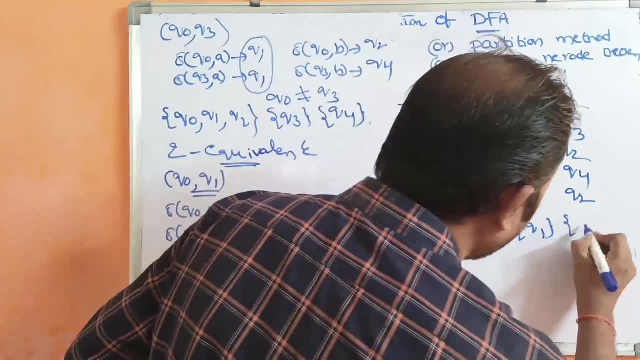 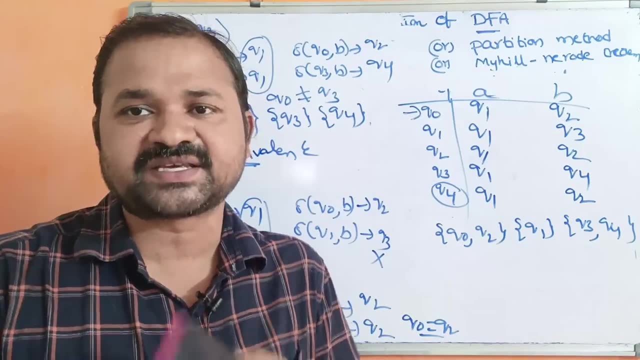 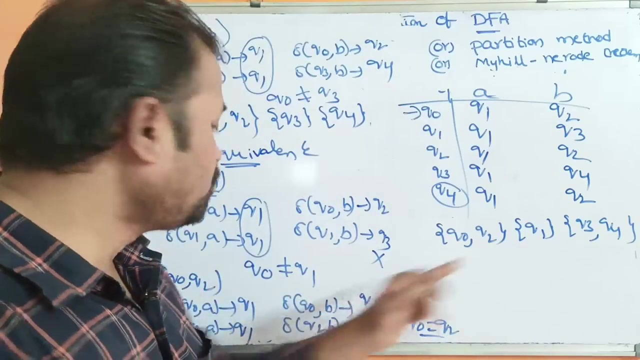 And the remaining sets are q3, q4.. q3, q4.. So second equivalence is over. Now let us calculate third equivalence. If third equivalence result is also same, just like the, if it is similar to the two equivalents, then we can stop the process. 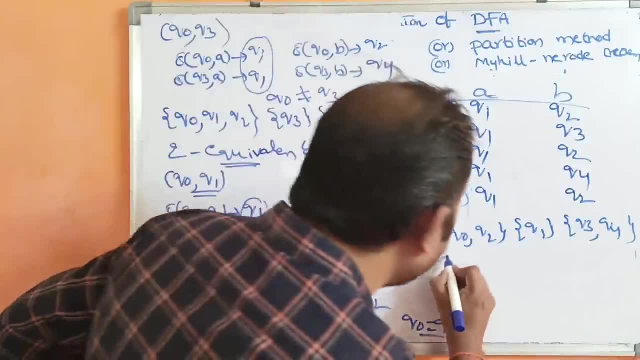 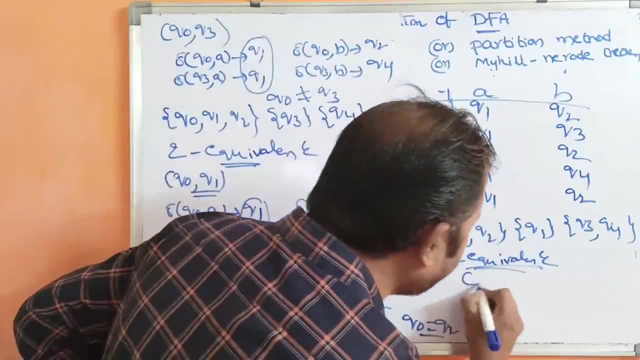 and we can make q0 and q2.. Let us calculate three equivalents. Let us calculate three equivalents. So in three equivalents we have to check whether q0 and q2 are equal or not. Here, third equivalence is calculated based upon the second equivalence. 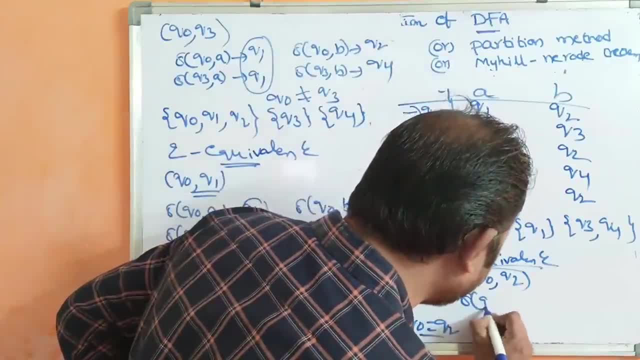 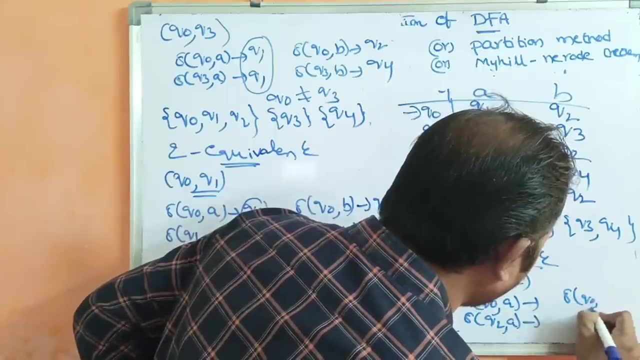 So, based upon this one only, we have to calculate the third equivalence. So delta of q0,a next to delta of q2,a next to delta of q0,b next to delta of q2,b, q0 on a means: q1- q2,b. 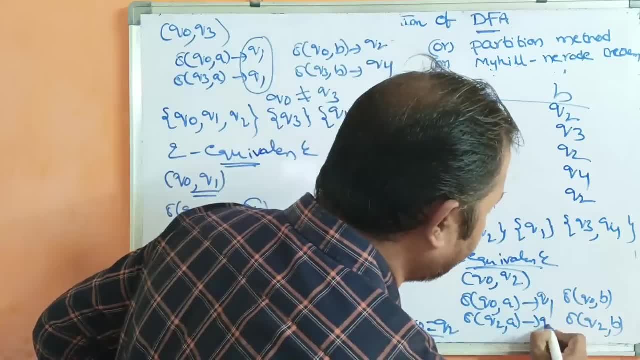 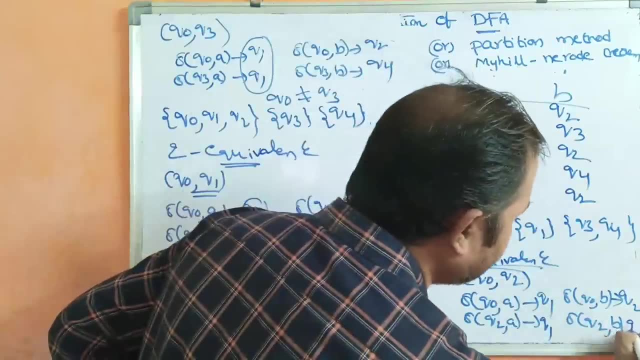 q2,b, q2,b, q2,b, q2,b, q2,b, q2,b. next to q2 on a means q1. next to q0, on b means q2. q2 on b means q2. so here we got only one state, so one state will q1. 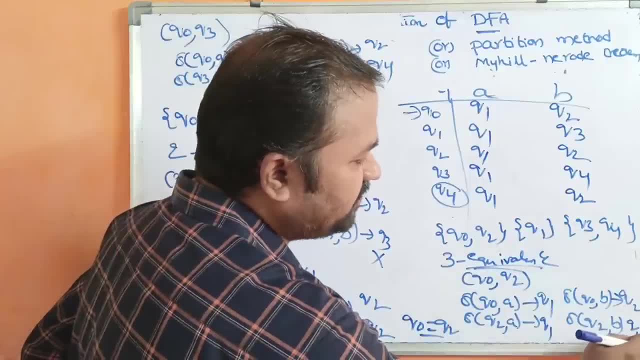 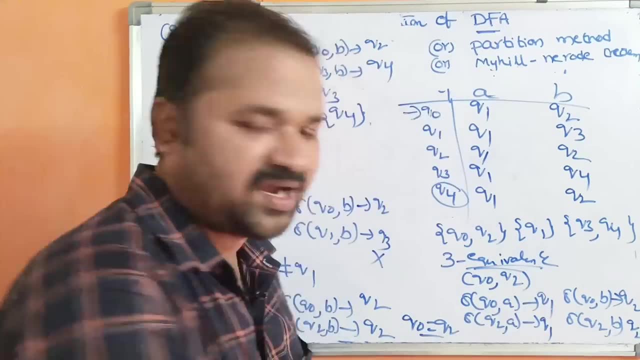 q1 is present in one set only. here also we got only one state, q2. q2 is present in one set only. so here we can conclude that q0 and q2 are equal. q0 and q2 are equal why? because here the result is available in only one set. 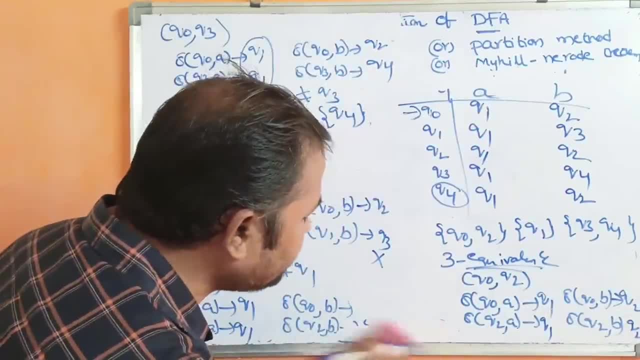 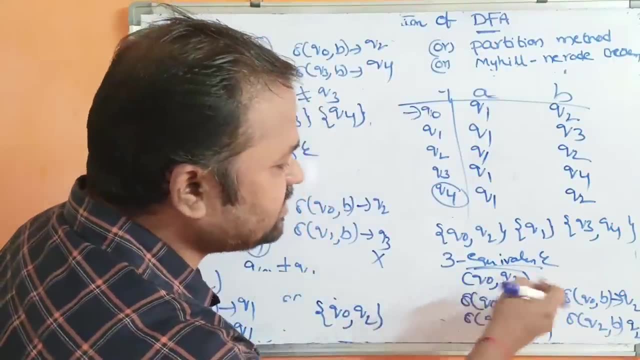 so here we can conclude that. so here we can conclude that here, third equivalence is also similar to the second equivalence. so what is the third equivalence, q0- q2? why? because these two are equal. we can say that these two are equal. q0 is equal to q2. 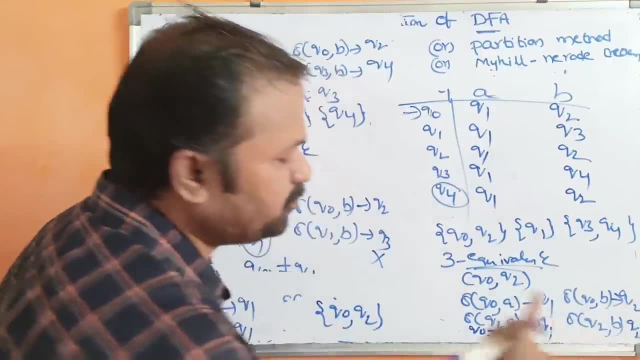 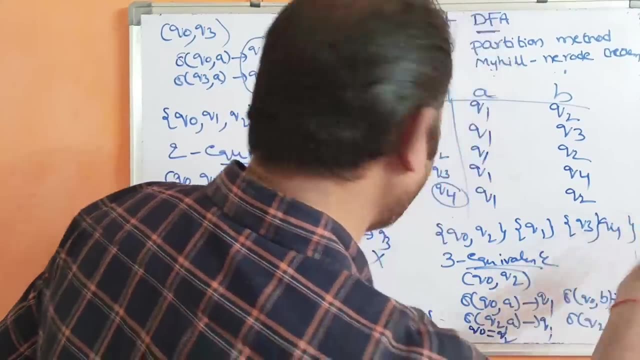 q1. q1: one state, one set only. q2- q2: one state, one set only. so next, q1. I'm sorry. q3 is one state, q4 is another state. these two are different states. q3 is one state. various q1 and q2 are same. 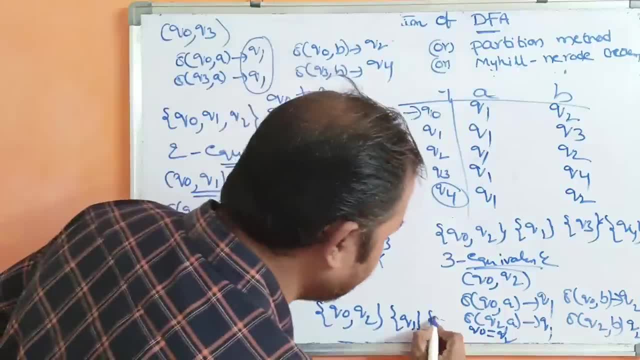 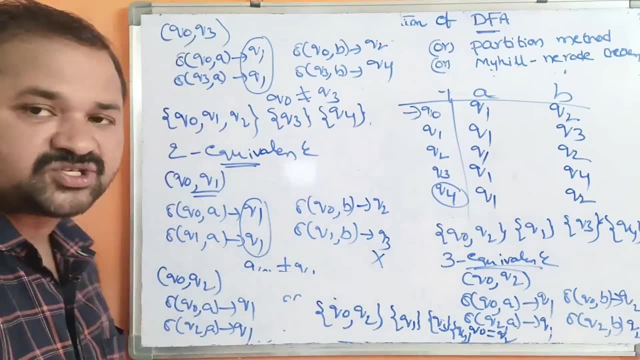 q3 is one state, various q2 are same as Q4 is another set. So Q1, Q3, Q4.. So third equivalence is similar to the second equivalence. So now we can stop the process and here we can combine. we can merge Q0 and Q2.. So we can merge. 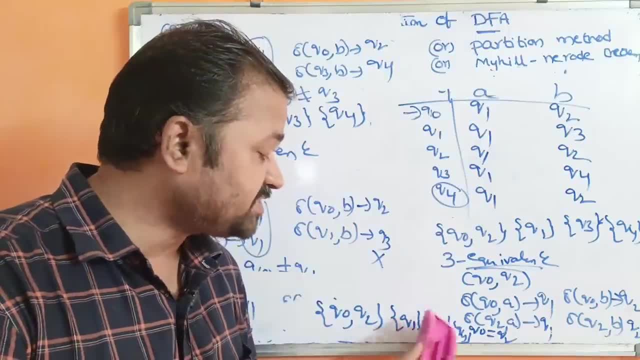 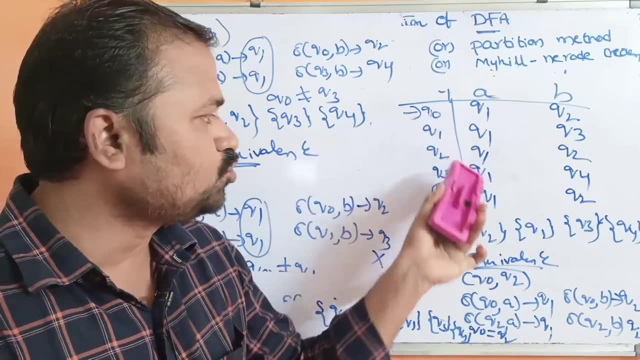 Q0 and Q2 into the one state. Next, Q1 will be the another state, Q3 will be the another state, Q4 will be the another state. Initially we have five states: Q0, Q1, Q2, Q3, Q4.. Now those five. 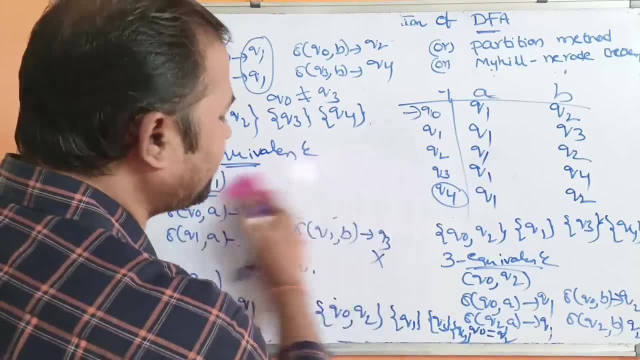 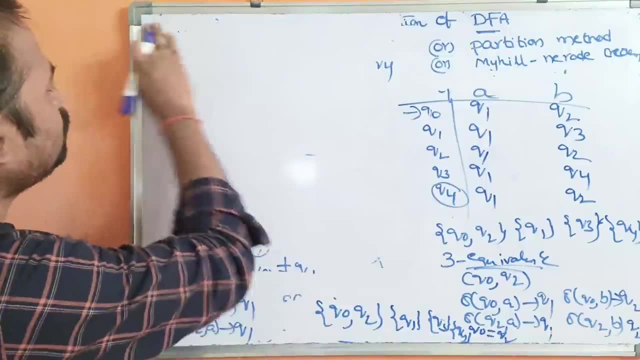 states are reduced to four states. So this is about minimization of DFA. Now we have to construct the DFA. So what is the first state? Q0, Q2.. Q0, Q2 is the first state Here. Q0 is the. 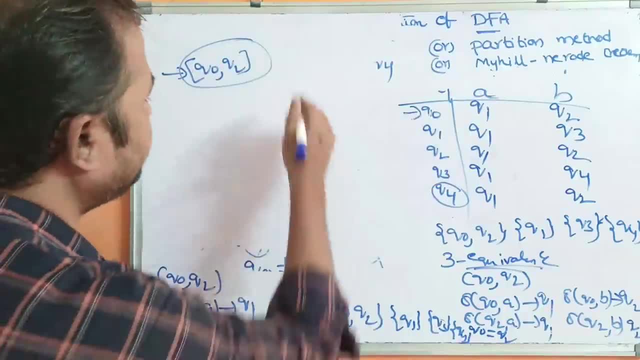 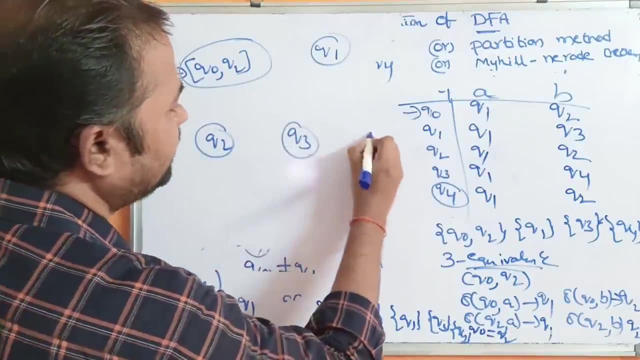 initial state. So let us use arrow symbol. Next, the remaining states are same: Q1, next Q2, next Q3, next to Q4. So five states are reduced to Q1,, Q2,, Q3, Q4. So five states are reduced to four states. So this is about minimization of. 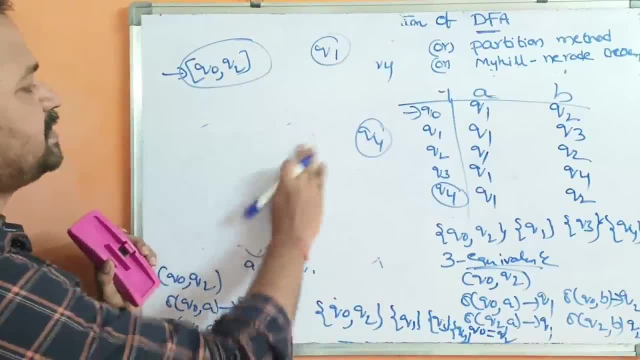 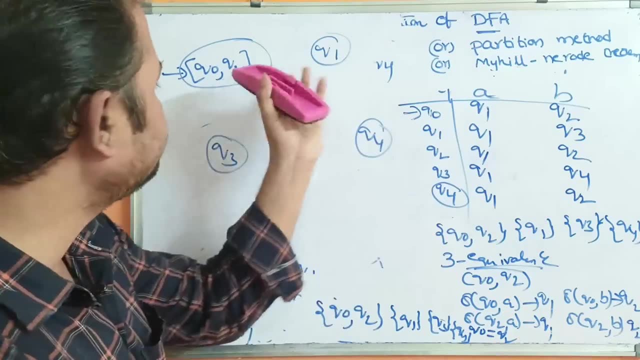 DFA: Q0,, Q2,. I am sorry there is no Q1.. So five states are reduced to four states. So one state, second state, third state, fourth state. Now let us apply the transition. Q0 on A. 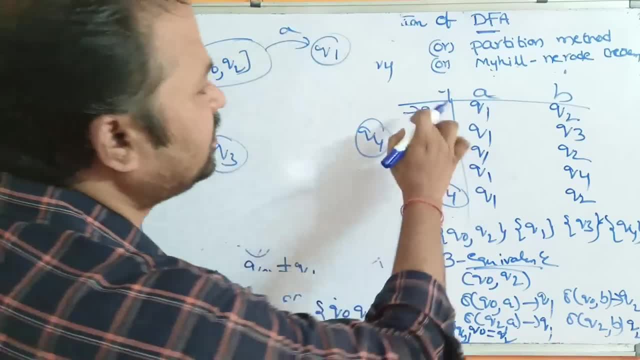 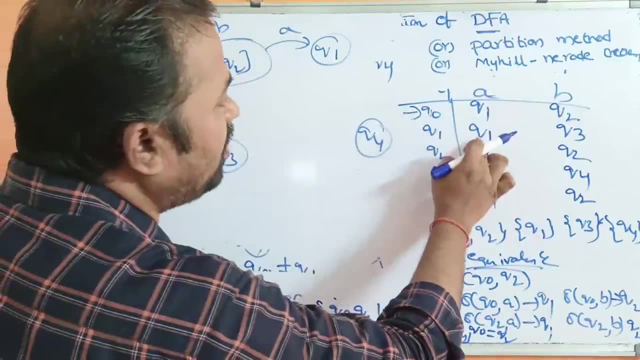 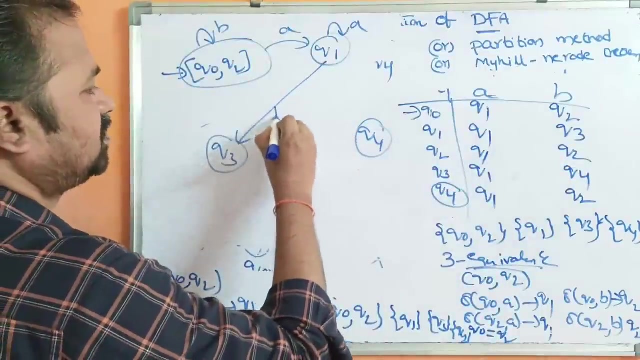 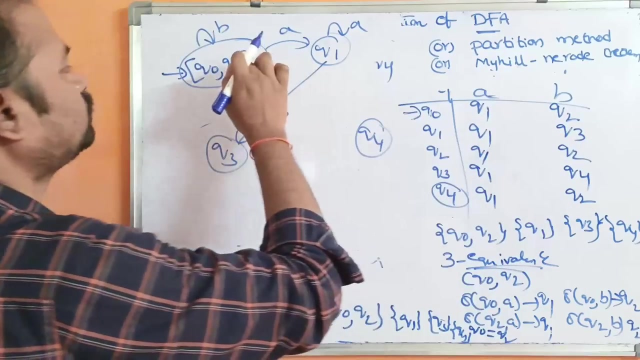 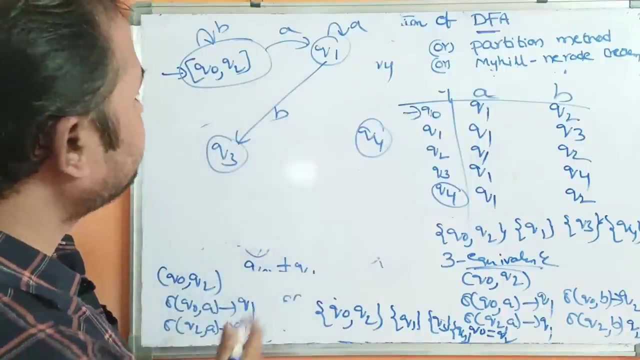 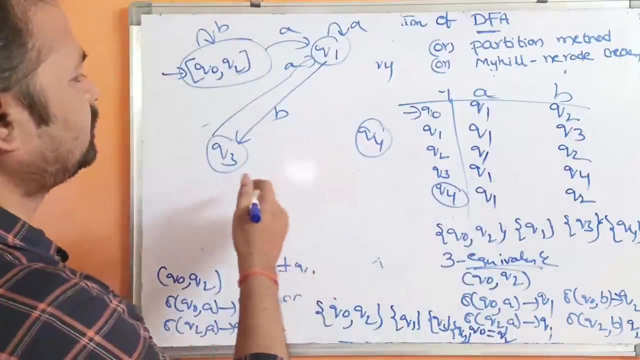 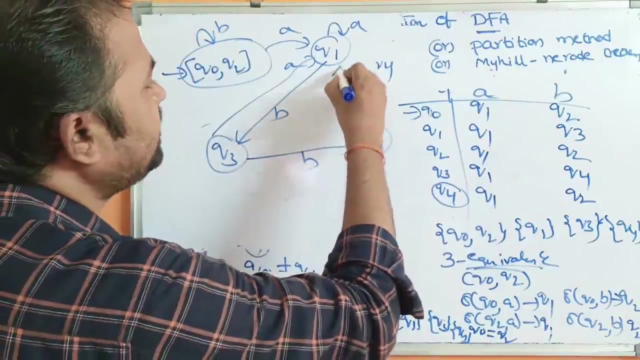 means Q1, Q0 on A means Q1, Q0 on B means Q2.. Q2 means same state only. Next Q1 on A means Q1, self-loop. Next Q1 on B means Q3.. Next Q2, Q2 on A means Q1, Q2 on A means Q1, Q2 on B means Q2, Q2 on B means Q2, same. Next Q3 on A means Q1, Q3 on A means Q1, Q3 on A means Q1, Q3 on B means Q4, Q3 on B means Q4,. next Q4 on A means Q1, Q4 on A means Q1, Q3 on A means Q4, same. 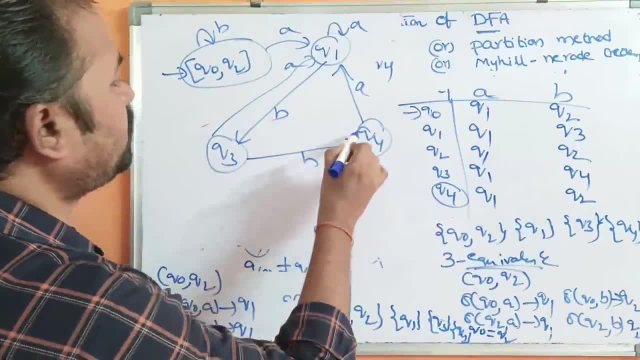 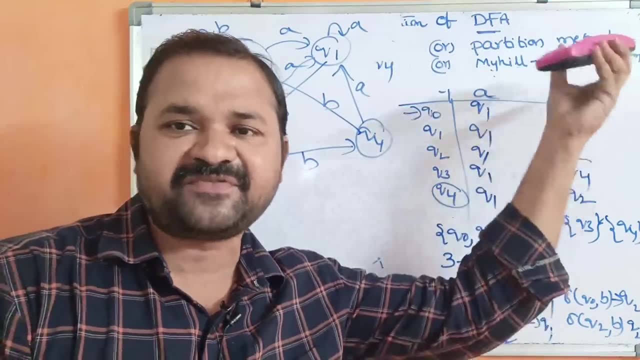 q4 on b means q2, q4 on b means q2. so this is about minimization of dfa. in the similar way, we can minimize nfa also. the only difference between dfa and nfa is in dfa. we can have only one final state. 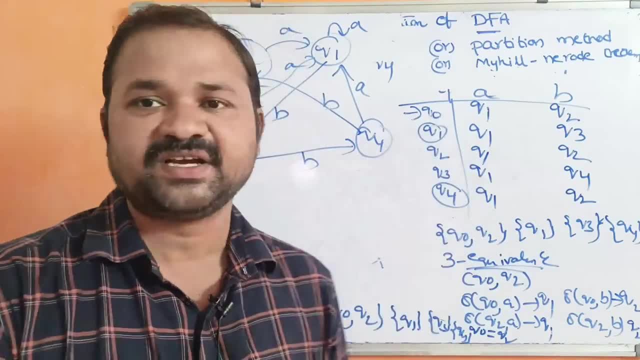 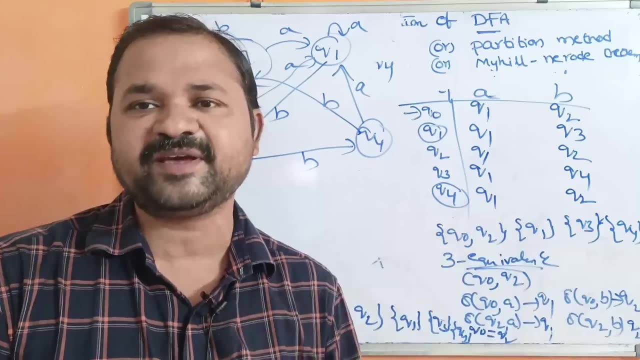 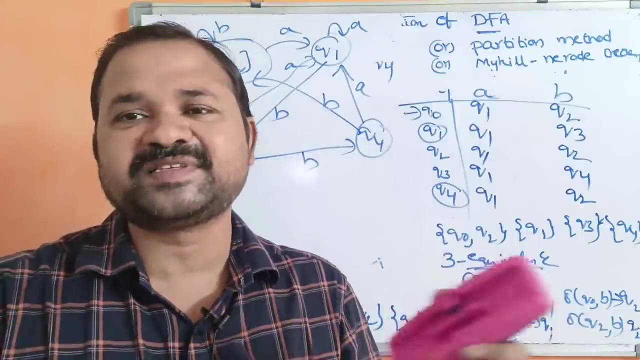 whereas in nfa we may have different final states, so there is no problem. so this can be called as minimization of finite automata, also minimization of dfa or minimization of nfa, same approach we have to follow. dfa means the state must use all the symbols present in the alphabet, so q0, q1, q2, q3. 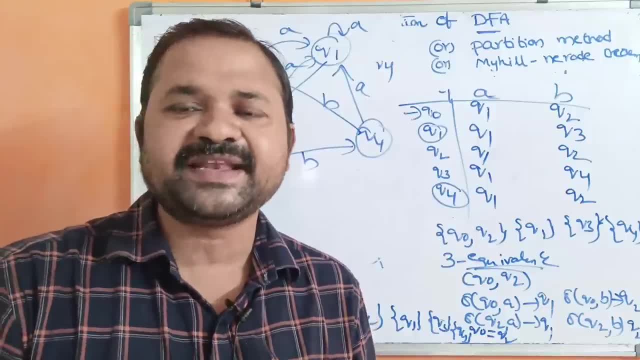 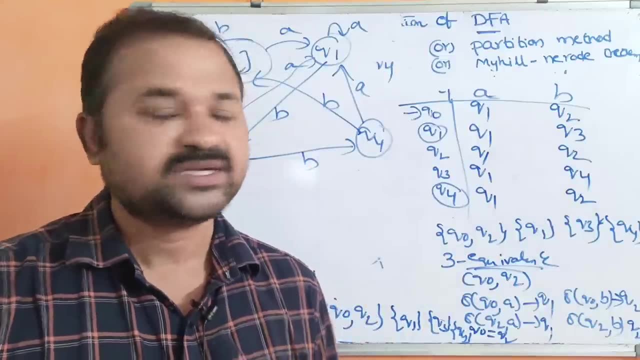 q4, every state must use a and b, whereas nfa means if some transition, if some input symbol is not used by the state, then there is no problem. okay, so in this way we can minimize the finite automata using partition method or equivalence method. now let us see the second method. 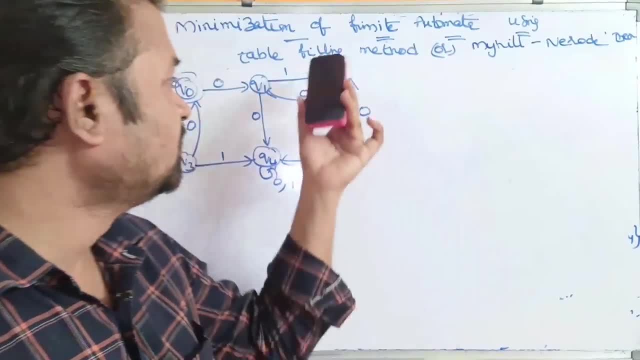 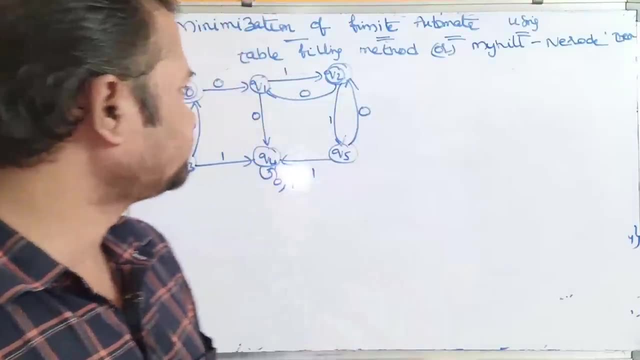 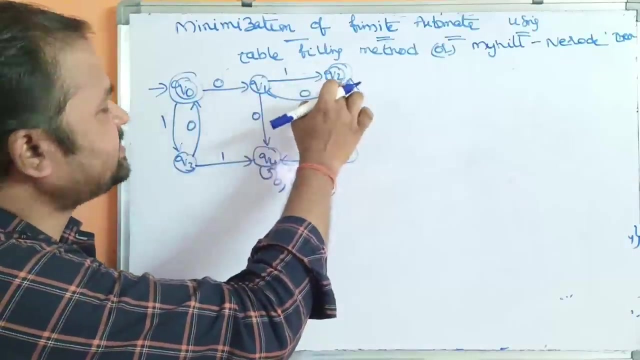 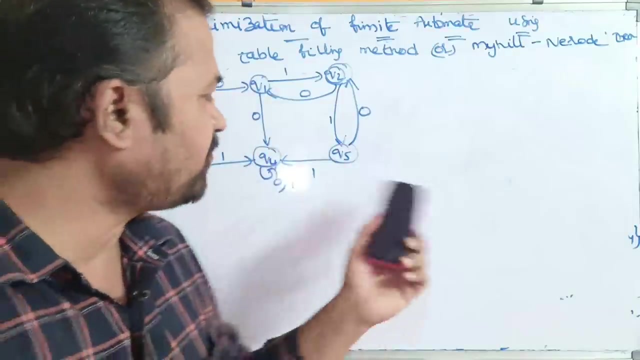 now let us see the second approach: you minimization of finite automata using table filling method or my hill nero theorem. here the finite automata is nfa. why? because here we have two final states: q0 and q2 are the final states, whereas q1, q3, q4, q5 are non-final states. okay, so here, minimization of nfa, whereas 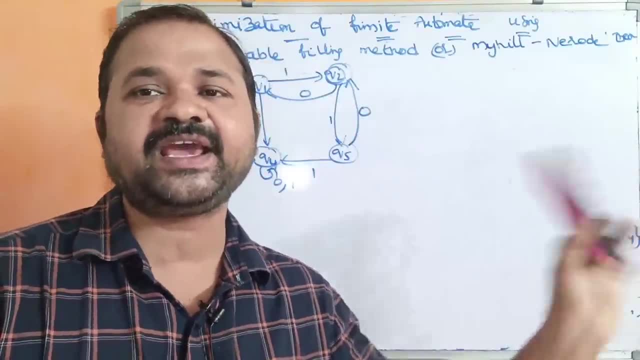 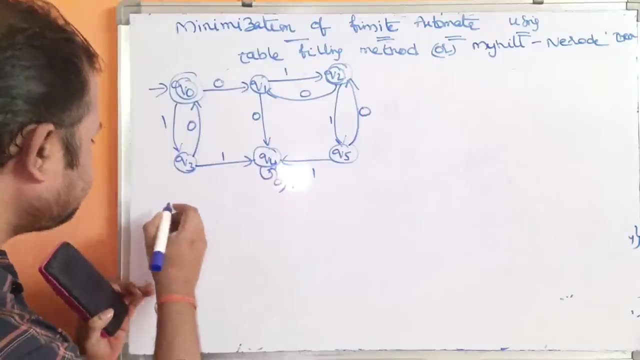 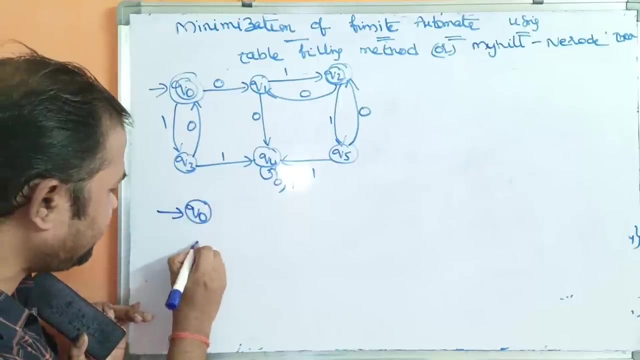 the first example is minimization of dfa, so same manner we have to follow. so first we have to construct the transition table. so let us construct the transition table here. q0 is both initial state as well as final state. q0 is both initial as well as final. q1 is non-final. q2 is also final state, next to q3 state. 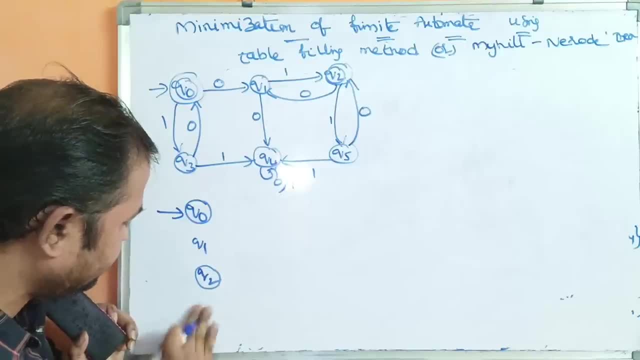 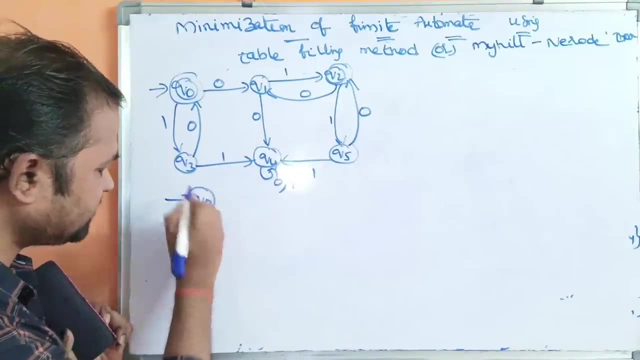 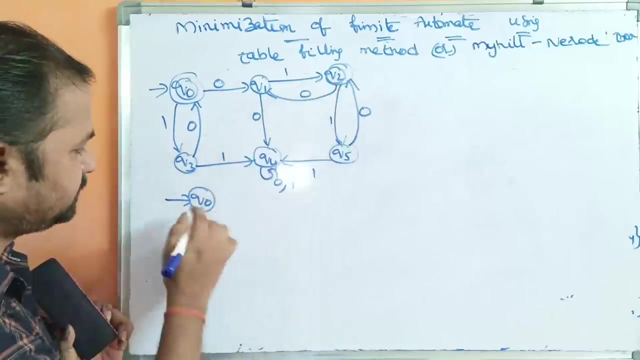 next we have q4 state, next to q5 state, so q naught. so for space constraints, let us write from here. so q naught is starting state as well as final state. next to q1, next to q2 is final state, final state next to q3, q4, q5. 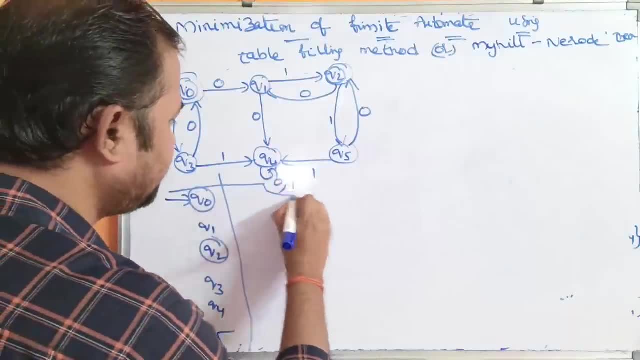 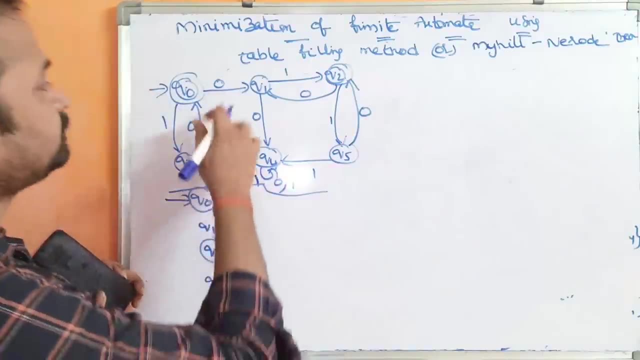 so here the into 12, sir you have. the input symbols are zero and one zero and 1 you not on. zero goes to q1. q not on 1 was to q3. q3 next to q2 is small state. here the input symbols are 0 & 1, 0, &1. q naught on 0 goes to q1. q naught on 1 goes to q3. qth next to q3 next to q1 is small state, just n. false state should be fine with repetition. so this is our behavior. 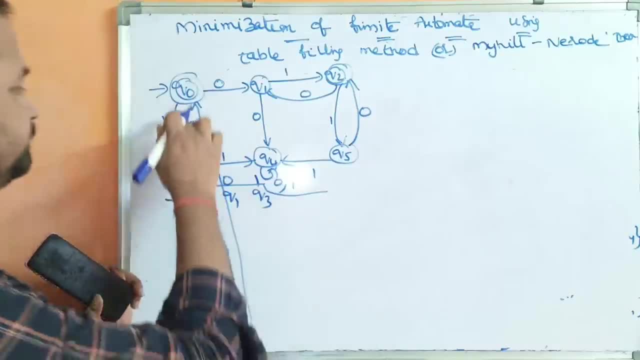 so here the input symbols are 0 & 1, 0 & 1. now we are going to write another equation. we are going to complete all the small cases with the V values. it's upto 40: q1, q1, q1. 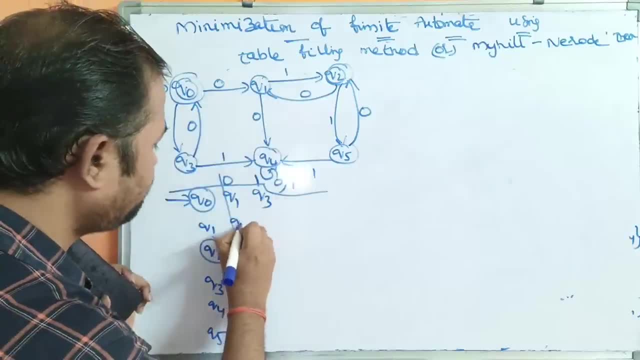 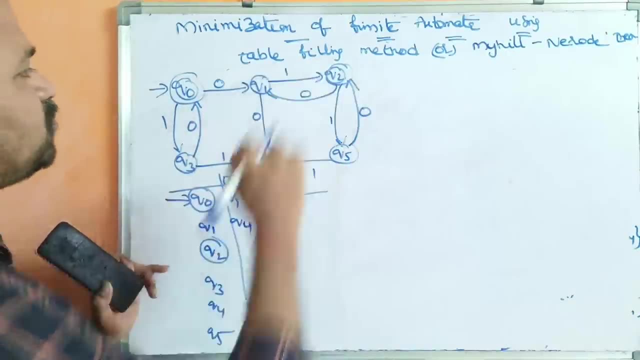 q0 & 1: q1, q1, q1, q1. Next Q1 on 0 goes to Q4.. Next Q1 on 1 goes to Q2.. Q1 on 1 goes to Q2.. 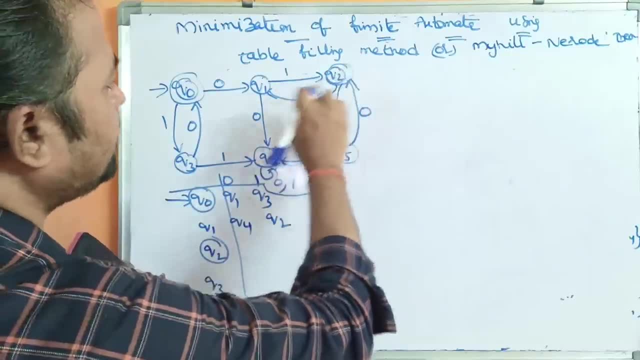 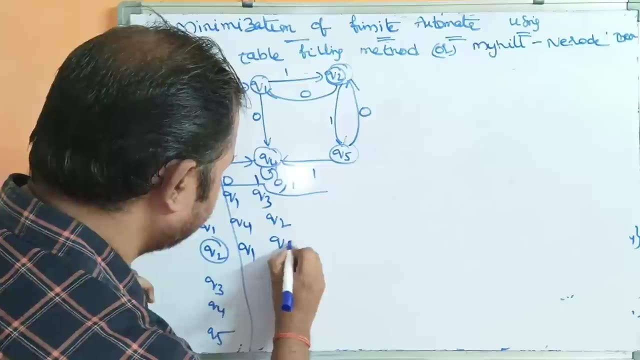 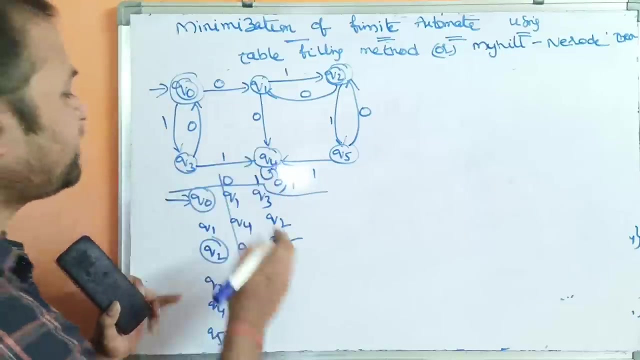 Next Q2 on 0 goes to. Q2 on 0 goes to Q1.. Q2 on 1 goes to Q5.. Next Q3.. Q3 on 0 goes to Q0.. Next Q3 on 1 goes to Q4.. 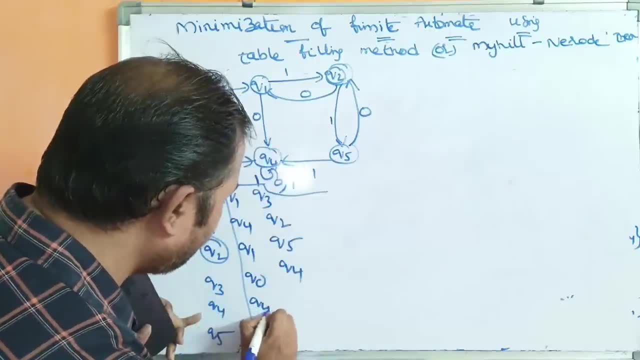 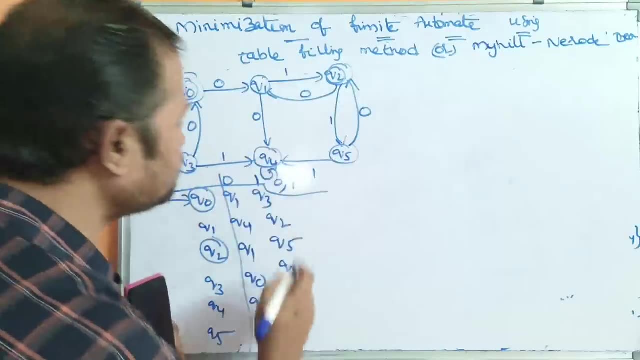 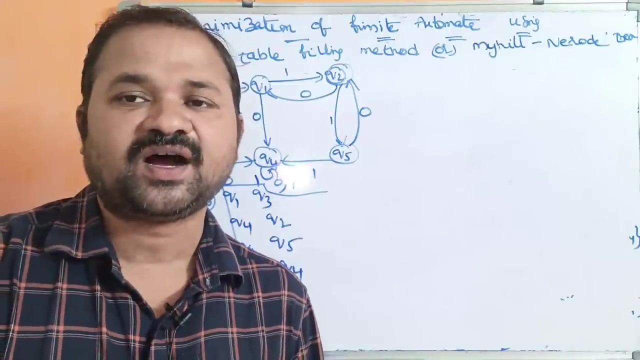 Next Q4 on 0 goes to Q4. only. Next Q5 on 0 goes to Q2.. Q5 on 1 goes to Q4.. So transition table construction is over. Now we have to construct one more table. 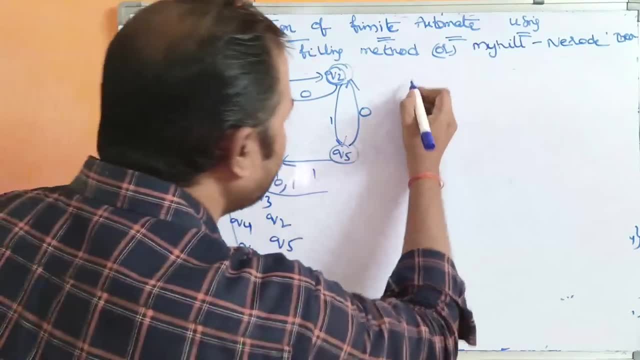 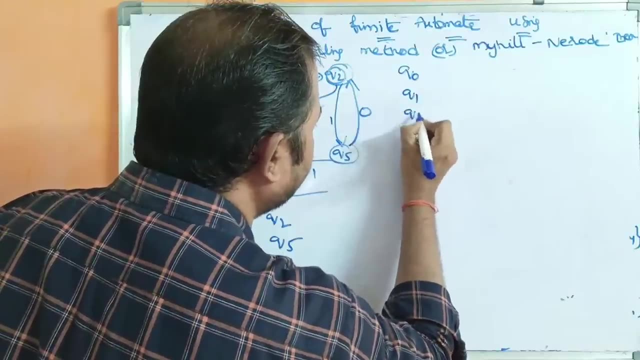 The table will be like this. So here, what are the states? Q9. Q1. Q2. Q3. Q4.. So let us write them in vertical manner, So Q0. Q1. Q2.. 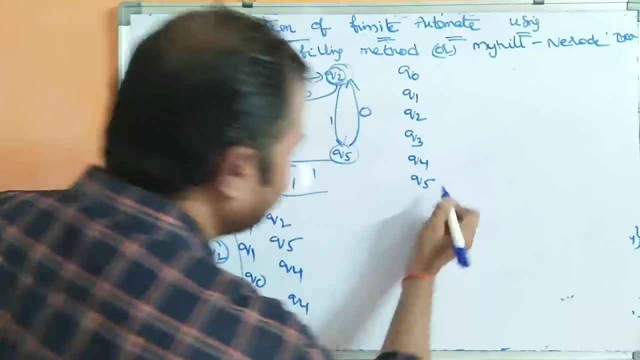 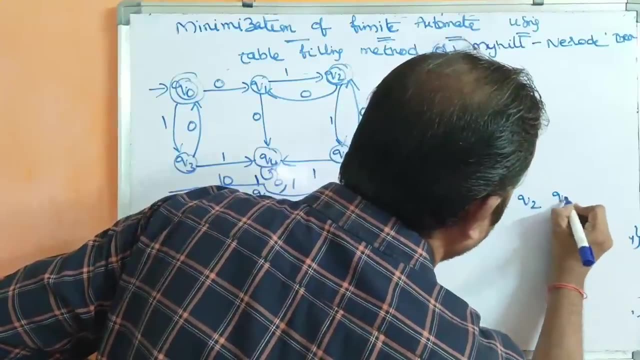 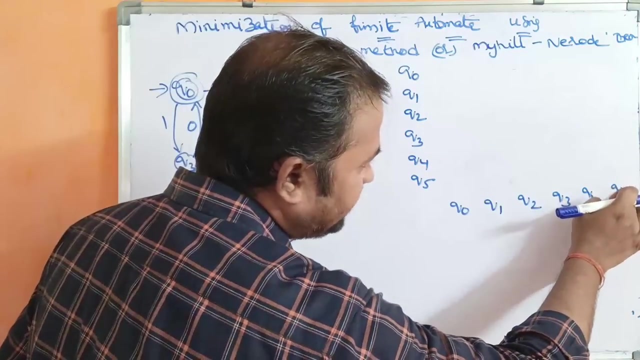 Q3., Q4., Q5.. Next, let us write the states in horizontal manner, So Q0., Q1., Q2., Q3., Q4. And Q5. Let us eliminate the last state in horizontal And the first state in. 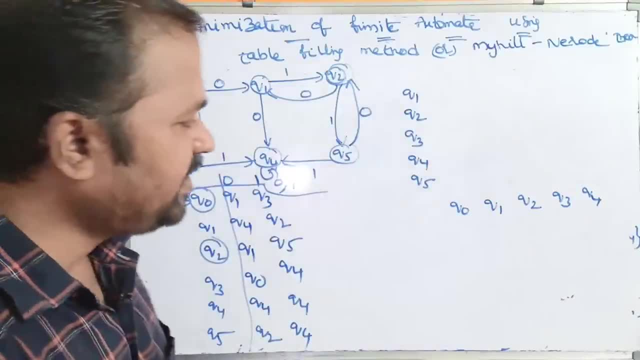 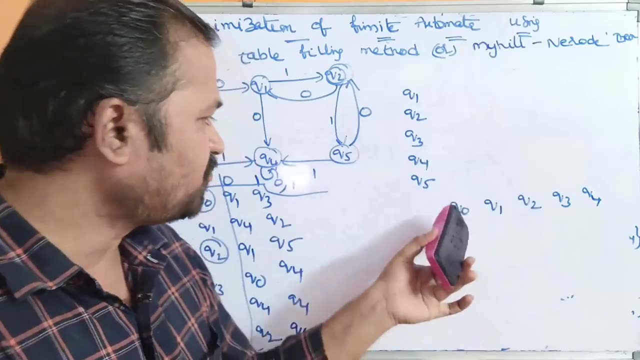 Vertical. Okay, Now we have to establish the connections from each state to remaining all other states, So from Q0 to Q1, Q2, Q3,, Q4, Q5.. Likewise, we have to establish the connections. 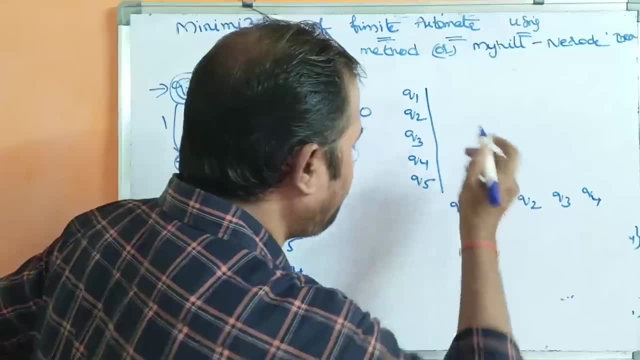 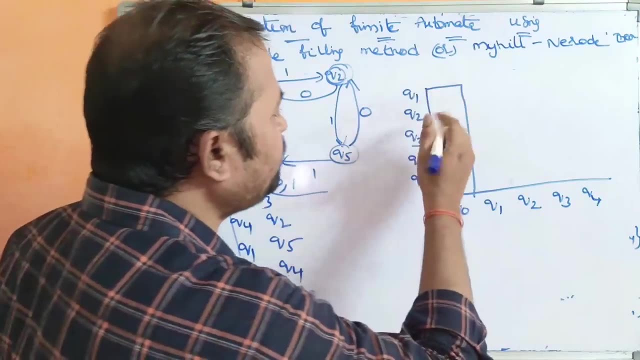 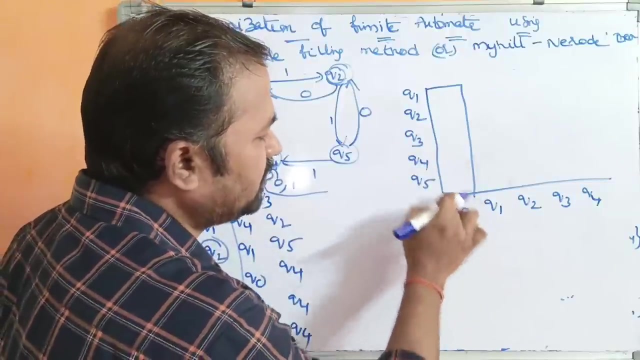 So let us see how we can do that. So, from Q0 to Q1.. From Q1 to Q2, Q3, Q4, Q5.. From Q0 to Q2, Q3,. From Q0 to Q4, Q5. 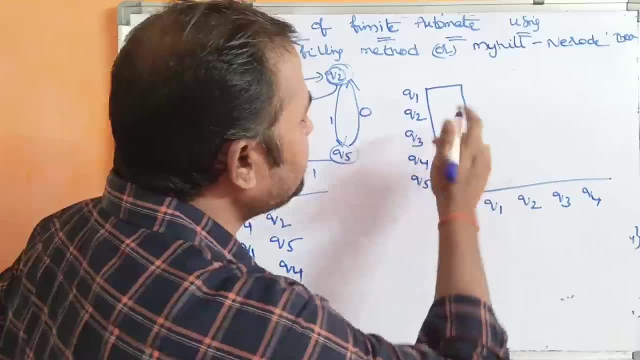 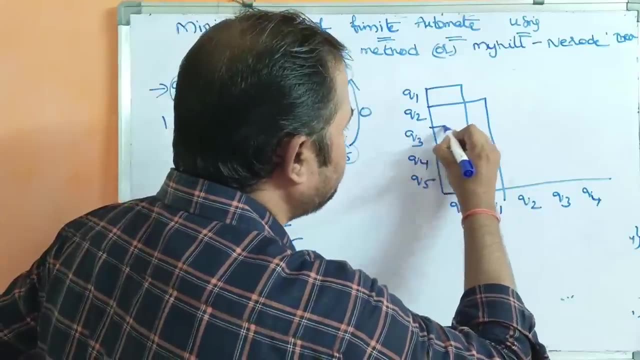 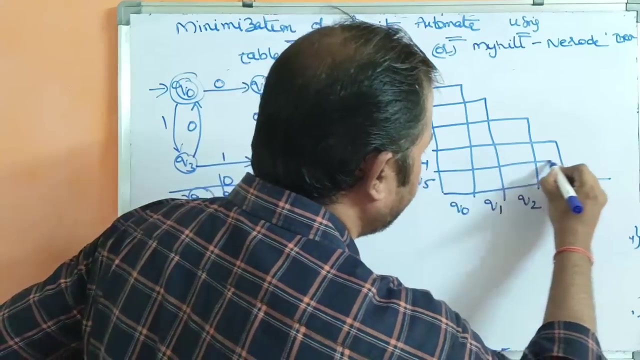 From Q0 to Q5.. Likewise, from Q1 to Q2,, Q3,, Q4, Q5.. Next from Q2 to remaining all states. Next from Q3 to remaining all states. Next from Q4 to remaining all states. 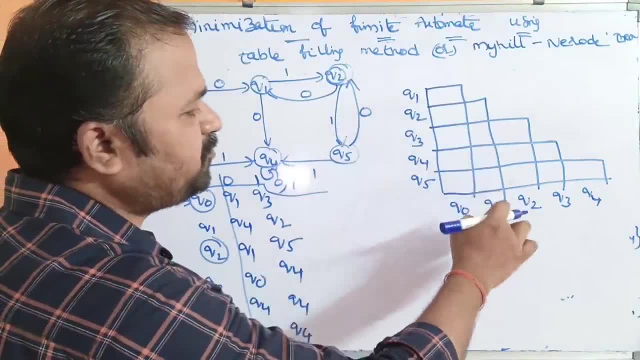 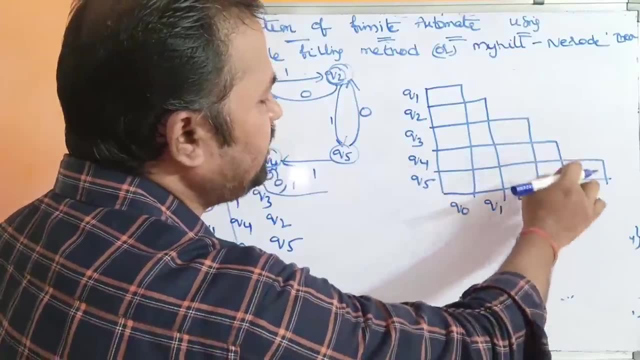 So Q0 to Q1.. Q2, Q3, Q4, Q5.. Next to Q1 to Q2.. Q2, Q3, Q4, Q5, Q2, Q2, Q3, Q4, Q5,, Q3, Q4, Q5, Q4, Q2, Q4, Q5, Q5. 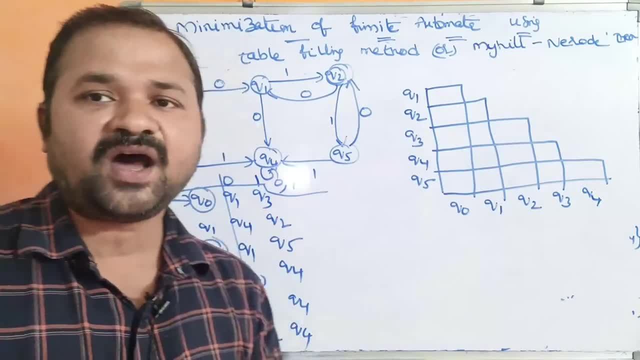 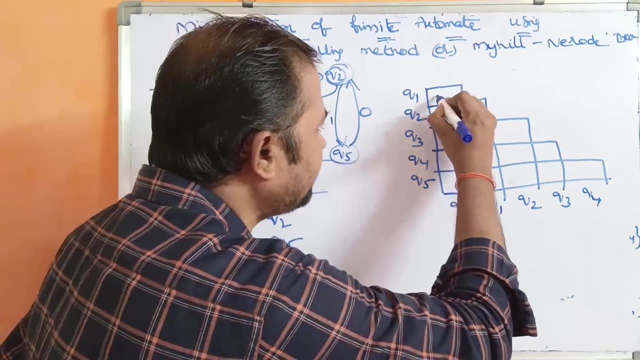 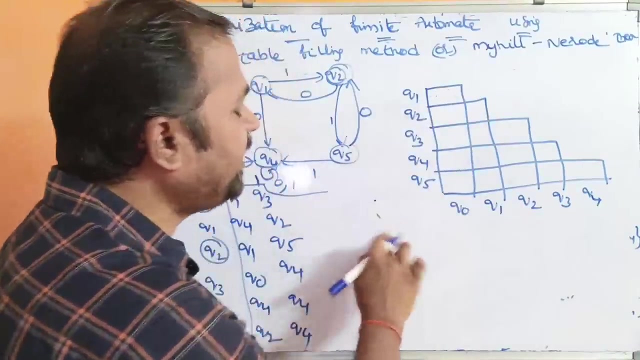 So we have to draw a table like this. Now we have to mark the states, So when we can do the marking Here. for marking we can use either a tick mark or cross mark. We can use any symbol. Here we can mark a pair. 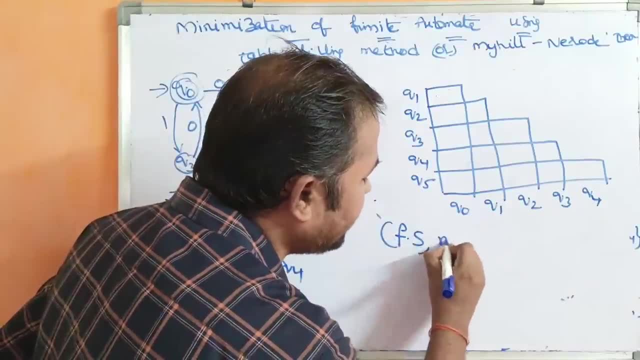 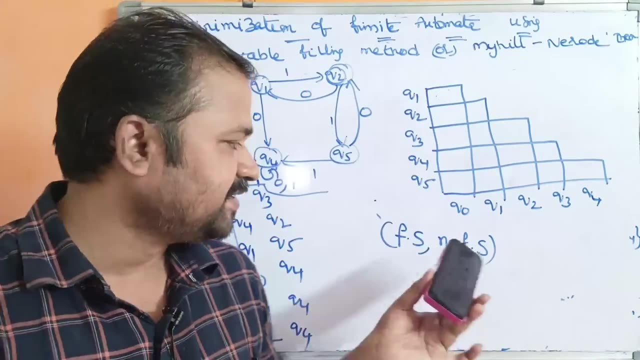 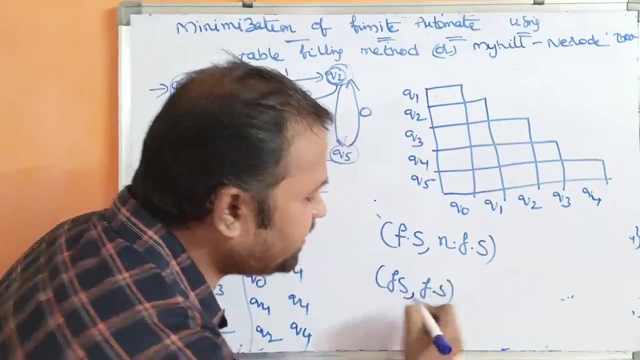 If the pair contains a final state as well as non-final state, We can mark a pair if the pair contains a final state as well as non-final state. If the pair contains only final states, then marking is not possible. Simply, we have to leave that pair. 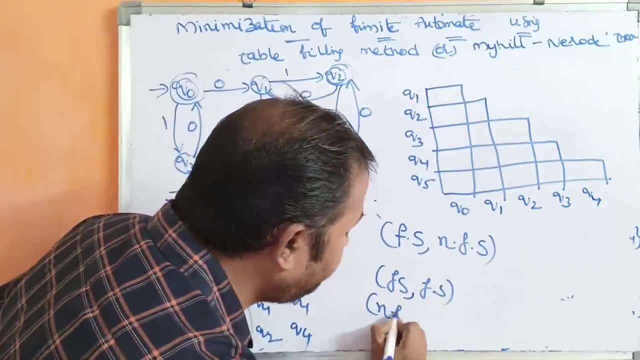 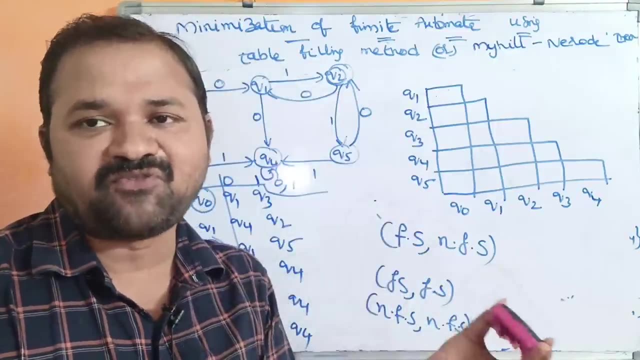 We have to leave that box. Likewise, if the pair contains non-final states, then also we have to leave the box. So when we can do the marking, If one state is final state and the other state is non-final state, Here what are the final states? 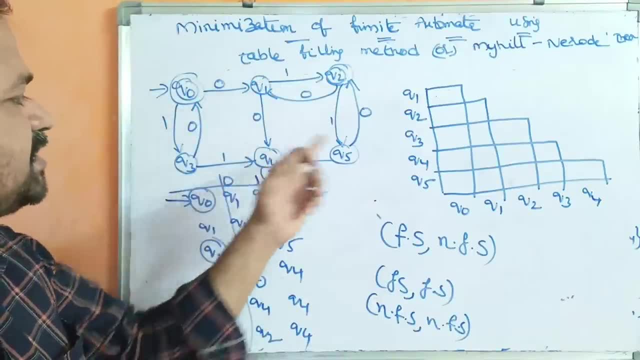 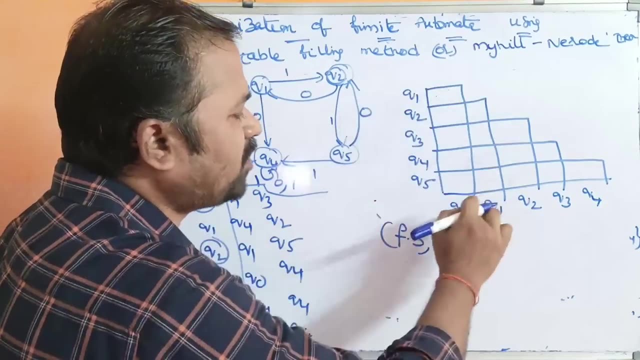 Q0 and Q2 are the final states, Whereas Q1, Q3,, Q4, Q5 are non-final states. So now let us see here: So Q1 to Q1, Q0.. So this pair is nothing, but this box belongs to Q1, Q0. 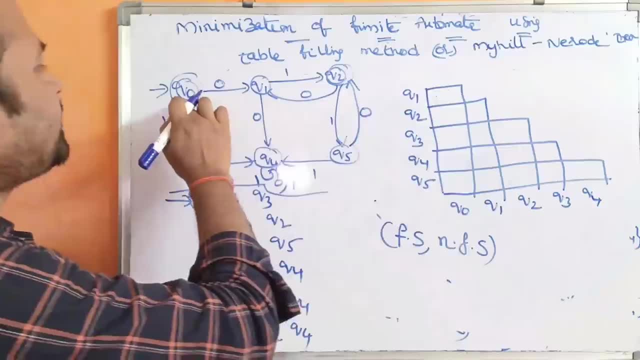 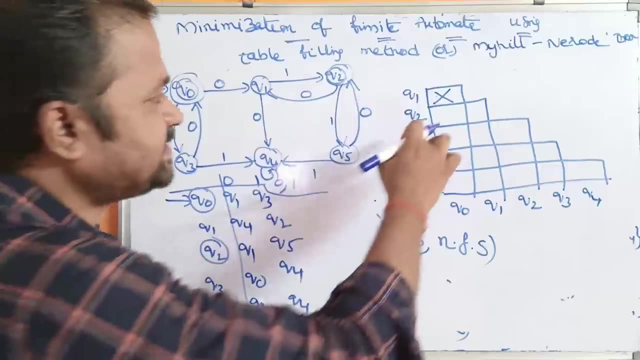 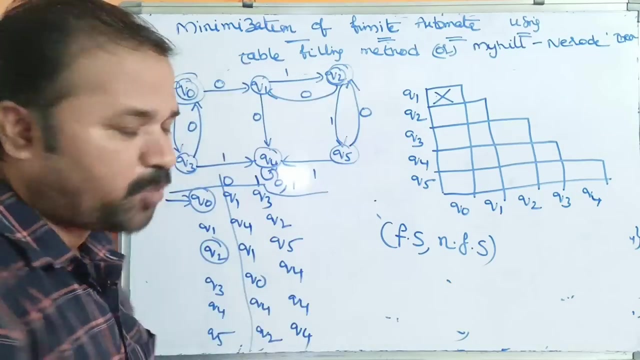 Or we can call as Q0, Q1.. Q0 is final state, Whereas Q1. Q1 is non-final state, So we can mark this box Next. this box belongs to Q2, Q0.. But Q2, Q0, both are final states. 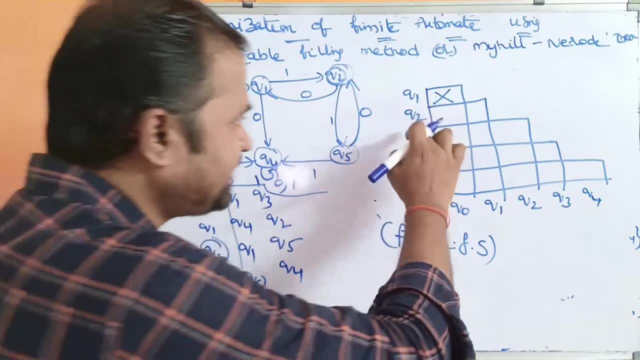 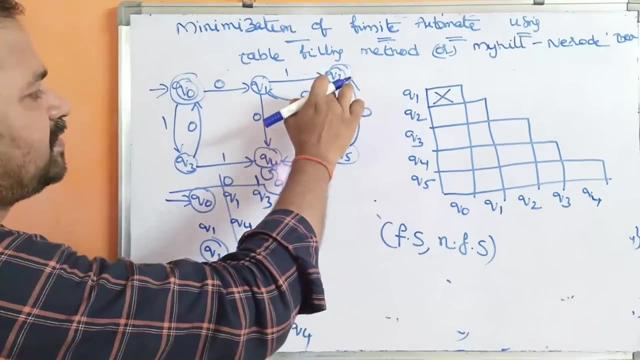 So, simply, we have to leave that box. Next, Q2.. Let us see this pair. So this pair belongs to Q2, Q1.. Q2, Q1.. So one is final state, Another one is non-final state. 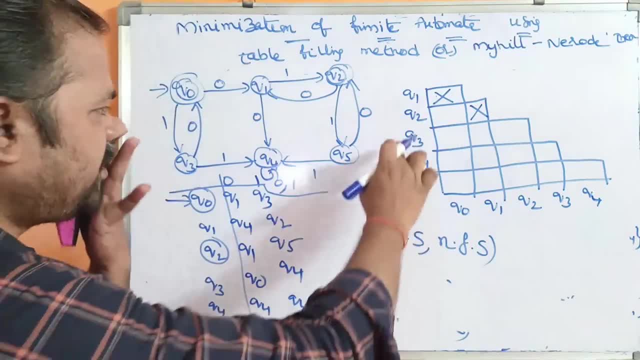 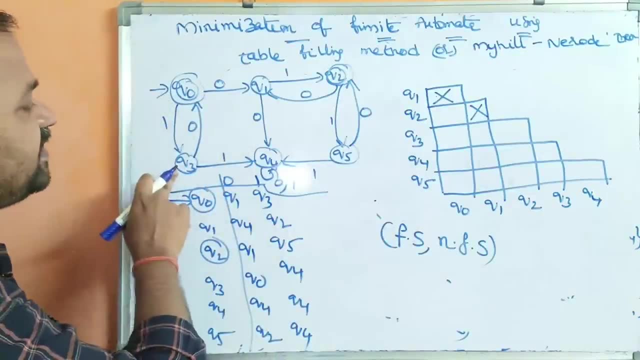 So we can mark this box. Next one: Q3, Q0.. Or we can also call it as Q0, Q3.. Q0, Q3.. One is final state, Another one is non-final state, So we can mark this box. 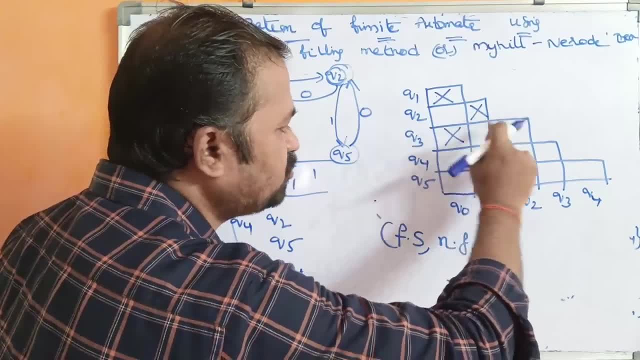 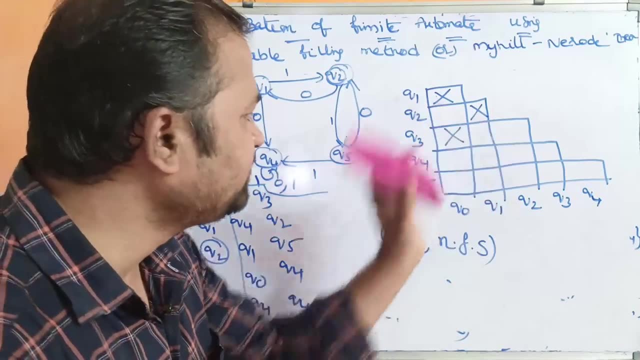 Next, this box belongs to Q3, Q1.. Q3, Q1.. So Q3 is non-final state. Q1 is non-final state, So simply leave this one. Next one: Q3, Q2.. Q3, Q2.. 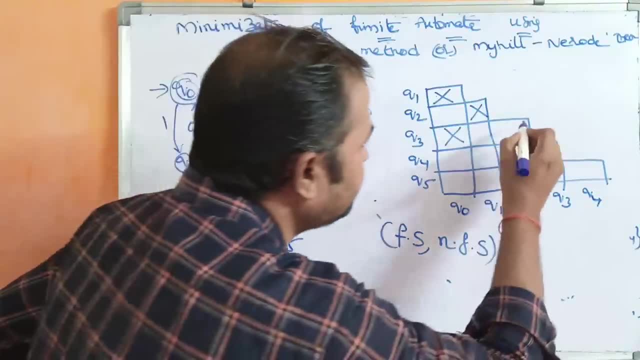 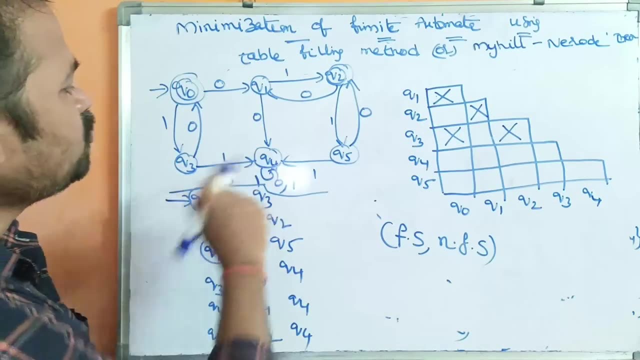 So one is non-final state, Another one is final state, So mark this pair, Mark this box. Next one: Q4, Q0.. So Q0 is final state, Q4 is non-final state, So mark this box. 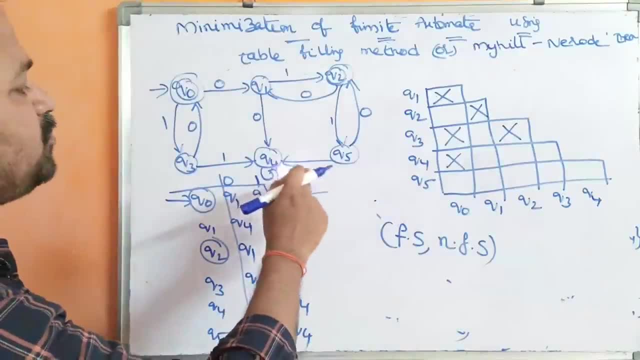 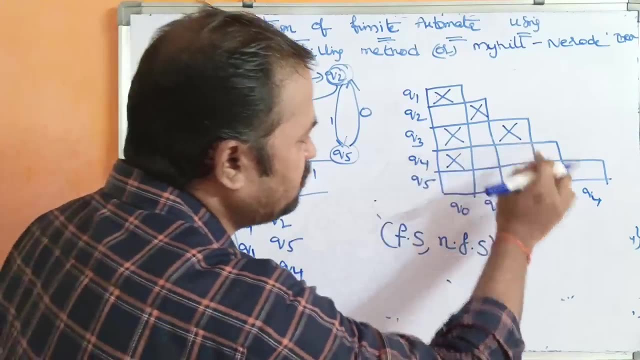 Next one, this pair: Q4, Q1.. Q4, Q1.. So Q4 is non-final state. Q1 is non-final state, So leave this box Next. Q4, Q2.. Q4, Q2.. 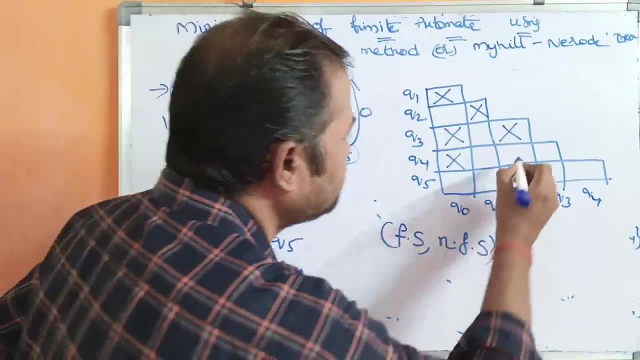 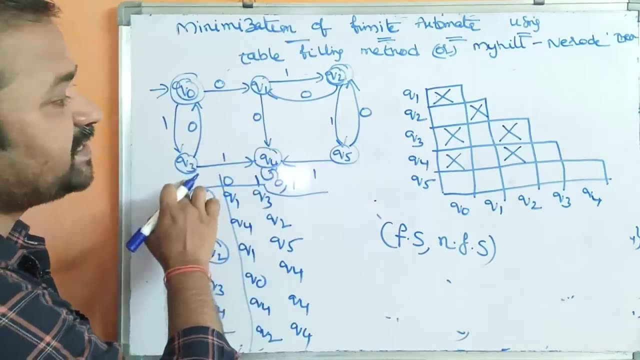 So Q4 is non-final state. Q2 is final state, So mark this box Next: Q4, Q3.. Q4, Q3.. Q4 is non-final state. Q3 is non-final state, So both are non-final states. 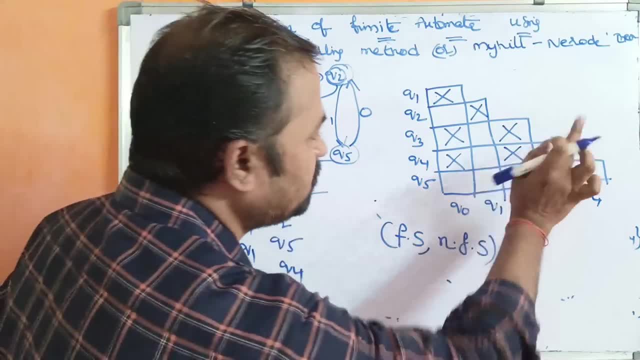 So leave this box. Next one: Q5, Q0.. Q5, Q0.. So Q0 is final state, Q5 is non-final state, So mark this box Next: Q5, Q1.. Q5, Q1.. 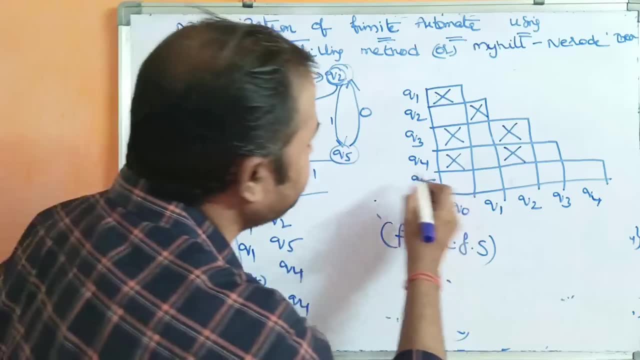 So Q5 is non-final state. Q1 is also non-final state, So leave this box. Next: Q5, Q2.. Q2 is final state. Q3 is non-final state, So mark this box. Next: Q5, Q1.. 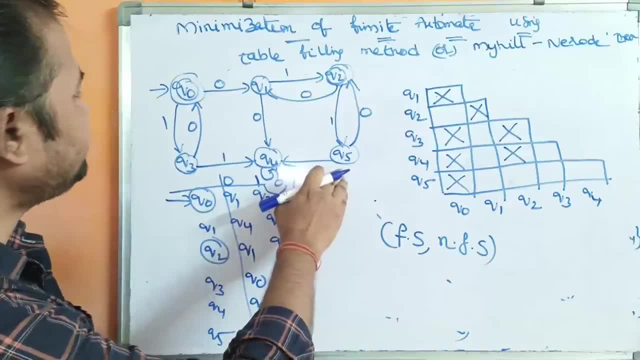 Q5, Q1.. So Q5 is non-final state. Q1 is also non-final state, So leave this box. Next, Q5, Q2.. Q2 is final state. Q5 is non-final state, So leave this box. 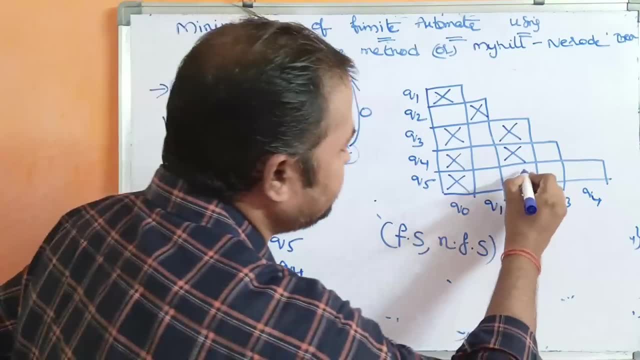 Next Q5, Q3.. Q5, Q3.. Q5 is non-final, Q3 is non-final, So leave this box. Next, Q5, Q4.. So Q5, Q4.. Both are non-final states. 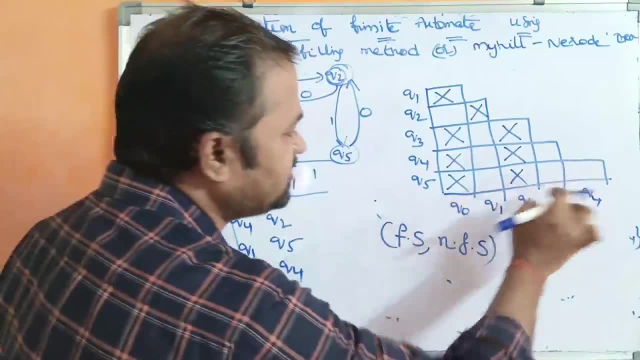 So leave this box. So here, what are the? what are the boxes? those are unmarked. So here, what are the boxes? those are unmarked. So here, what are the boxes? those are unmarked. So here, what are the boxes? those are unmarked. 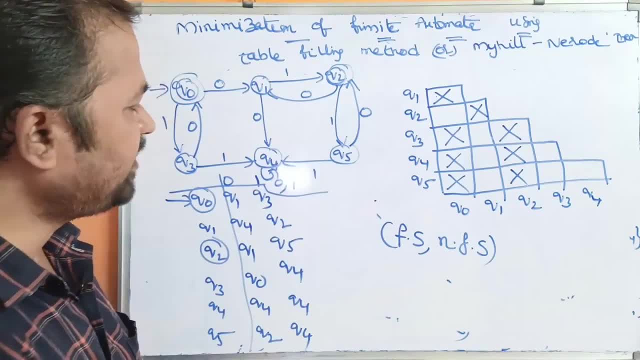 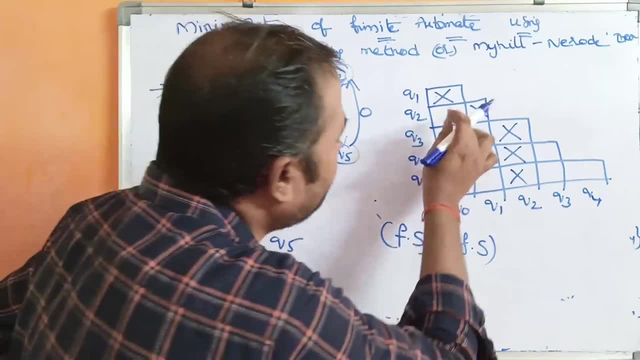 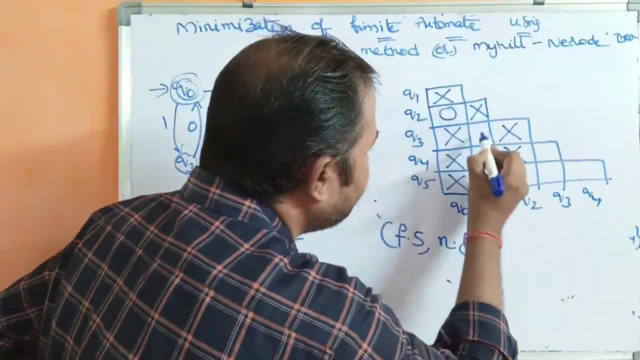 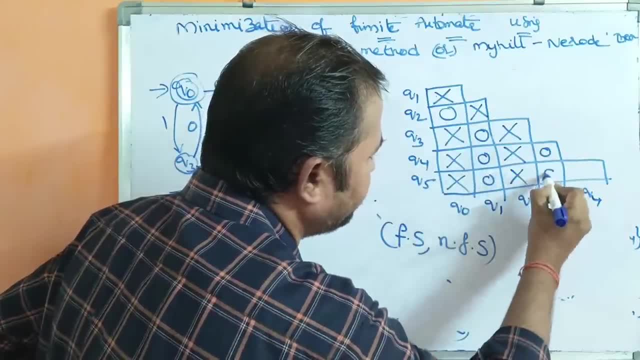 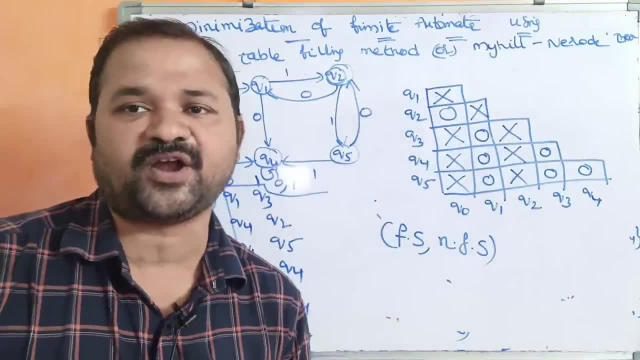 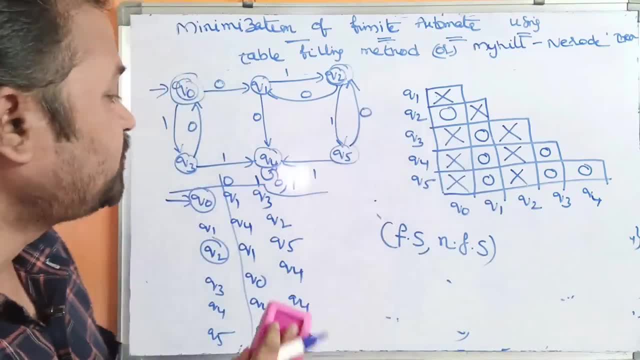 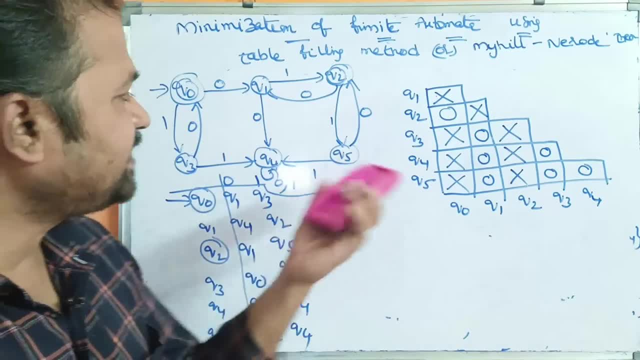 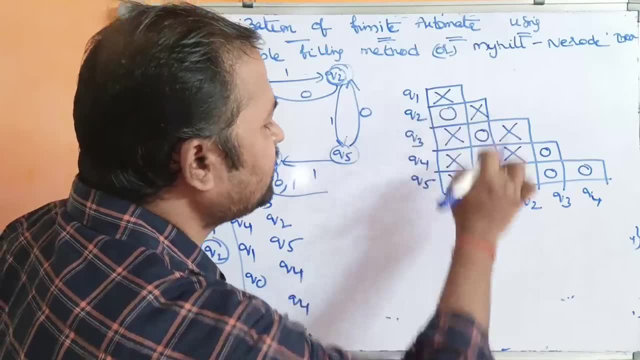 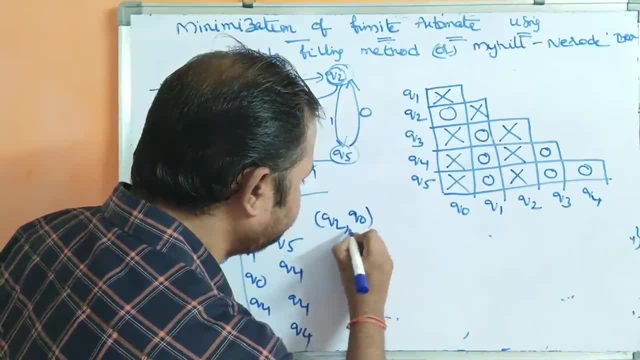 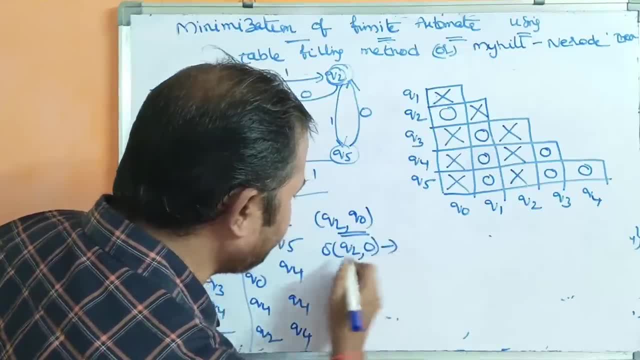 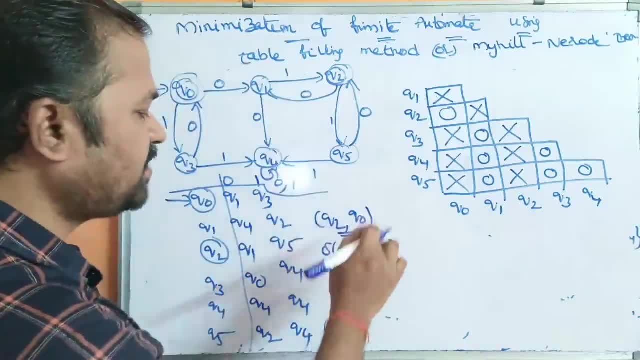 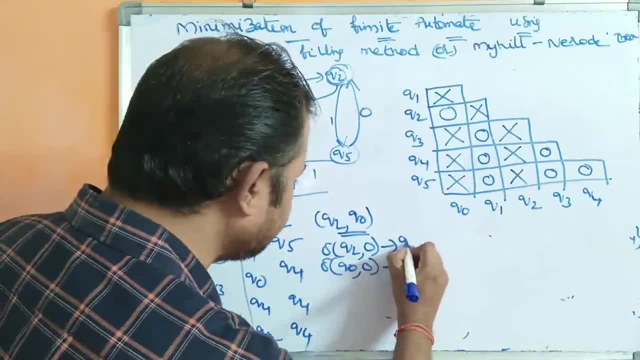 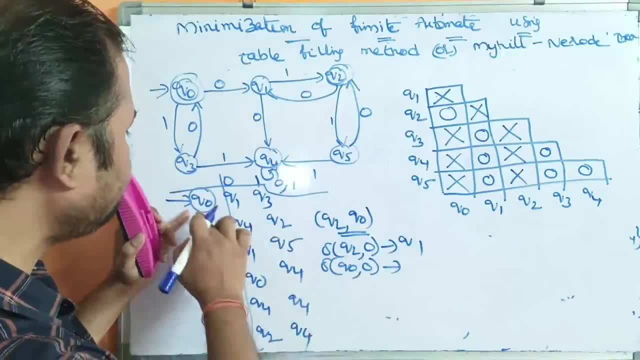 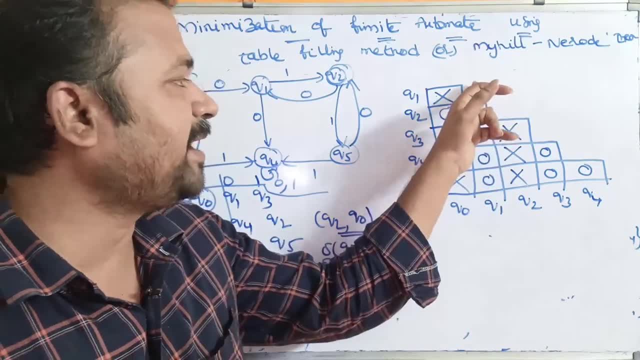 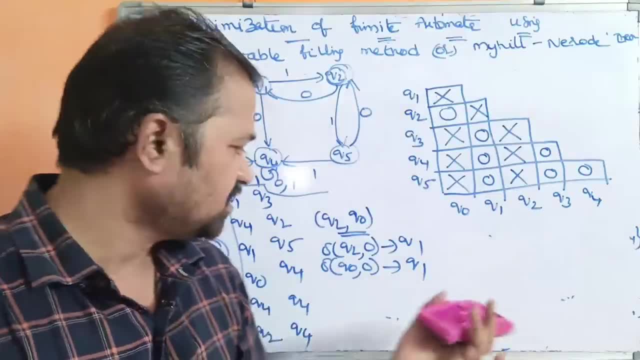 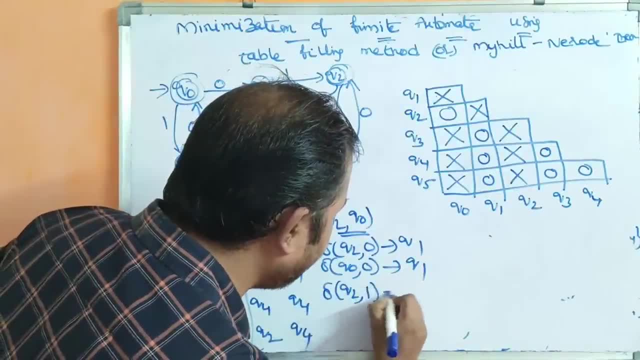 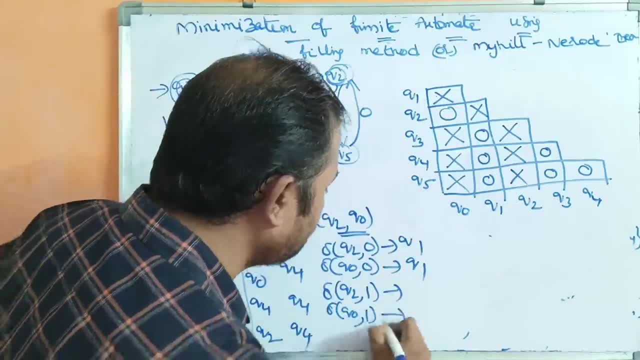 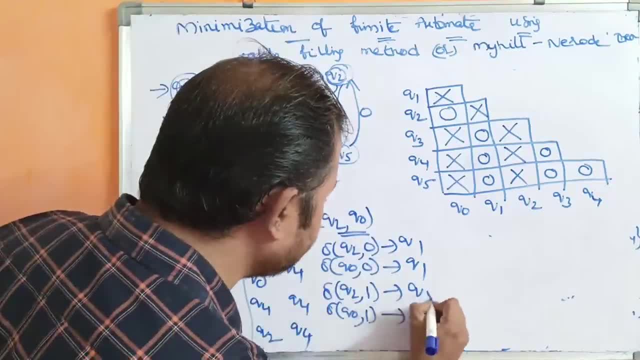 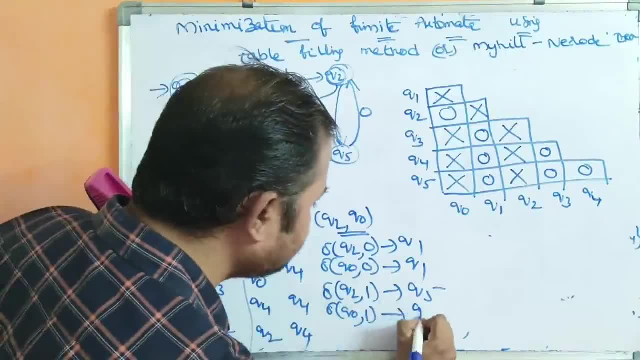 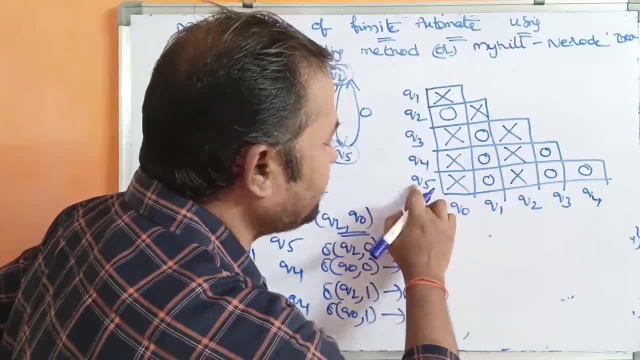 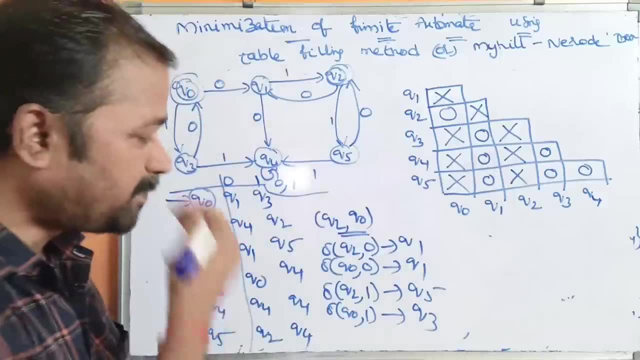 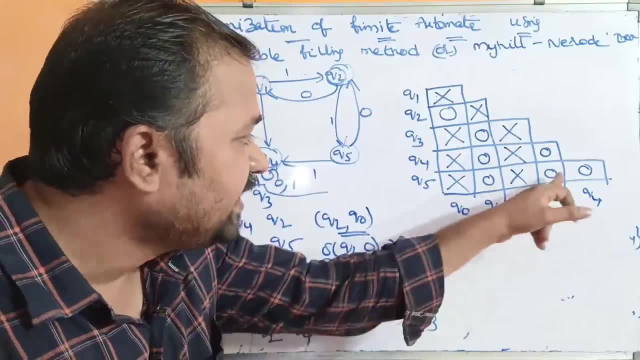 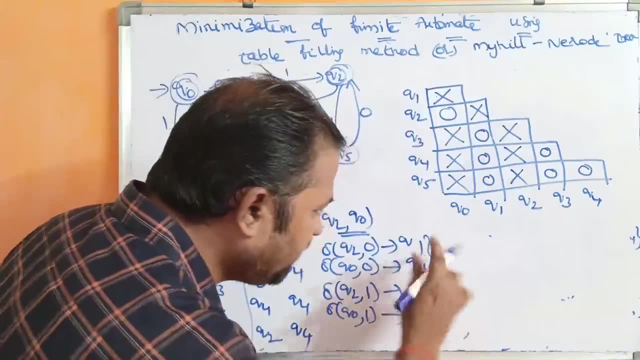 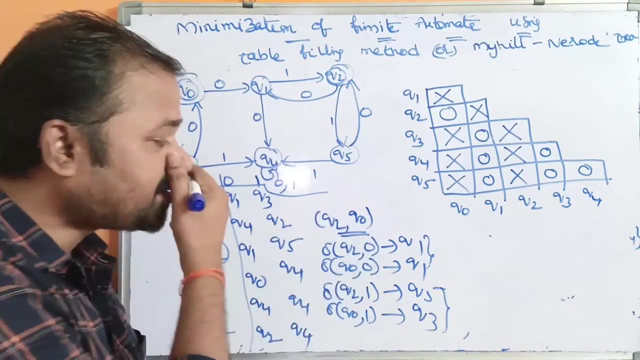 possible Why? Because Q5, Q3.. If this pair is marked, If one of the pair is marked, Either this one or this one, If one of this pair is marked, If either this pair or this pair, If one of this pair is marked, Then we can mark Q2- Q0.. But here the problem is we don't have Q1- Q1. 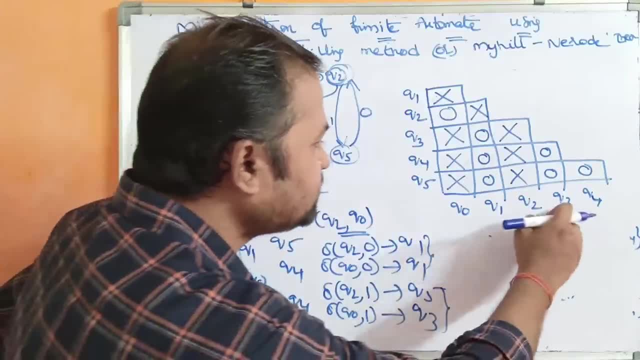 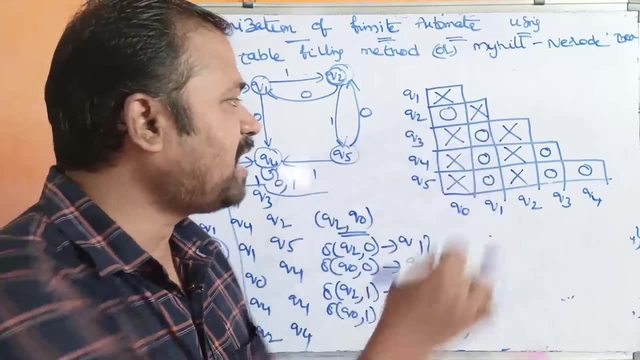 pair And if we observe Q5, Q3.. So Q3, Q5 means this pair. This pair is not marked. So marking Q2, Q0 is not possible, So we have to leave this pair as it is. Now let us see the next one, That 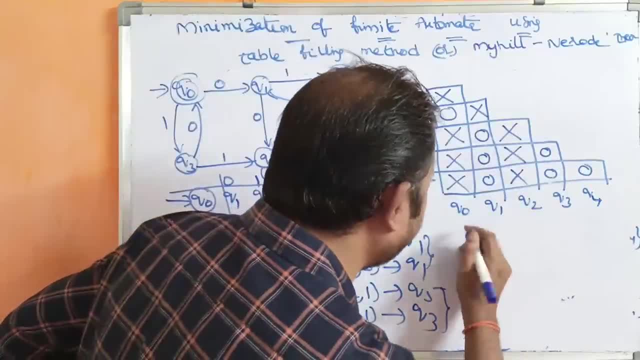 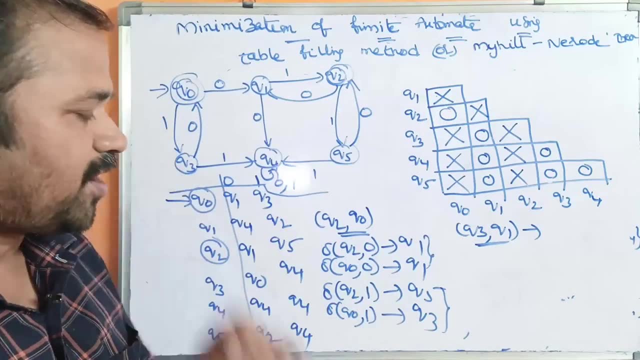 is: what is this pair? This pair is Q3- Q1.. Q3- Q1.. We have to check whether We can mark Q3- Q1 or not. So for that purpose, simply, we have to apply the input symbol. So this pair is: 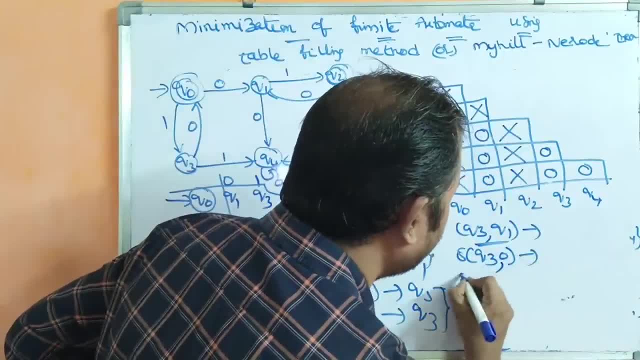 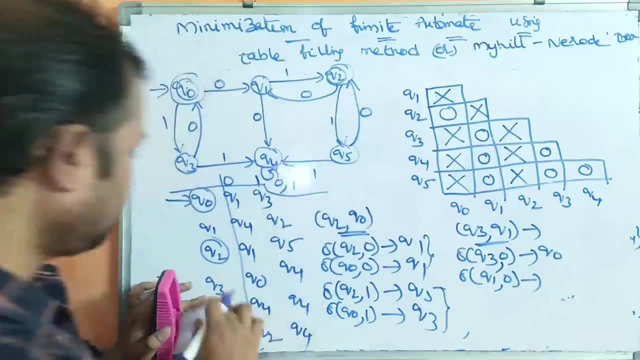 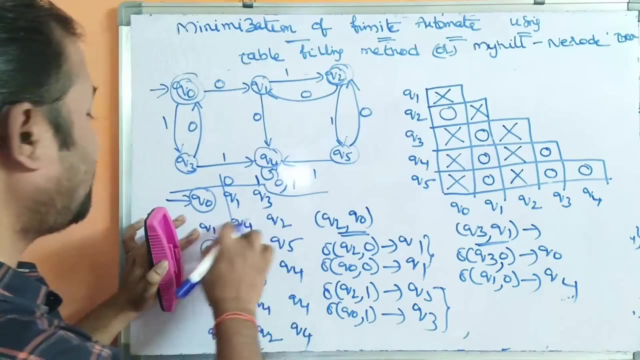 what? Q3- Q1.. So Q3 and 0.. Next one is Q1 on 0.. What is Q3 and 0?? Q3 and 0 means Q0.. Q3 and 0 means Q0.. Next one is Q1 on 0.. Q1 on 0 means Q4.. Q1 on 0 means Q4.. So here we got Q0- Q4.. Q0- Q4. 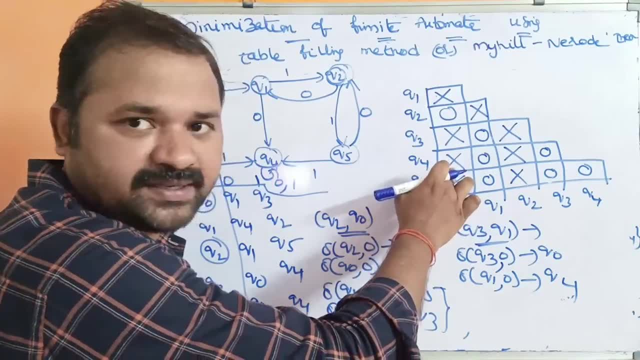 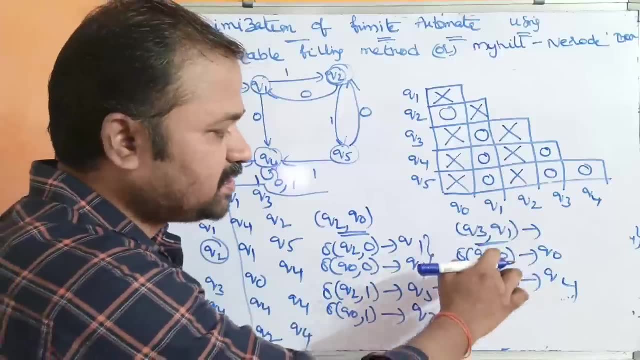 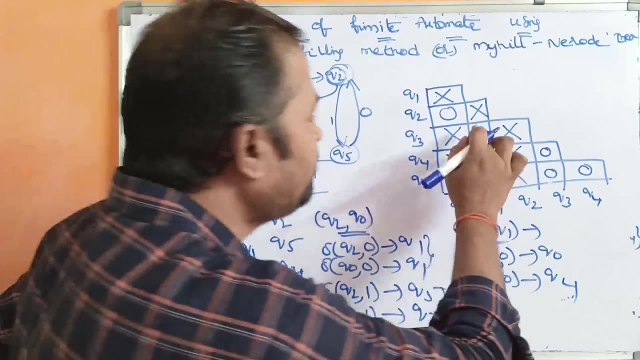 Q0- Q4 pair is already marked. Let us see this one. Q0- Q4 pair is already marked, So we can mark Q3- Q4.. Q0- Q4 is already marked. This is that pair, So we can mark Q3- Q1.. So we can mark Q3- Q1. 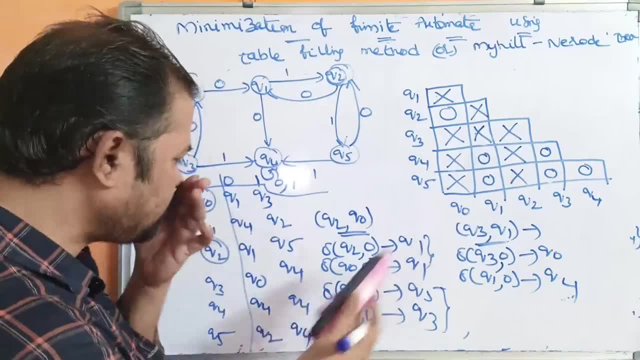 So we can mark Q3- Q1.. So likewise we have to check the remaining pairs. So for space constraints here there is no need to apply one symbol. Why? Because here already the pair is marked. So we can mark Q3- Q1.. So we can mark Q3- Q1.. So likewise we have to check the. 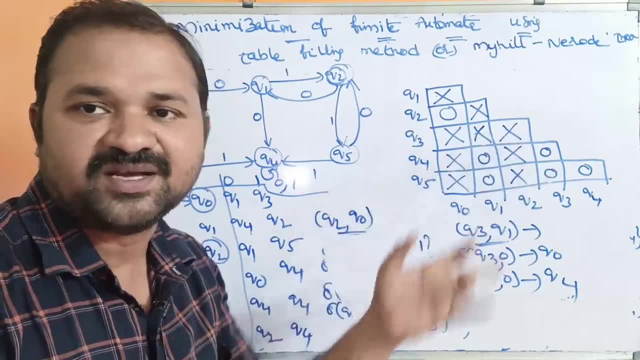 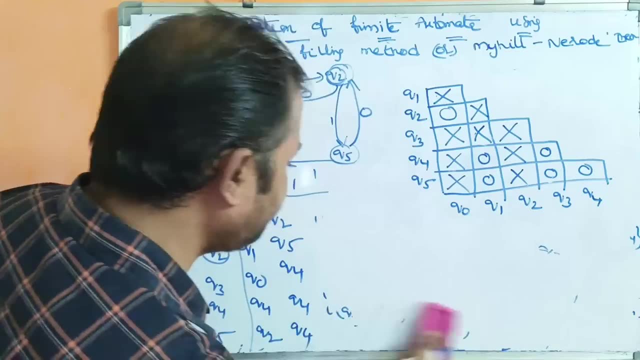 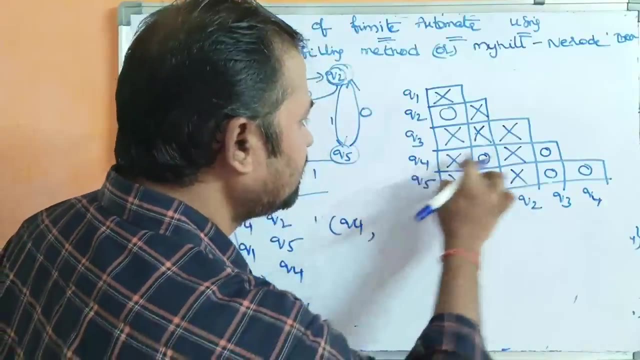 is marked Already. we have marked Q3, Q1 pair, So there is no need to apply one input symbol. So next one is, Next one is So this pair. So this pair is nothing but Q4, Q4 and Q1.. So now we have to. 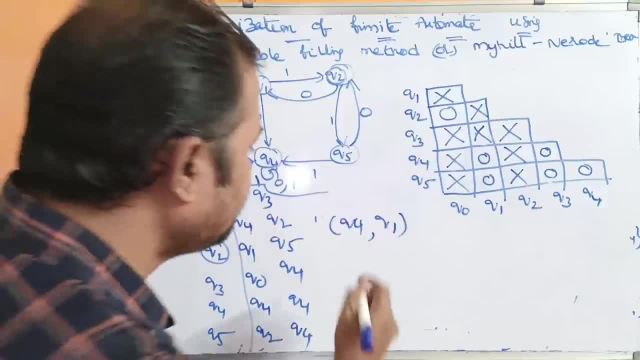 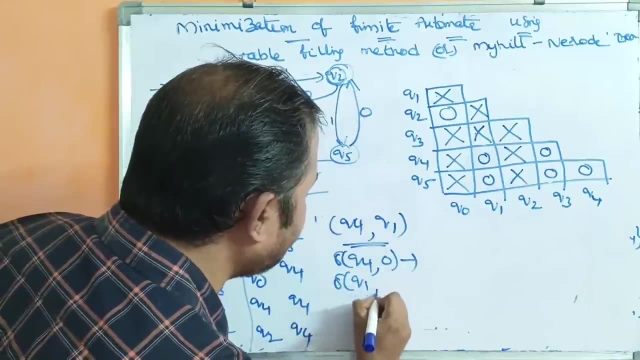 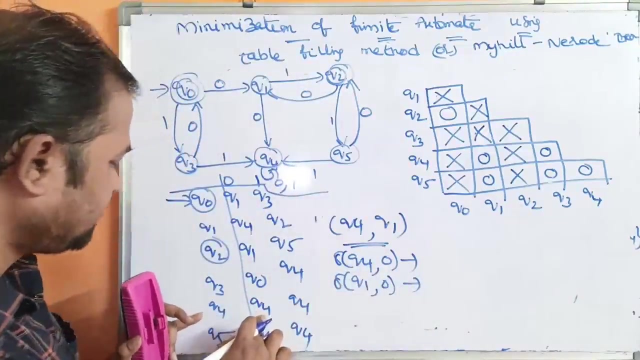 check whether we can mark Q4 and Q1 or not. So for that purpose, simply, we have to apply transitions: 0 on Q4.. Next one is 1 on Q4.. 0 on Q4 and 0 on Q1.. 0 on Q4 means 0 on Q4 means Q4.. Next one is: 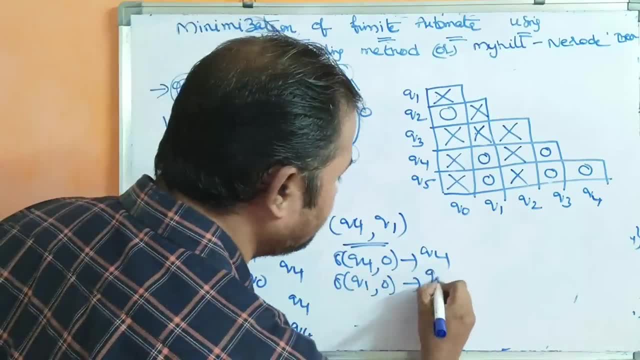 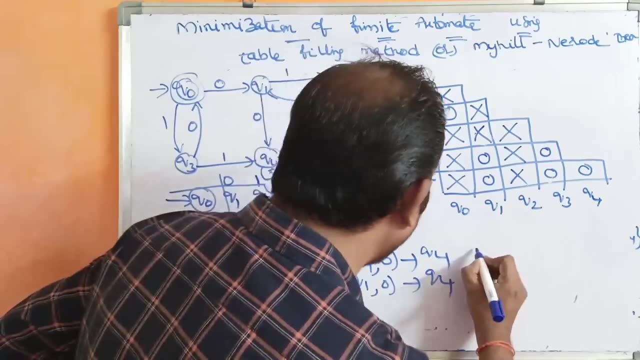 0 on Q1 means 0 on Q1 means Q4. So here we got Q4- Q4. But we don't have any pair like Q4- Q4. So now we have to apply the next one, So apply one input symbol. 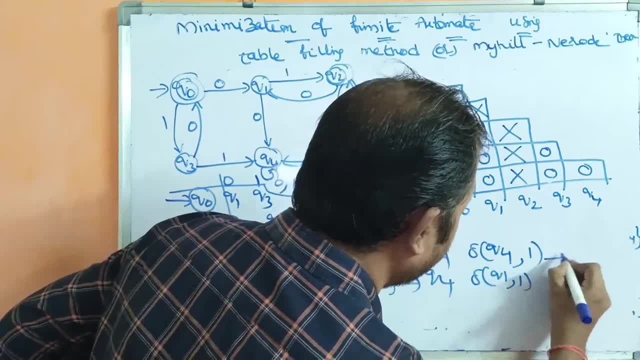 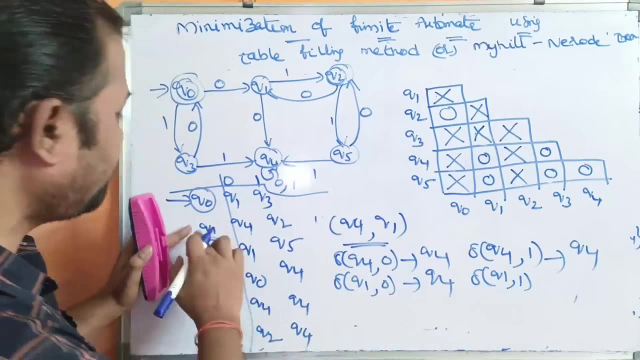 Q4 on 1.. Next one is Q1 on 1.. So Q4 on 1 means Q4.. Q4 on 1 means Q4.. Next, Q1 on 1 means Q2.. Now we have to check whether Q4- Q2 is marked or not. 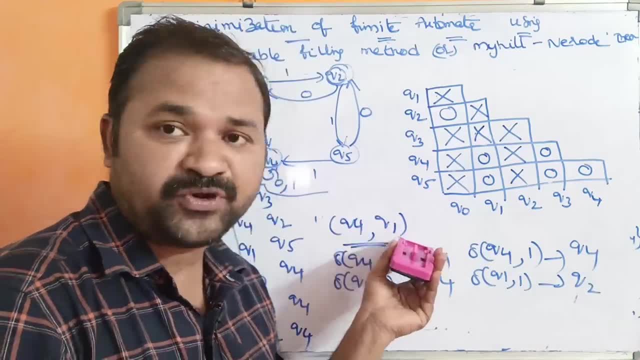 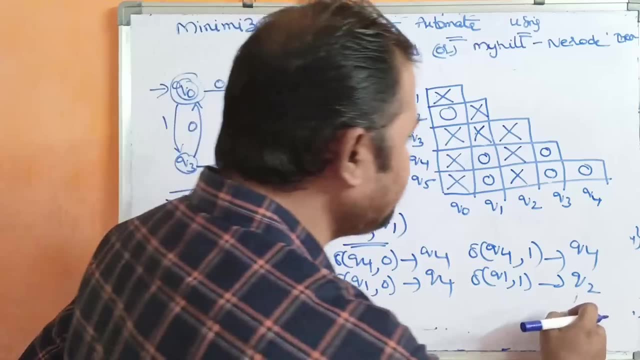 If Q4- Q2 is marked, then we can mark Q4- Q1.. Suppose, if Q4- Q2 is not marked, then it is not possible to mark Q4 and Q1.. Let us check the pair Q2- Q4.. Q2, Q4 or Q4. 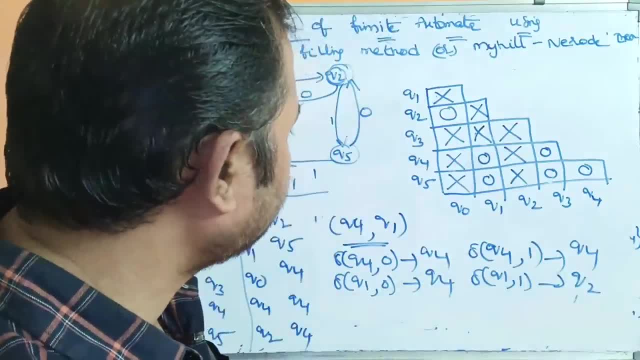 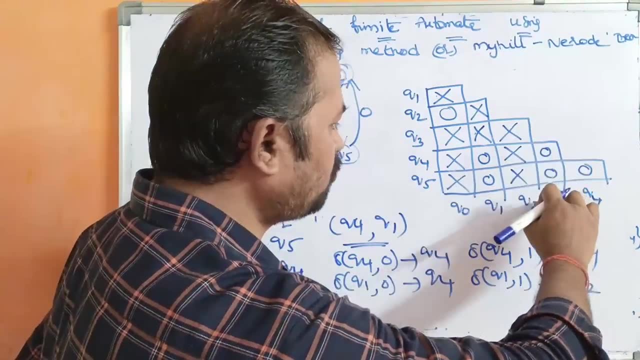 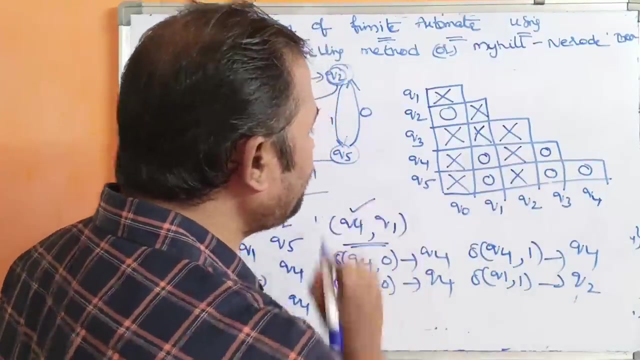 q2. both are same, only q2, q4, q4, q2. so this pair q4, q2, q4 or q4- q2, both are same, only. so this is that pair q2- q4 is already marked, so we can mark q4 and q1. we can mark q4 and q1, so let us mark. 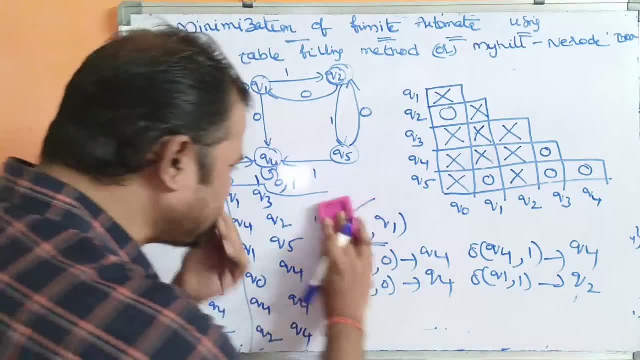 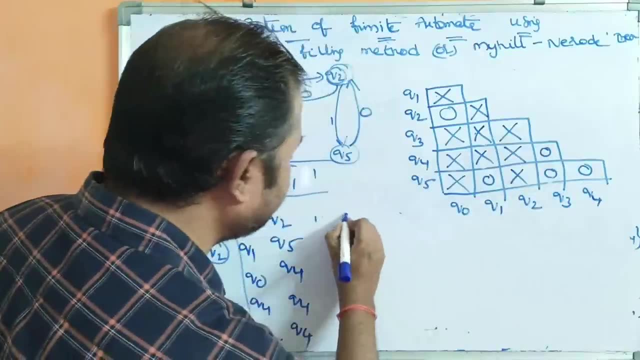 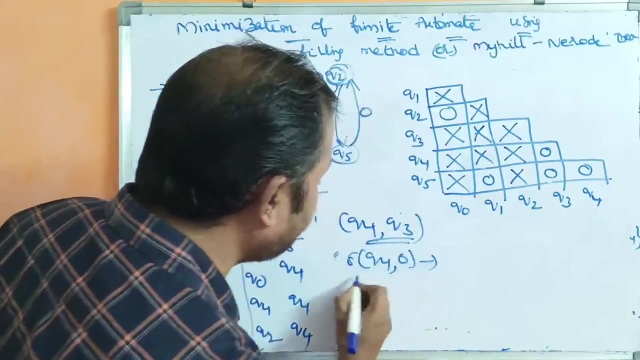 this pair, q4 and q1. now let us check the next pair. what is the next pair? this one, the zero. this zero belongs to what? q4, q3. now let us check whether q4- q3 is marked or not. so, for that purpose, apply the inputs: delta of q4 comma zero. delta of q3 comma zero. what is q4 comma? 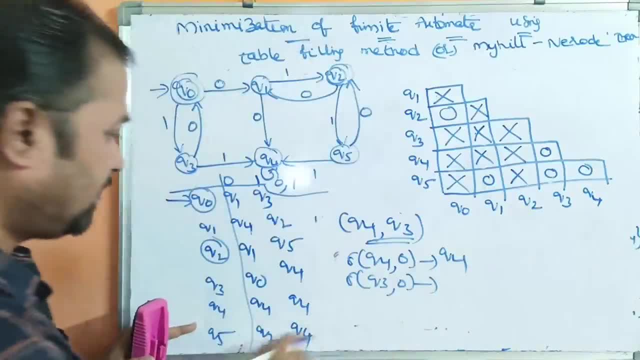 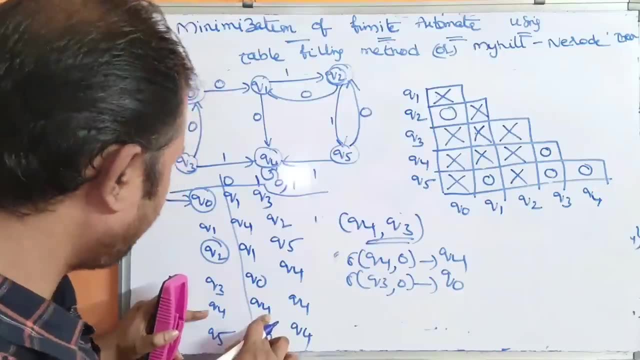 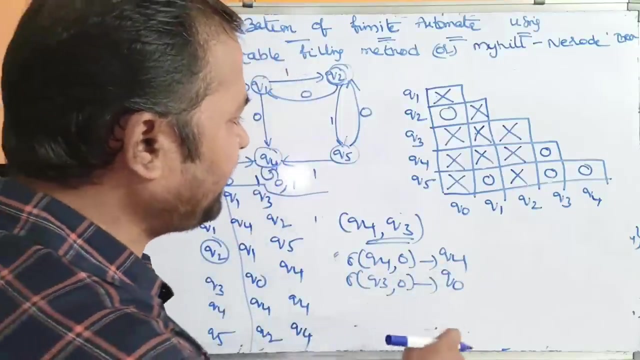 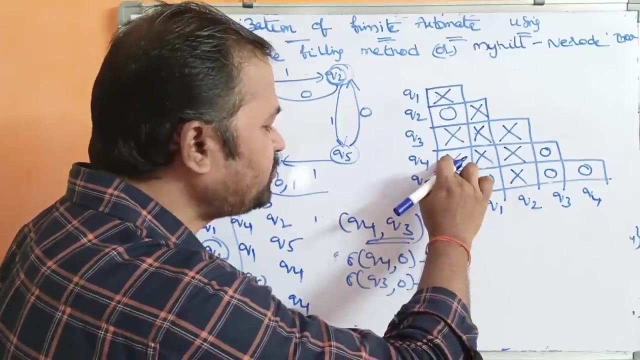 zero. q4 comma zero means q4. next to q3 comma zero means q- naught. q4 comma zero means q4. next one is q3 comma zero means q4- q0. and now let's check about q0- q4 pair, so q4- q0. so this is that pair: q0- q4 or q4- q0, so q4- q0 pair. 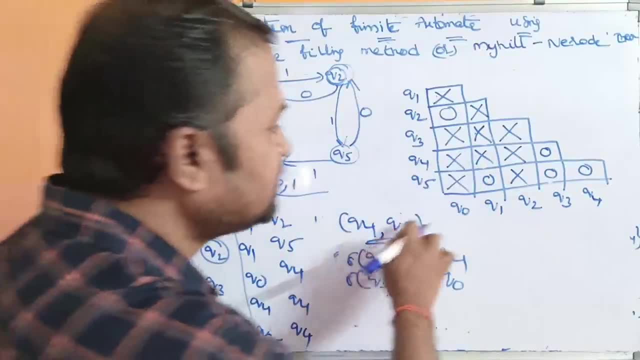 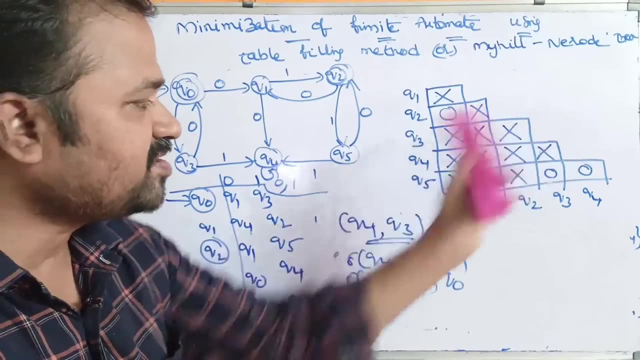 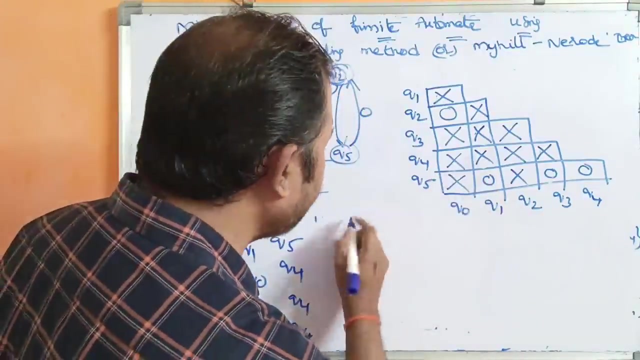 is marked. so we can mark q4- q3. so we can mark q4- q3. so we can mark this pair. now there is no need to apply one symbol. why? because this is already marked. now let us see the next pair. the next pair is q5, q5, q1. 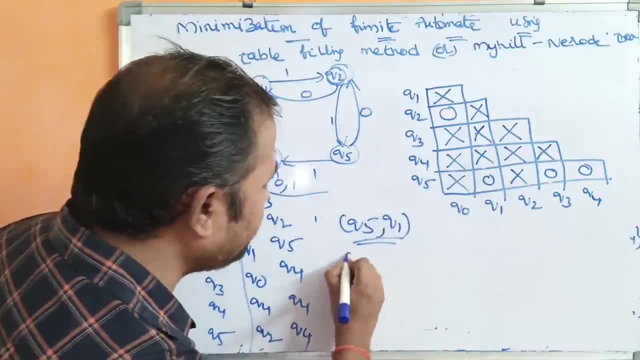 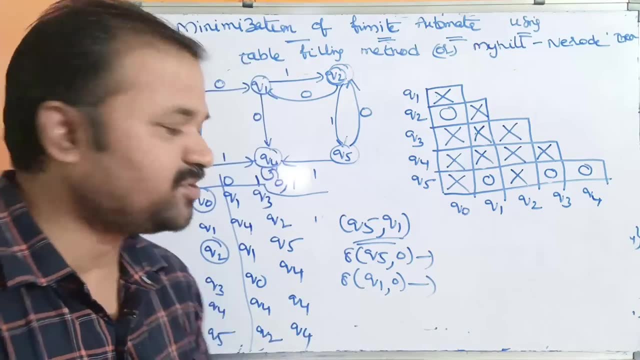 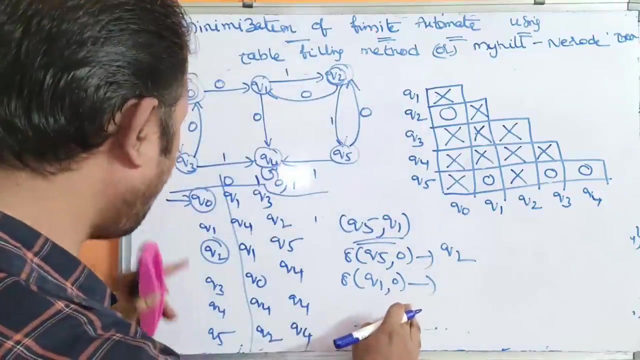 let us check whether we can mark q5, q1 or not. q5, q1. so delta of q5 comma zero. next one is delta of q1 comma zero. so apply zero symbol. so q5 on 0 means q5, on 0 means q2. next, q1 on 0 means q4. 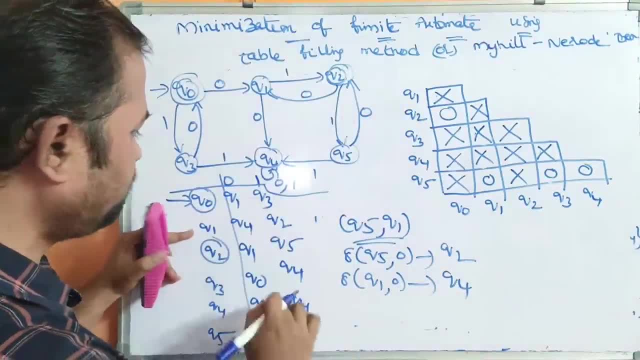 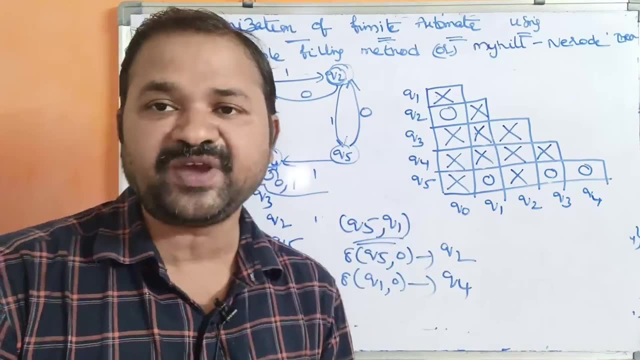 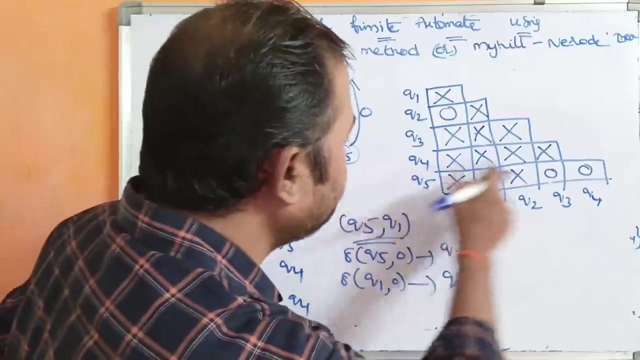 q5 on 0 means q2, q1 on 0 means q4. now let's check whether q2- q4 is marked or not. if q2- q4 is marked, then we can mark q5 and q1. so let's say q2, q4, q2, q4 or q4, q2, q4, q2, q4, q2. so this is that pair: q2- q4. 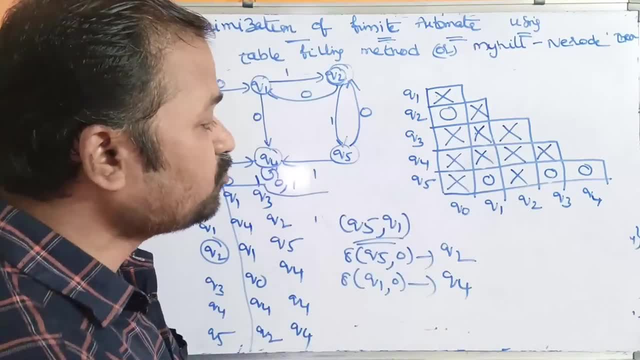 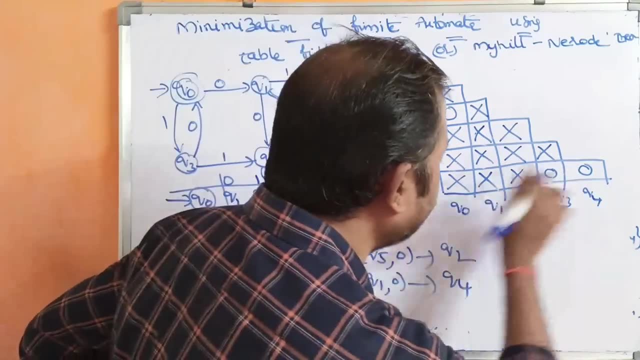 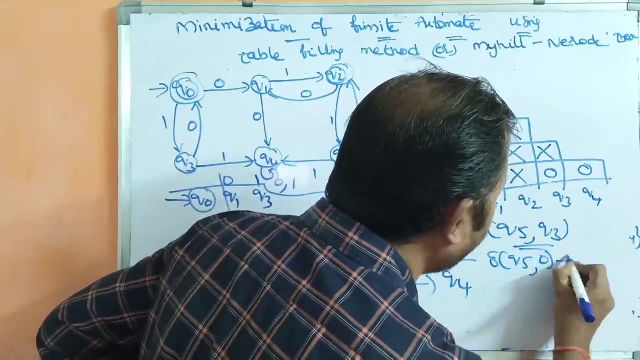 this pair is already marked, so we can mark q5 q1. we can mark q5 q1. now let us check the next pair. what is the next pair? q5 q3, q5 q3, q5- q3. so let us apply zero symbol delta of q5, comma zero. 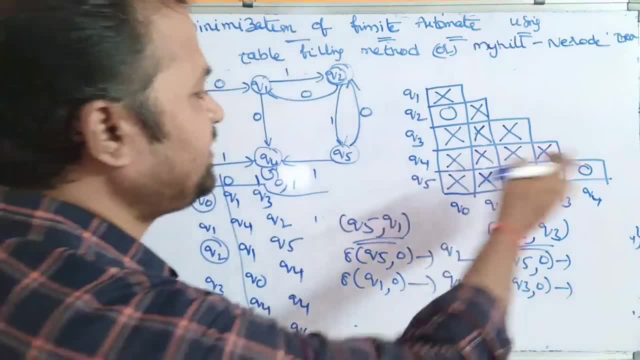 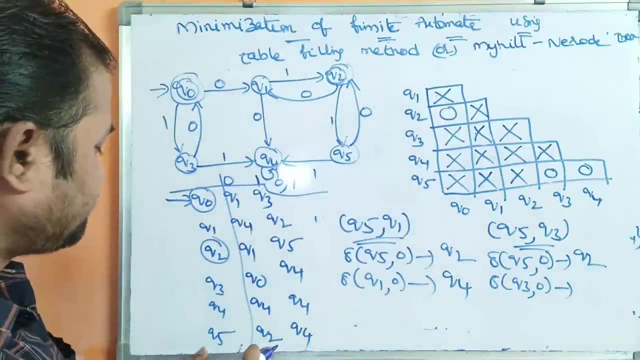 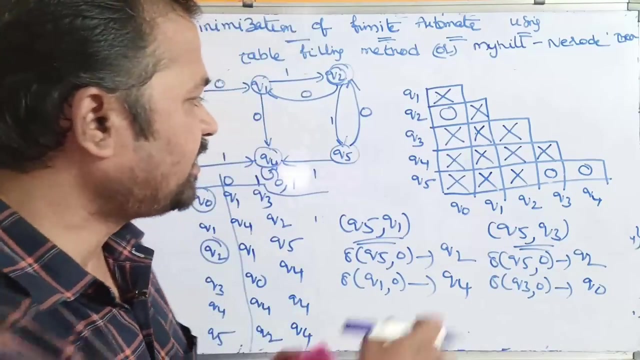 delta of q3 comma zero. so q5, q3, q5 and 0 means q2, q5 and 0 means q2, q3 and 0 means q0, so q0, q2. let's check whether q0, q2 is marked or not. so here we have q, naught, here we have q2. so q, naught, q2 is. 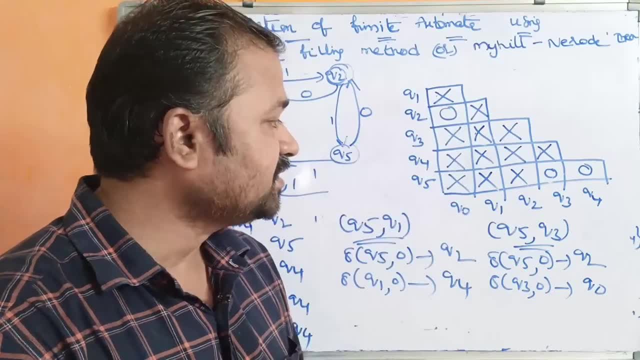 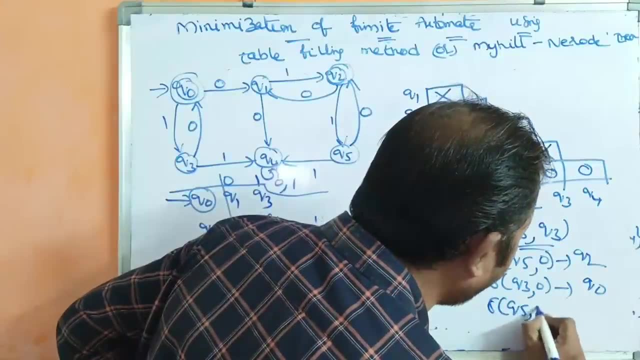 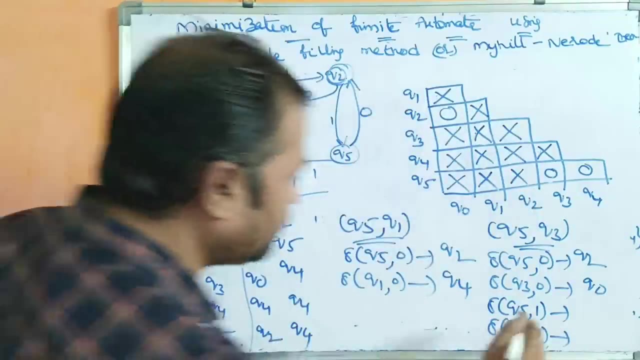 not marked, q naught, q2 is not marked, so it is not possible to mark this pair. so now let us apply one input symbol: delta of q5 comma 1 comma, delta of q3 comma 1. so q5 comma 1 means q4, q5 comma 1 means 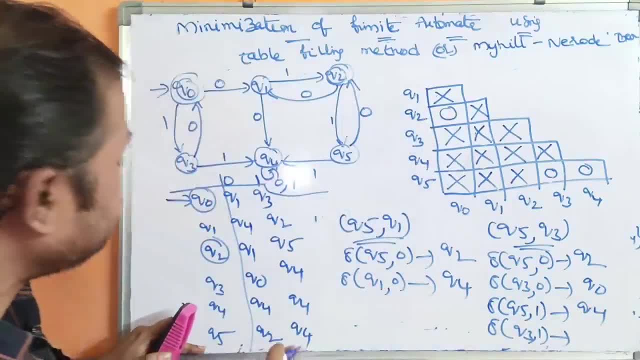 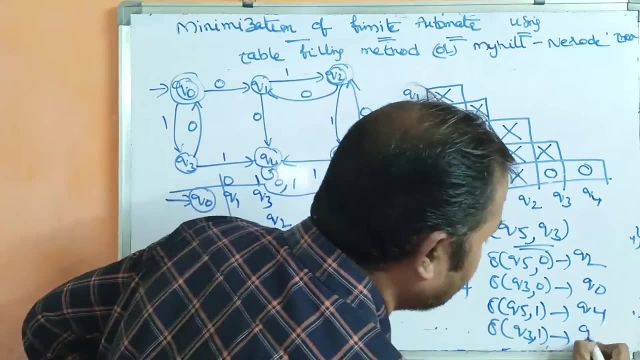 q5. i'm sorry, q5 comma 1 means q4, correct, only next to q3 comma 1. q3 comma 1 means q4- q4. here we got q4- q4, but we don't have a pair like this. we don't have q4- q4. 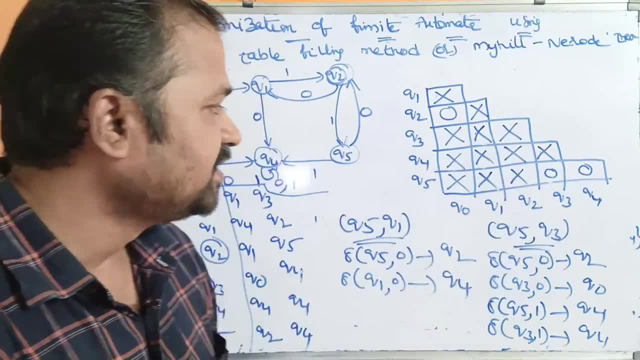 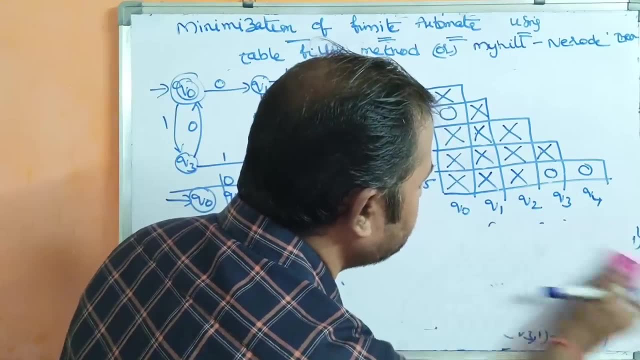 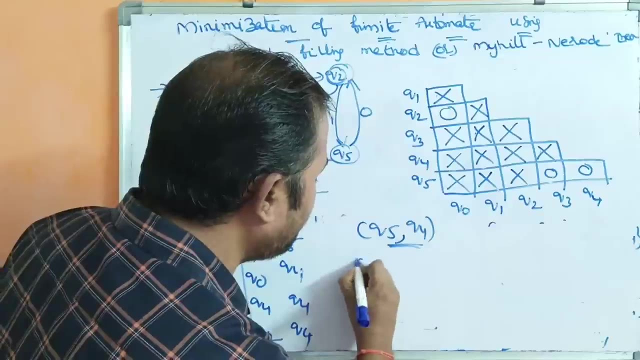 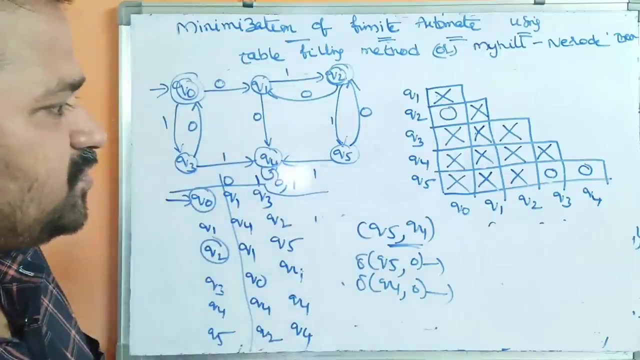 so it is not possible to mark this pair. so marking this pair is not possible. now let us check the next one. let us check the next one. so what is the next one? q5- q4, q5- q4. let us check whether we can mark this pair or not. so q5 comma 0 next to q4 comma 0. q5 comma 0, q4 comma 0, so q5 and 0 means 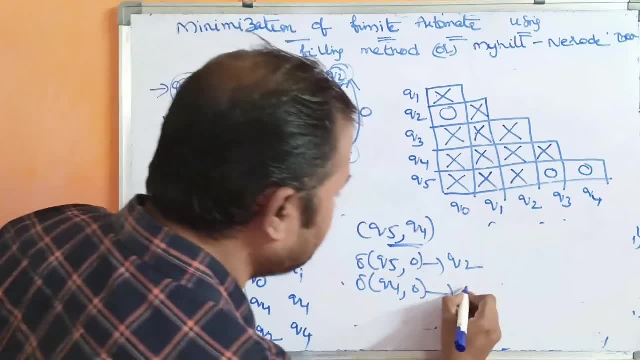 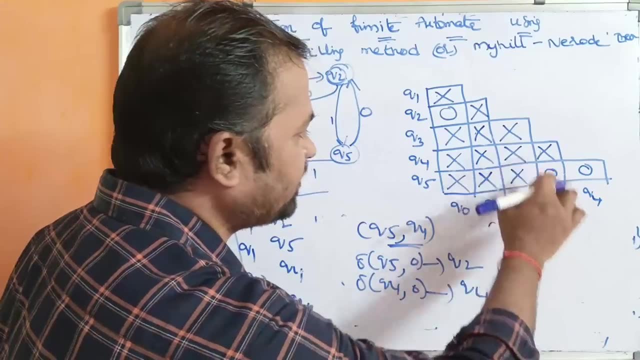 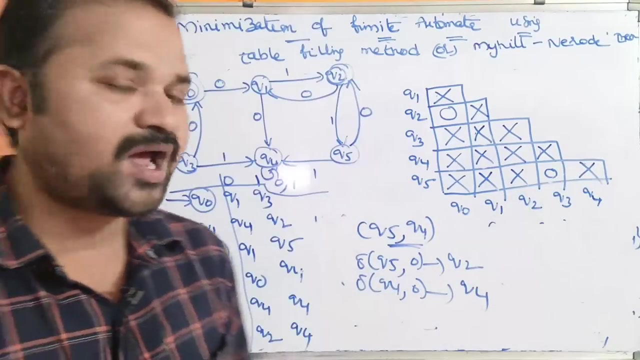 q2- q4 and 0 means q4. let us check whether q4- q2 is marked or not. so q2- q4- this is that pair. q2- q4 is already marked. so we can mark q5- q4. we can mark q5- q4. now we have to do one more iteration. 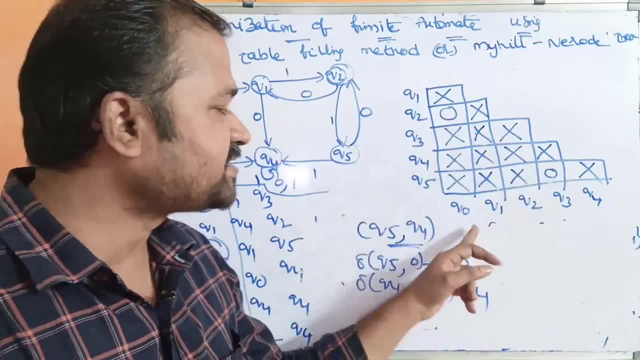 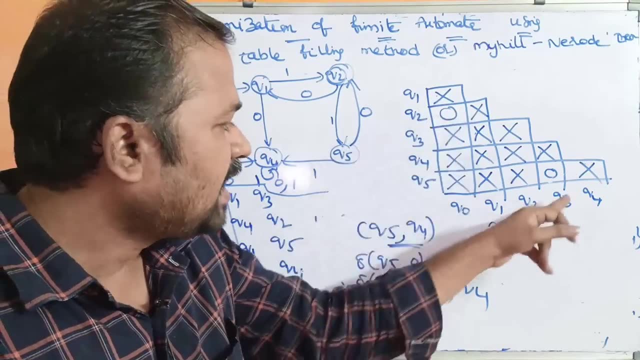 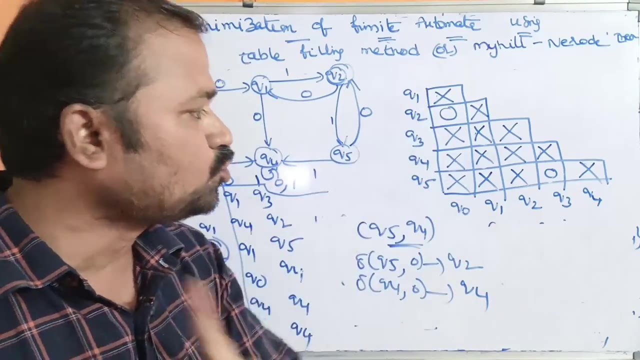 and let's check whether we have two unmarked pairs. are there? let us do the repeat, let us do the process one more time and let's check whether q, naught and q2 and q5 and q3 are marked or not. if they are still unmarked, then we can merge q naught and q2. 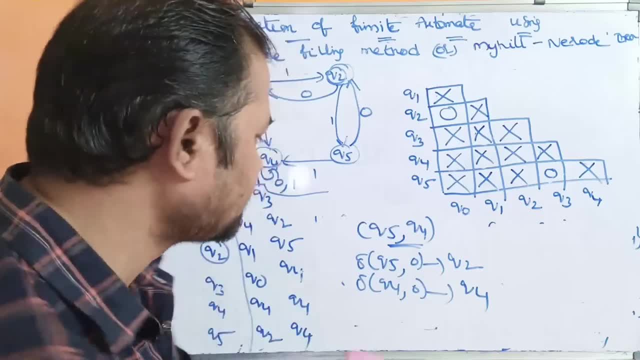 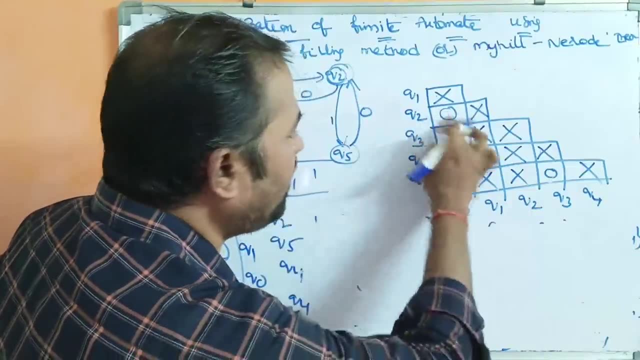 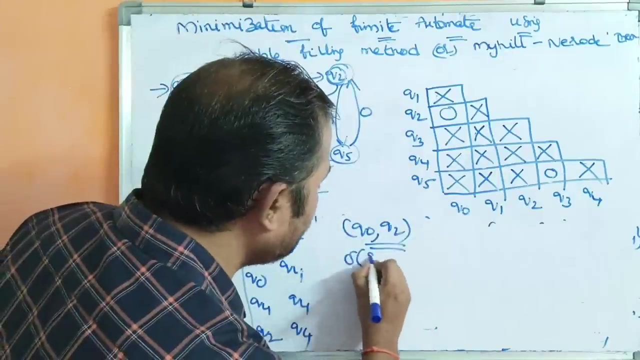 to one state and q3 and q5 to one state. okay, so let us do that process. so what is the pair? q naught q2. let's check here we have two unmarked pairs. are there? let us check whether we can do marking or not. so q naught q2. so q naught on a. next one is q2 on a. so next one is q2 on a, next one is q2 on a. here we have two unmarked pairs are there next, and 작은ian炷sta and q3 and q5 are not. if they are unmarked and q3, then we have q2 and q2 are. 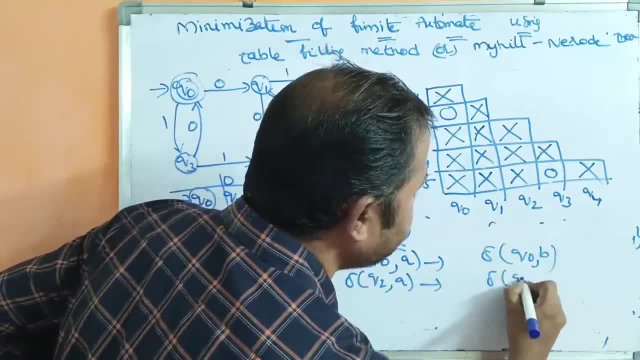 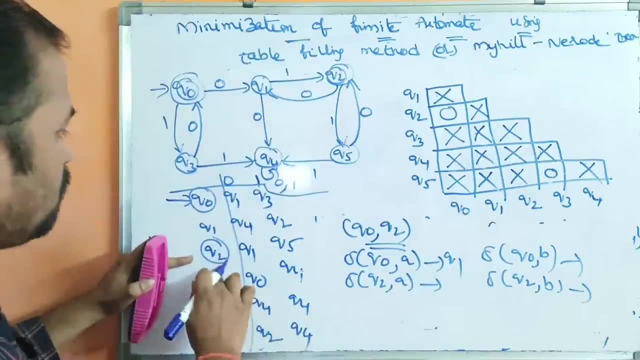 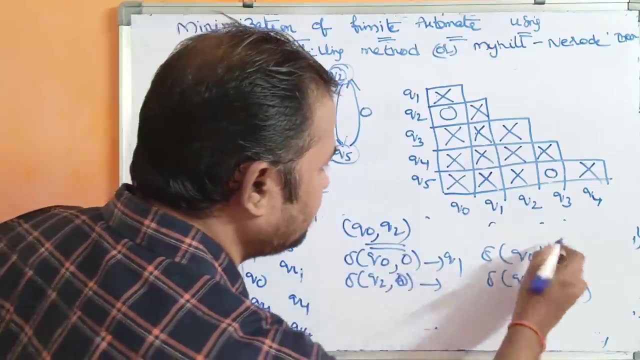 Next Q0 on B. Next one is Q2 on B. What is Q0 on A? Q0 on A means Q1.. Q2 on A means Q0 on. here the inputs are 0.. So this is 0, this is 0, 1, 1.. 1, 1.. 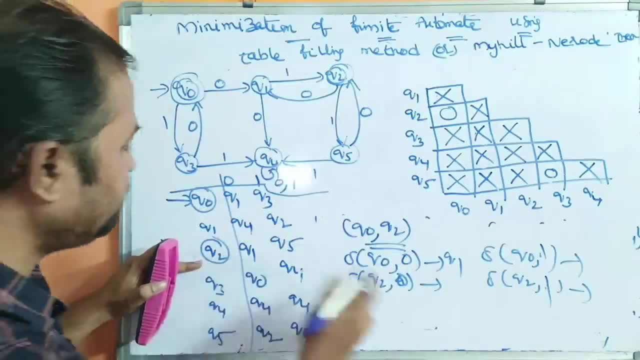 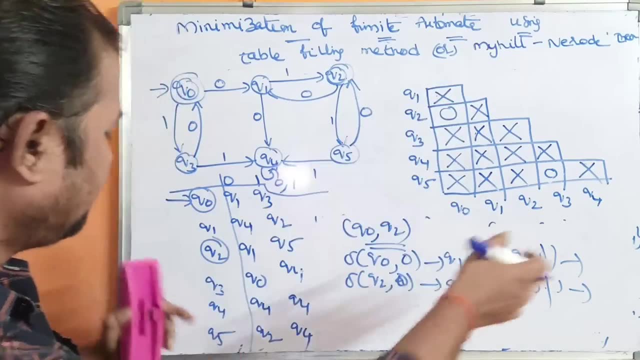 So Q0 on 0 means Q1.. Q2 on 0 means Q1.. We don't have any pair like Q1, Q1. So marking that pair is not possible. Let us apply one: Q0 on 1 means Q3.. Next, Q2 on 1 means Q5. 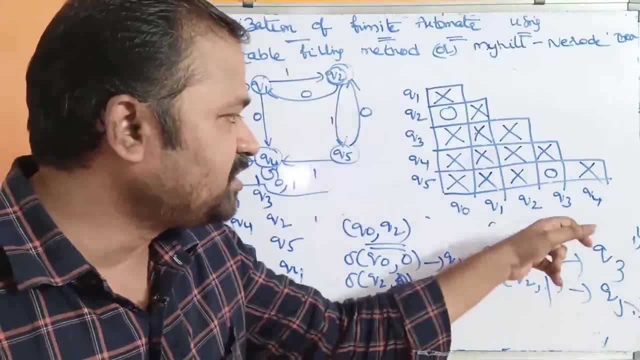 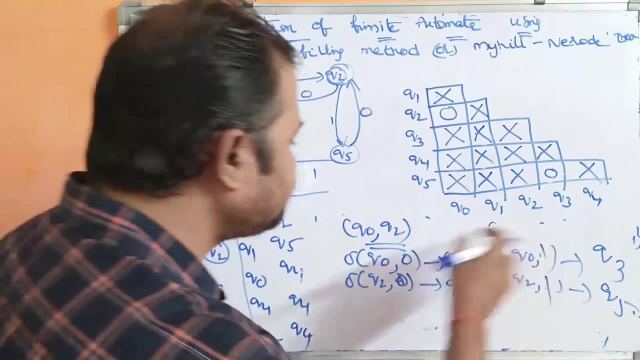 Now let's check whether Q3, Q5 is marked or not. So Q3, Q5 means this pair. This pair is not marked, So marking Q0 and Q2 is not possible. Likewise check Q3, Q5.. Q3, Q5. 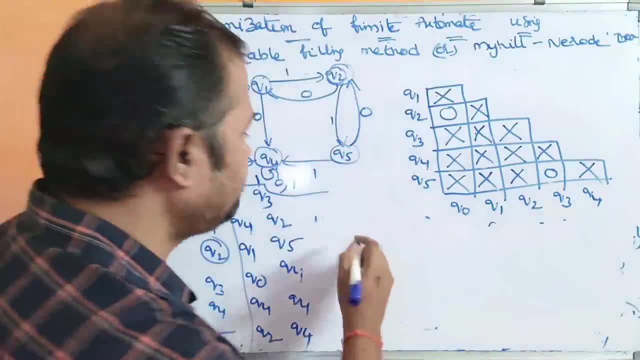 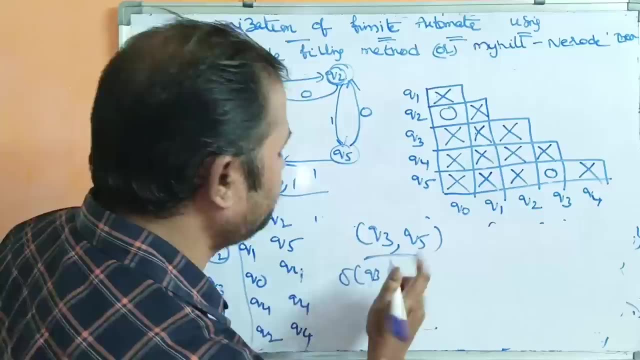 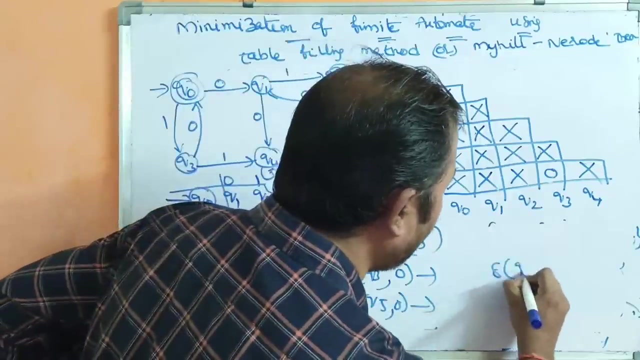 Likewise check Q3, Q5.. So delta of Q3, Q5.. So apply the symbols Q3, Q5.. So delta of Q3, 0.. Delta of Q5, 0.. So next one: delta of Q3, 1.. Delta of Q5, 1.. 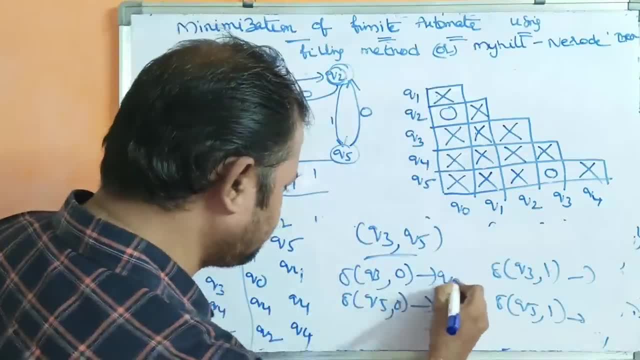 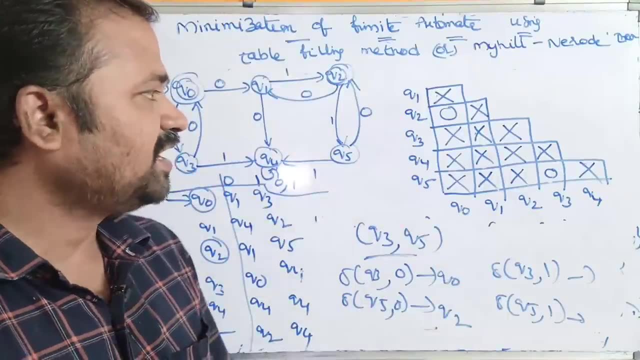 So Q3 on 0 means Q0.. Q5 on 0 means Q2.. Q5 on 0. q2. so here we got q naught q2. let's check whether q naught q2 is marked or not. q naught q2, this pair. 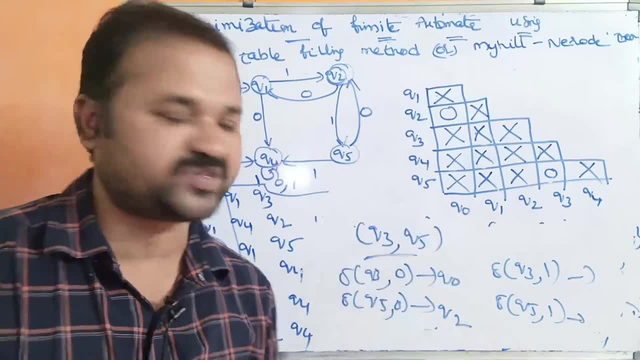 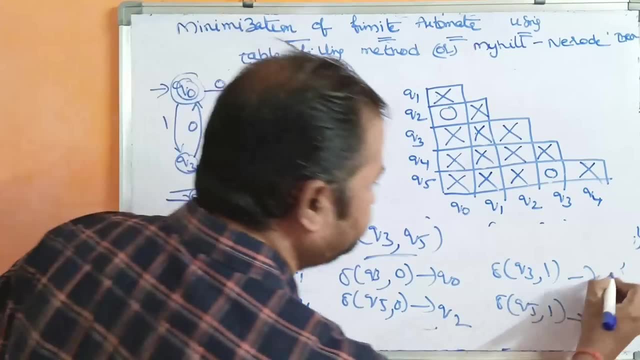 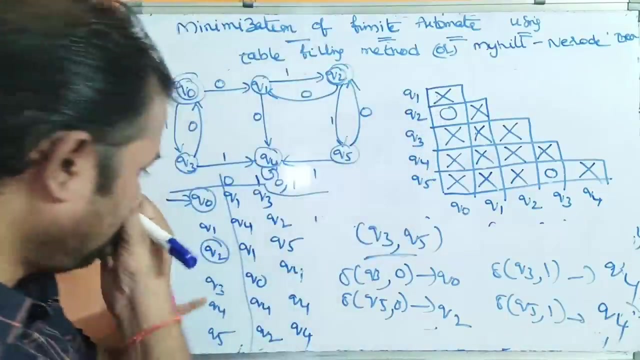 this pair is not marked, so marking this pair is not possible. next: q3 and 1. q3 and 1 means q3 and 1 means q4, q3 and 1 means q4, q5 and 1 means q4, so q3, q5, q3 and 1 means q4, q5 and 1. 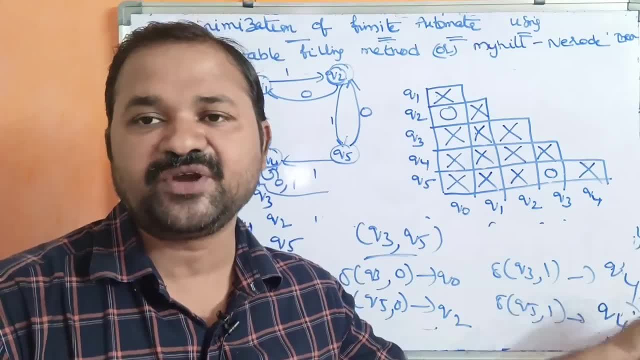 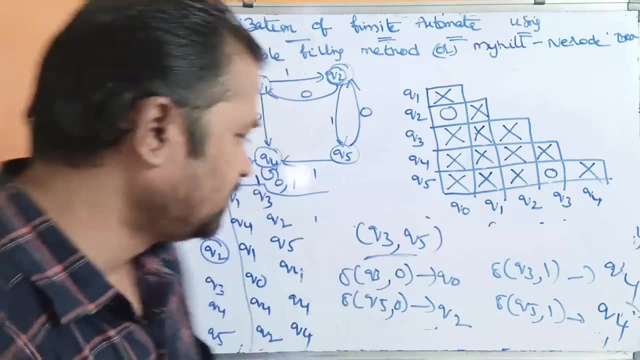 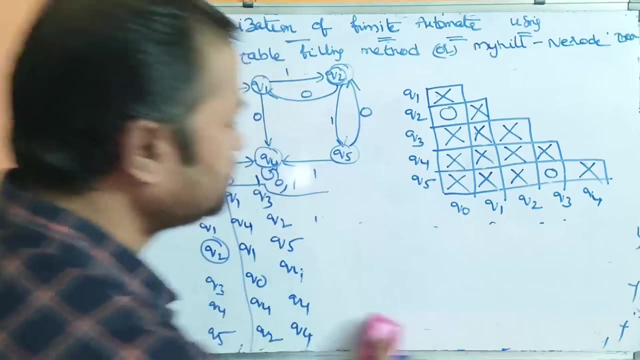 means q4. we don't have q4, q4. we don't have the box q4, q4. so here with this, we can conclude that these two pairs are not marked. so now we can merge these two into one states. we can merge those two into one states. so now the states are. we can merge q, naught and q2. why? because marking. 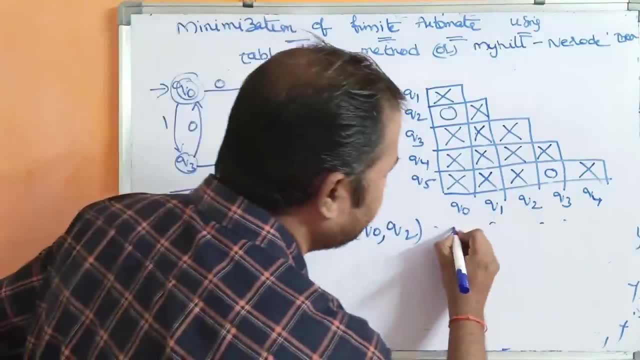 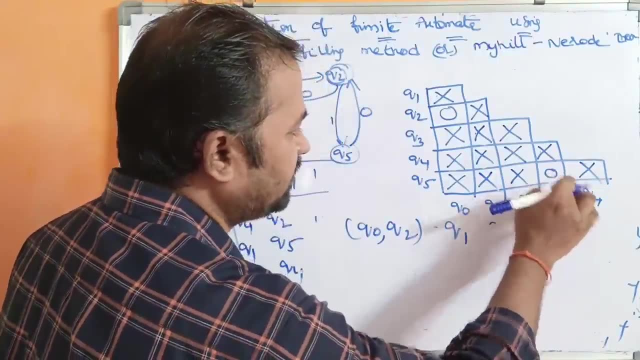 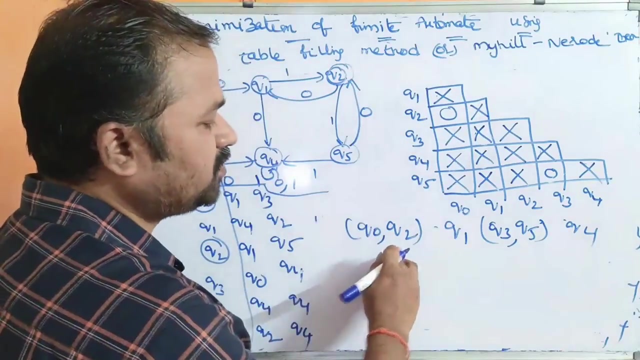 this pair is not possible. q naught and q2 is one state, next state is q1, next state is q1. next here we can merge q3 and q5. we can merge q3 and q5, so next state is q4. so q0, q2, q1, q3, q5, q4. 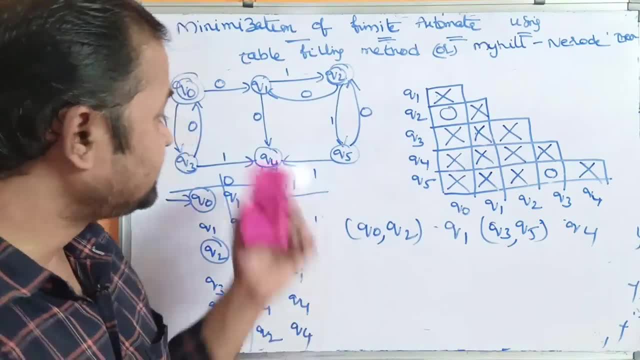 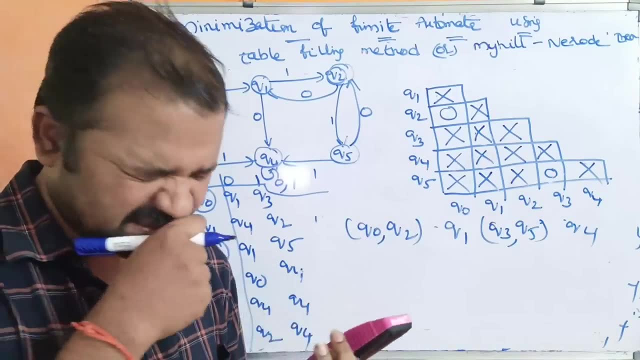 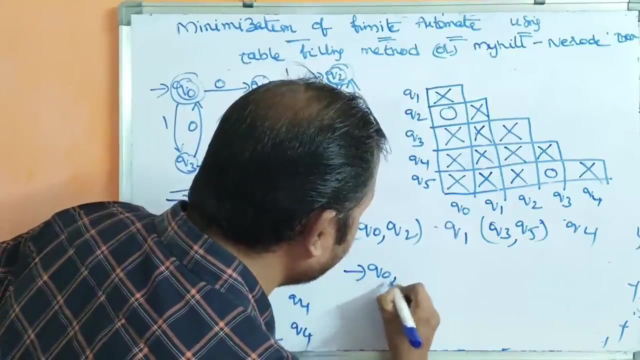 initially, the finite automata contains 60 states, six states. now those six states are reduced to one, two, three, four, four states. now let us construct the. now let us construct the finite automata, let us construct the nfa. so the first state is q0 comma q2, q0 comma q2. so next state is q1.